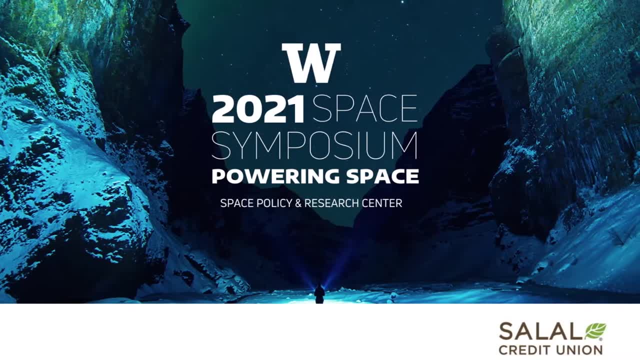 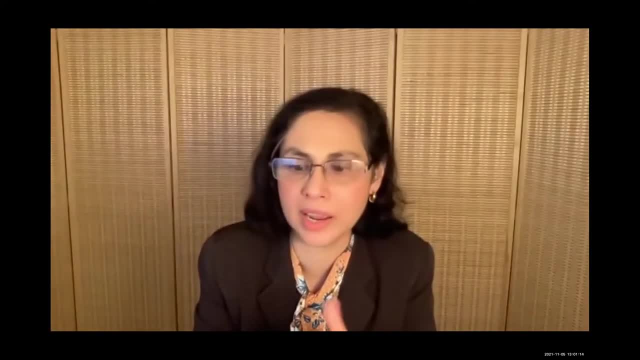 All right, Thank you very much. Welcome back, everyone. What a great morning. We hope you're enjoying being here with us today. We're pleased to present this next panel, which is about Power for Propulsion, And I have the pleasure of introducing our moderator, a colleague. 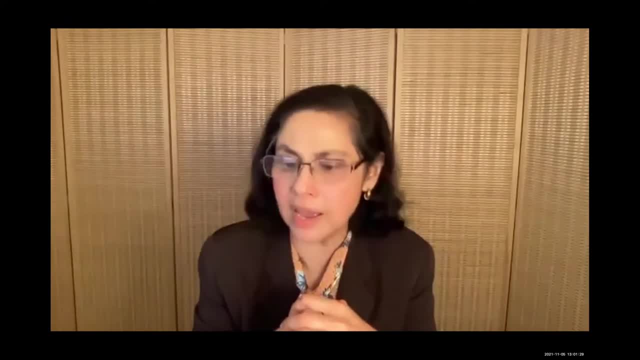 of ours here at the University of Washington, Yuri Shumlat Yuri is a professor in aeronautics and astronautics. He has won numerous awards for his teaching, research and mentoring. He's a fellow of the American Physical Society, an associate fellow of the American Institute. 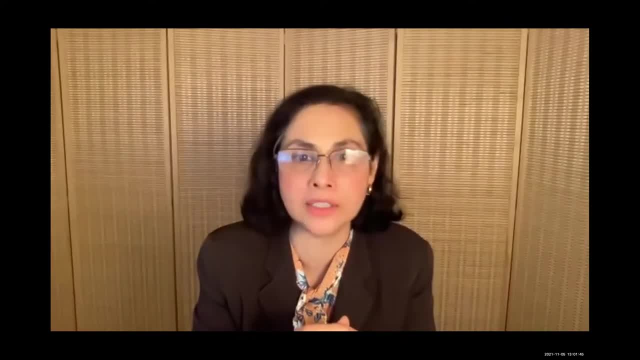 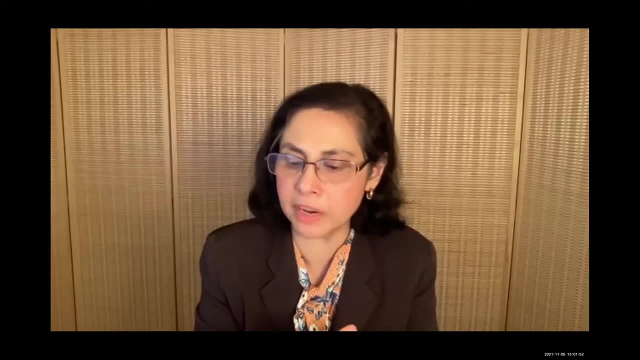 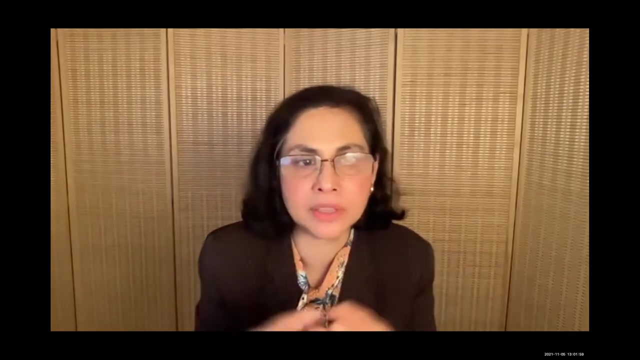 of Aeronautics and Astronautics and a senior member of the Institute of Electrical and Electronics Engineers. He has also co-founded Zapp Energy, a spin-up company from the UW to develop commercial fusion applications, And I believe that, after the panel is done, 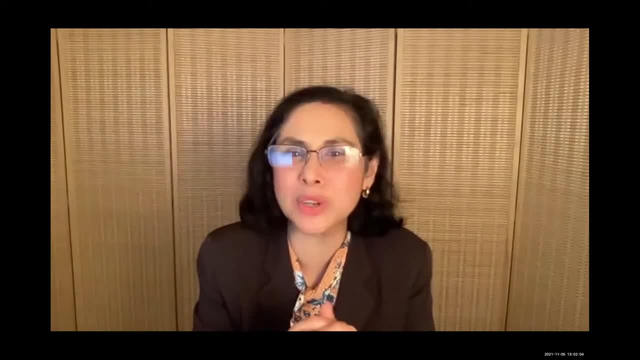 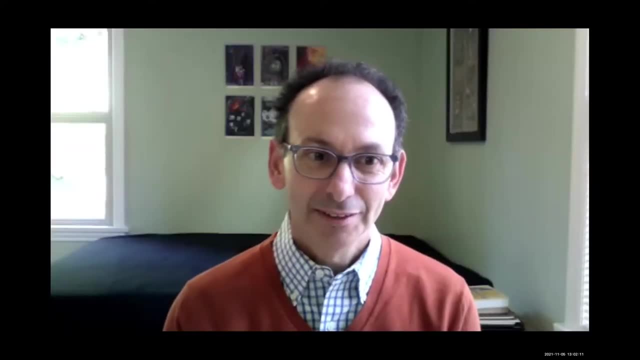 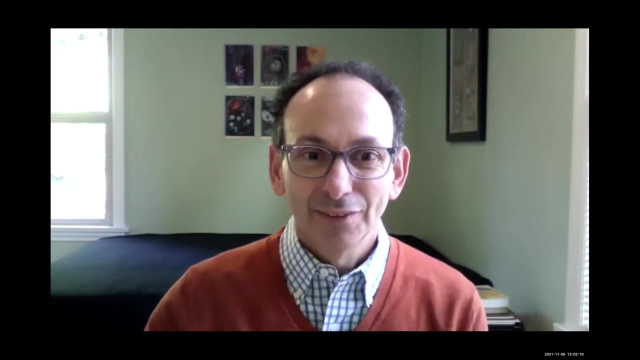 Amy Sprague will be moderating the Q&A. So, Yuri, I'm going to hand things over to you. Thank you very much for your role today. Great Thank you, Saadi. Thank you for the kind introduction. So I think perhaps, if I just add one thing, I'm also a child of the. 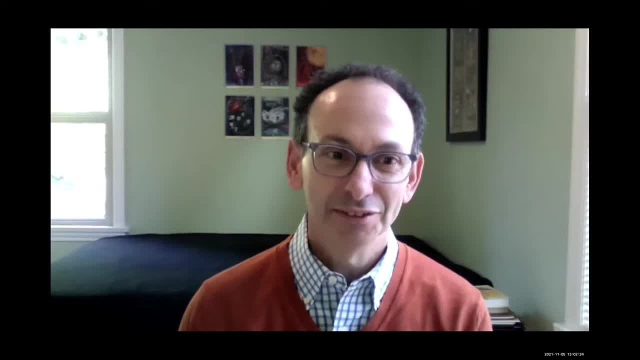 Apollo-Soyuz and the oil embargoes of the 70s, both of which strongly influenced and shaped my scientific and societal objectives for my career. So I'm very happy to be here And I'm very excited to be here, And I'm very excited to be here And I'm very excited to be here And I'm 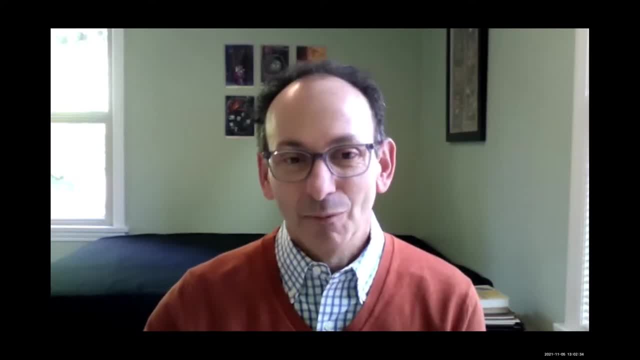 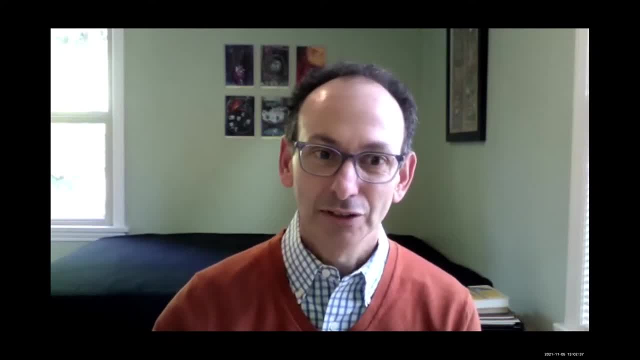 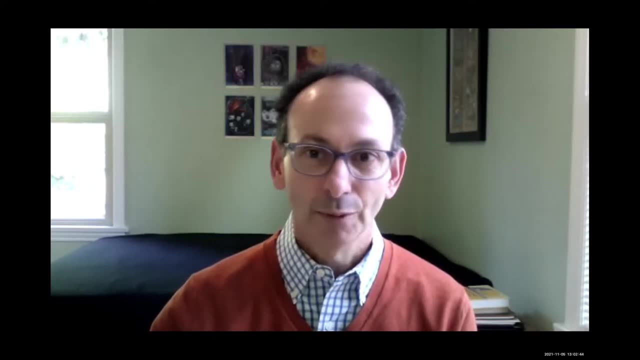 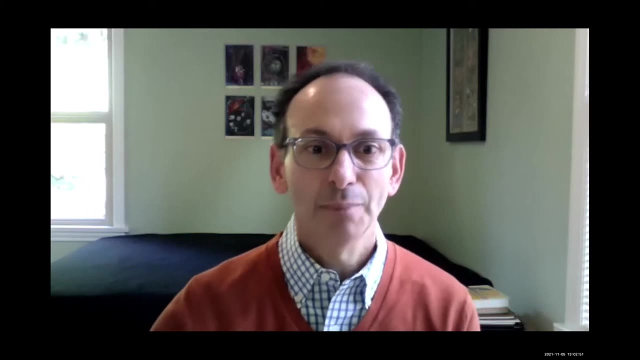 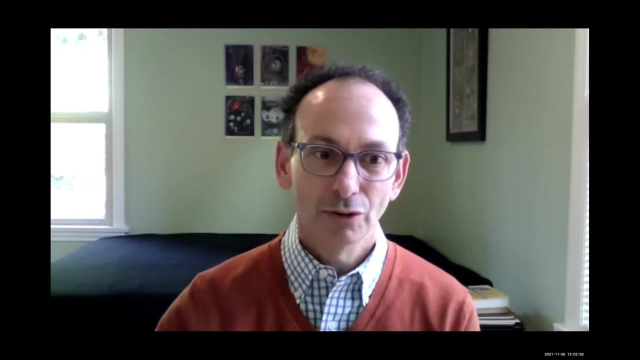 passions and interests center around plasma technologies, particular fusion energy for terrestrial and space applications, in particular, rapid deep space exploration. So I'm really delighted to be here, to be moderating this panel today on power for space propulsion. Our panelists provide an interesting cross-section of the field. 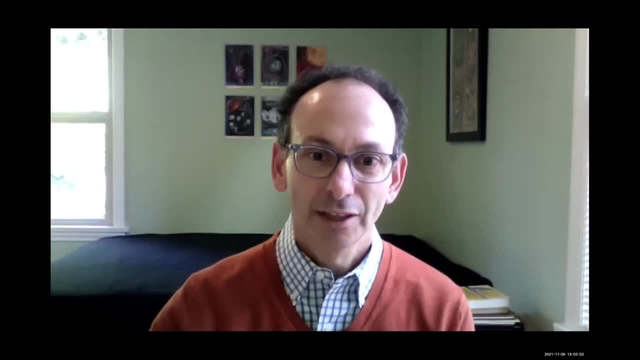 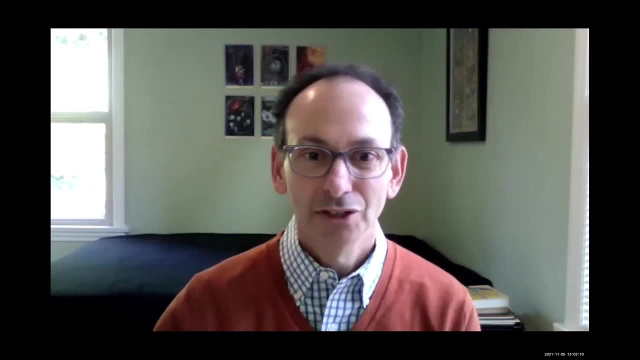 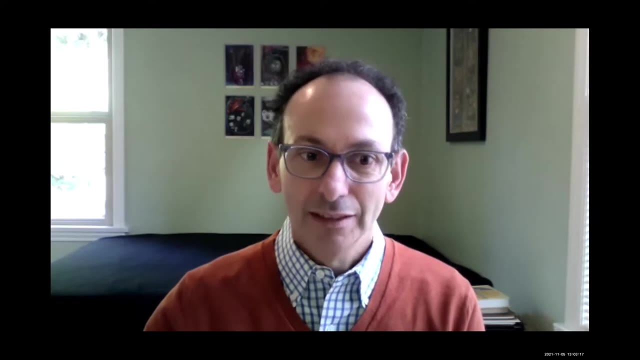 each bringing an expertise that's highly relevant to the facet of space power. I so look forward to what will be a fascinating and informative conversation, And so now I'd like to begin by introducing our panelists, And so, to begin, I'll introduce Roger Myers. 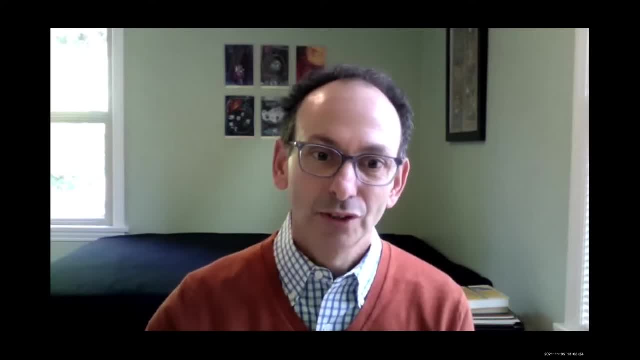 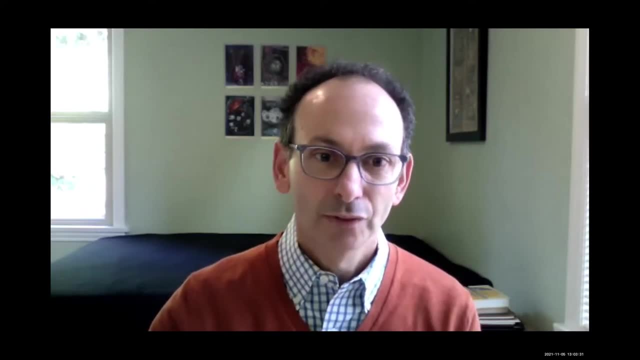 He's chair of the Joint Center for Aerospace Technology and Innovation, CHICOTI. He's a long-time leader in aerospace, served in several scientific and executive roles in Aerojet Rocketdyne. He's served on committees for the National Academies, including recently the Space Nuclear Propulsion for Human Mars Exploration. 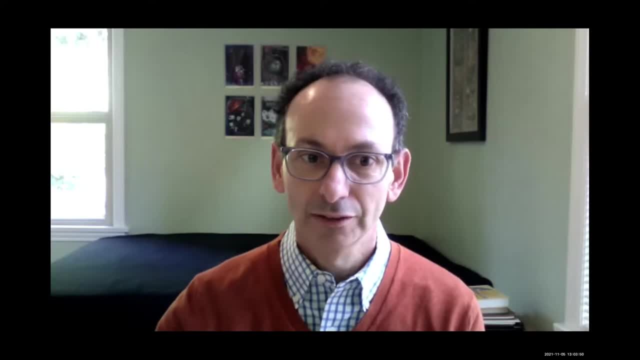 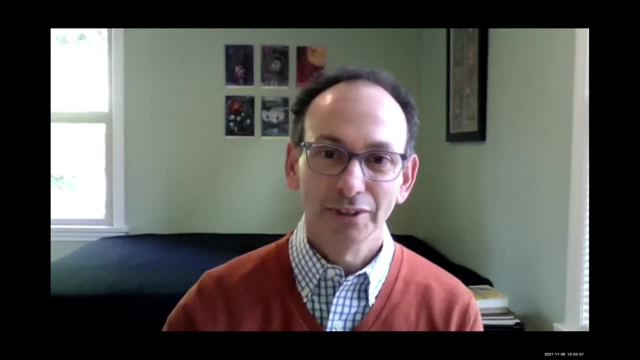 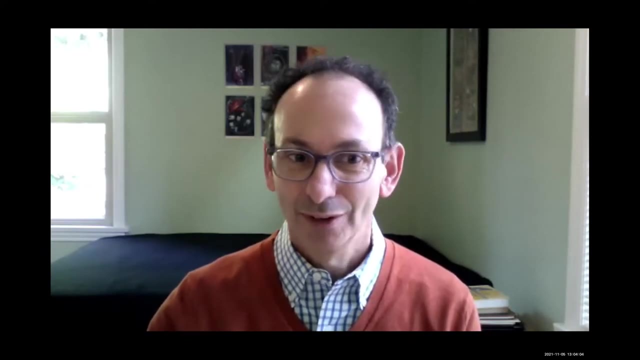 He's a fellow of American Institute of Aeronautics and Astronautics. He's a long-time friend and colleague and a trusted expert on any and all space-related technologies. And after this, Roger will be giving us a brief tutorial. so, Roger, would you like to say hello? 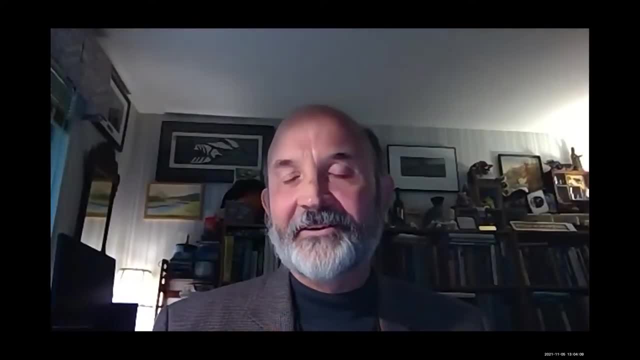 Roger Myers. Hello everybody, It's an honor to be asked to do this and I hope that my tutorial is good. And Yuri, are you going to do we? should I start now or are you going to introduce everybody first? 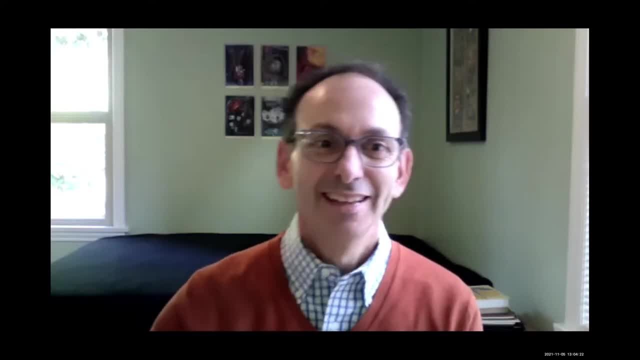 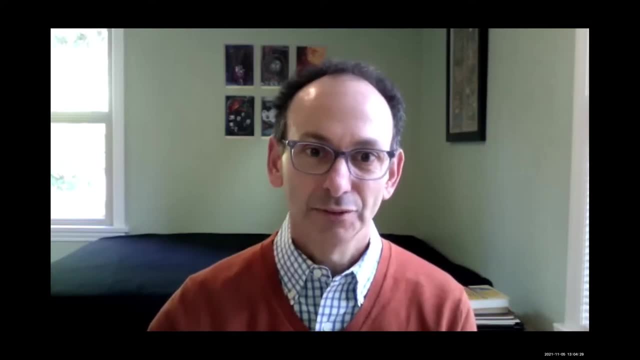 I'm going to introduce all the panelists. first, Roger Myers. Perfect, perfect, Roger Myers. And so next, it's my pleasure to introduce Jess Rogers. She's a legislative and regulatory analyst at Pacific Northwest National Laboratory. She's an international lawyer specializing in arms control and nonproliferation. 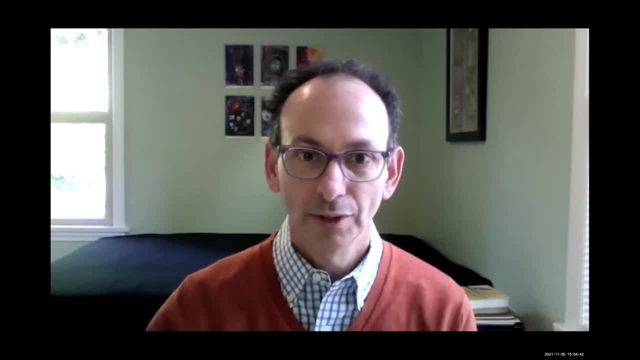 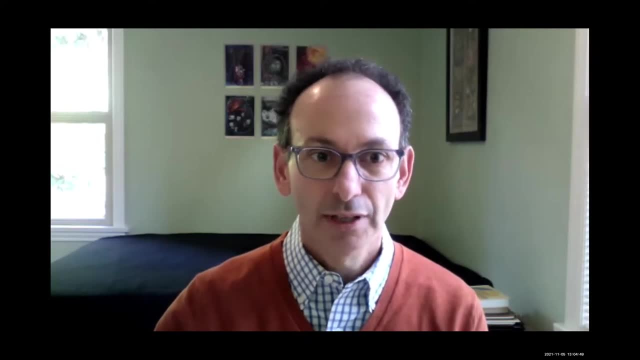 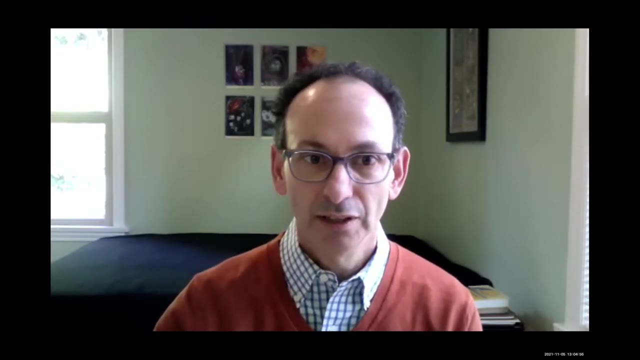 She's promoted nuclear arms control policy at the Nuclear Threat Initiative. helped implement treaty obligations at the US Department of State Bureau of International Security and Nonproliferation. serves as an expert for the US Department of Energy, US Department of Defense, US Department of State. 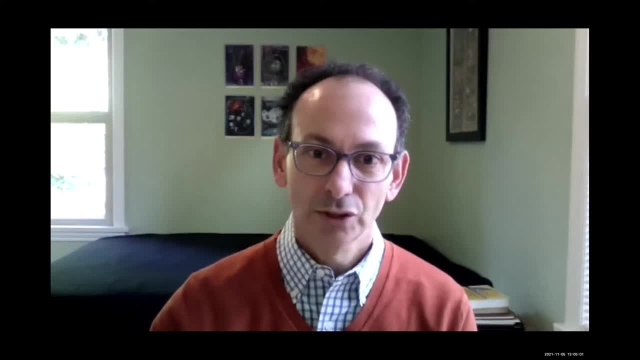 And she will add what I'm sure is going to be a vital perspective that contextualizes many of the opportunities and challenges for space power, Particularly the power needed for deep space exploration, the high power needed for deep space exploration. Roger Myers, Jess, would you like to say hello? 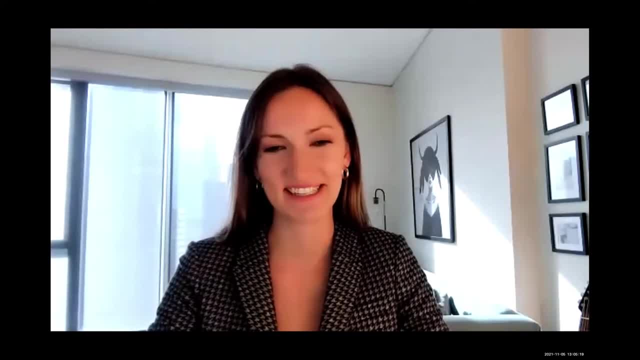 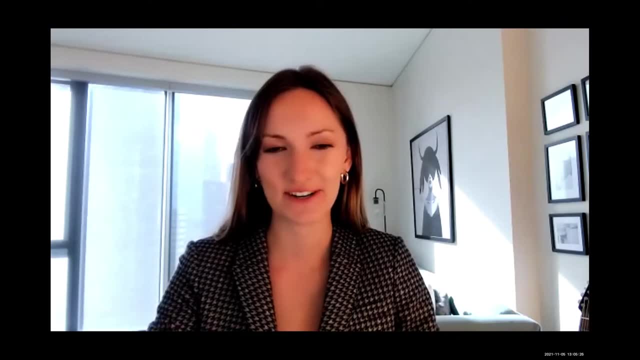 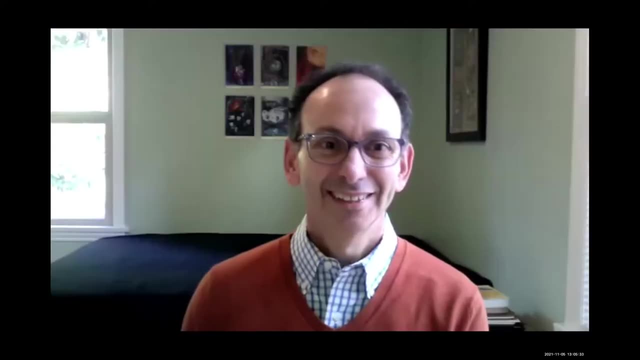 Jess Rogers. Yeah, thank you, Yuri. Hello everyone, Very delighted to be on this panel, particularly because this year PNNL and SPARC have just entered into a new partnership. So very, Roger Myers, Okay, very much looking forward to this cooperation. great, thank you, jess. um, and so next i'd like. 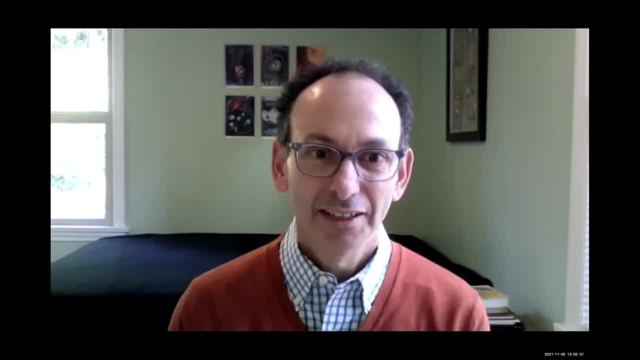 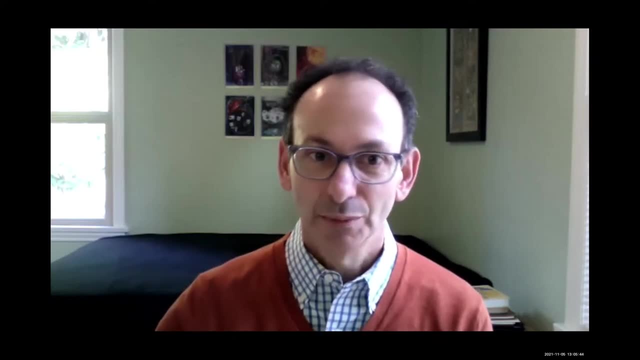 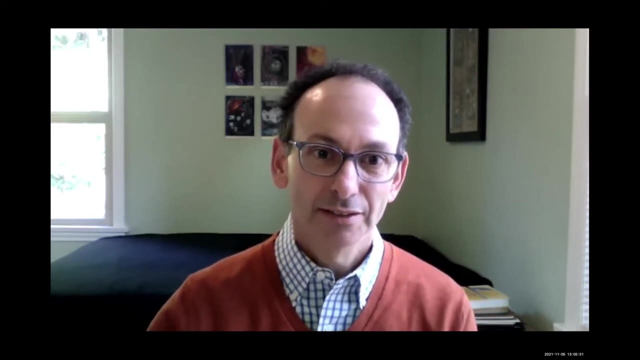 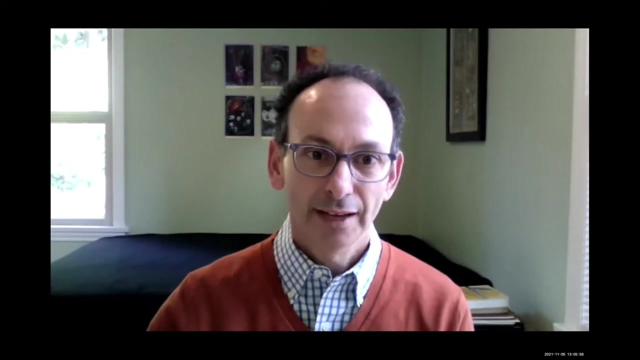 to introduce jeff katalinich, who's a research scientist. research scientist at pacific northwest national laboratory. he previously was a project manager at an afrl sponsored university satellite project. in his phd he specialized in nuclear engineering and applied aerospace engineering, material science and chemistry. he received the national science foundation graduate fellowship. 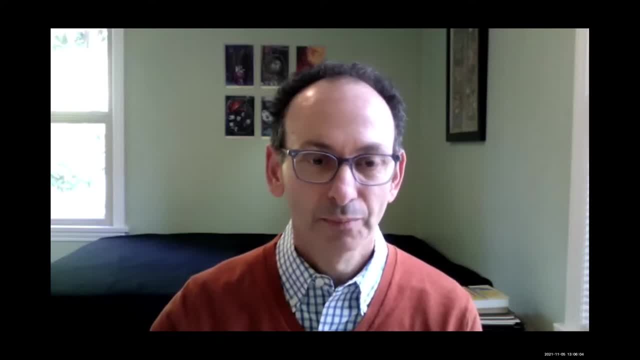 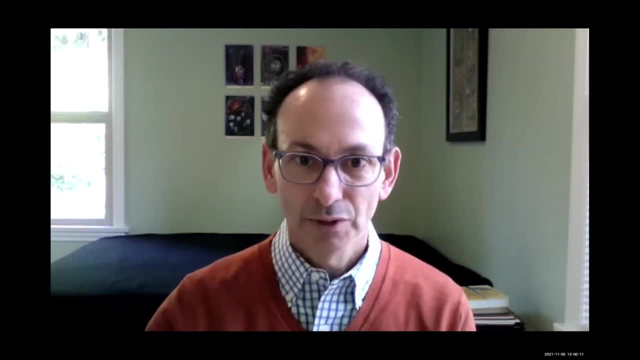 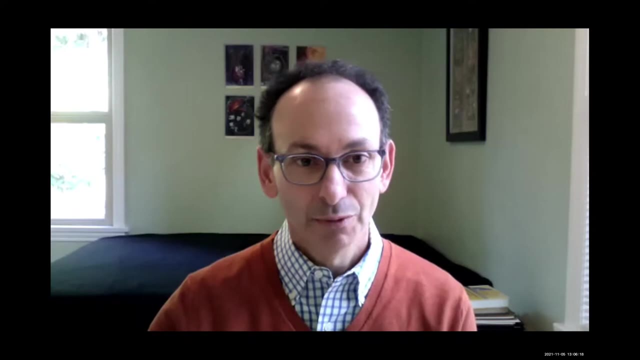 and the national defense science and engineering graduate fellowship, after which he joined pnl as a linus pauling postdoctoral fellow and he is now a research scientist specializing in national security, material processing and space nuclear power. he recently received the ronald brovinsky award for early career- exceptional achievement. 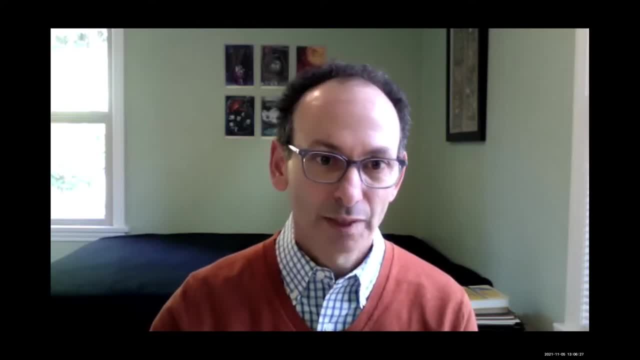 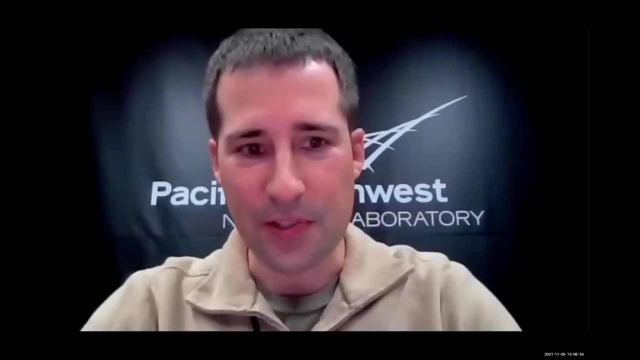 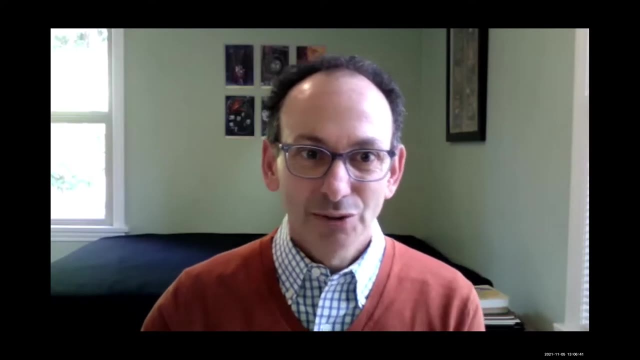 for his work on blue toning 238 soul gel for space heat and power. so congratulations, jeff. would you like to say hello? thank you, it's a pleasure to be here with you all today. okay, thank you, and so next i'll introduce jake leachman, who's an associate professor. 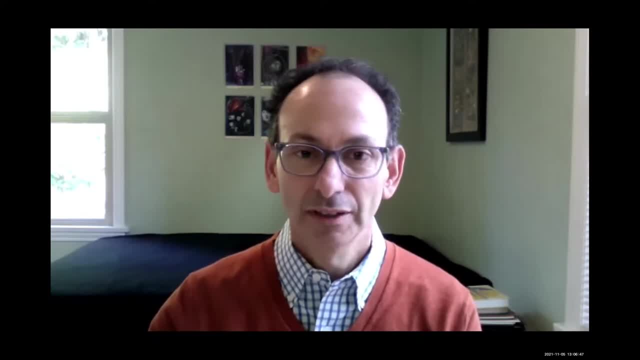 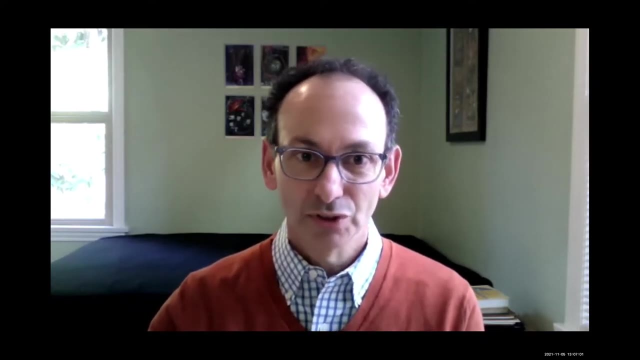 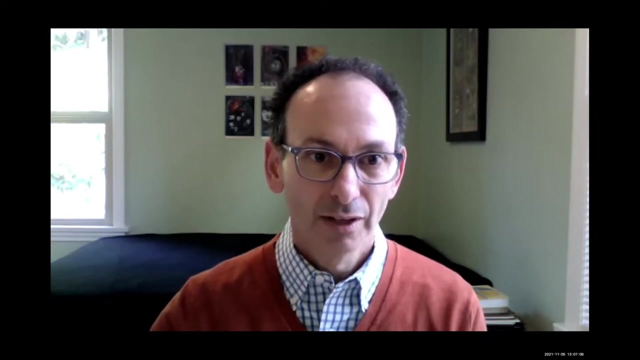 of mechanical and mechanical and materials engineering at washington state university. he founded the hydrogen properties for energy research, the laboratory to advance cryogenic hydrogen systems. his interesting is ms research was adopted as the foundation for hydrogen, hydrogen fueling standards and custody exchange. he's received the roger w boom. 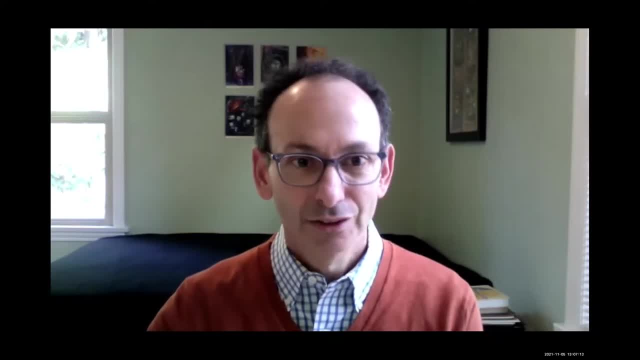 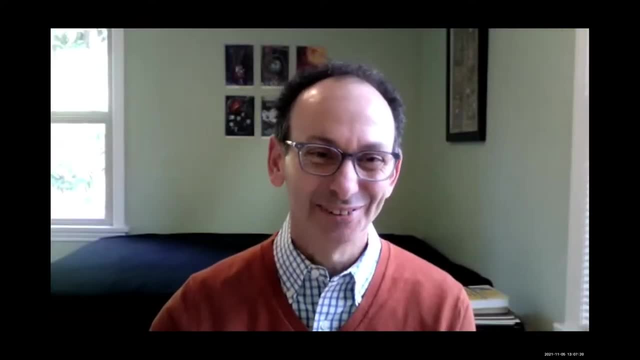 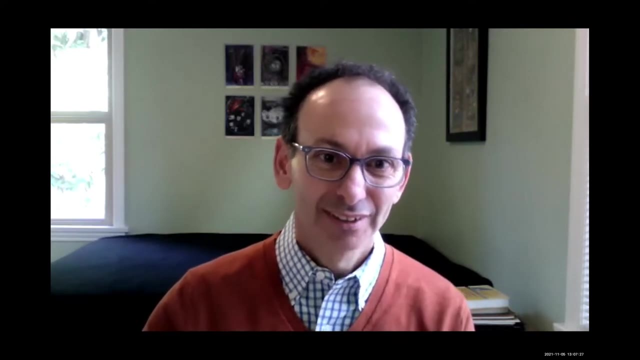 award from the cryogenic society of america. jake, would you like to say hello? thanks, siri, for inviting the cook to the room. absolutely my pleasure. next, i'd like to introduce uh, josh smith. josh is a professor of computer science and engineering at the university of washington. 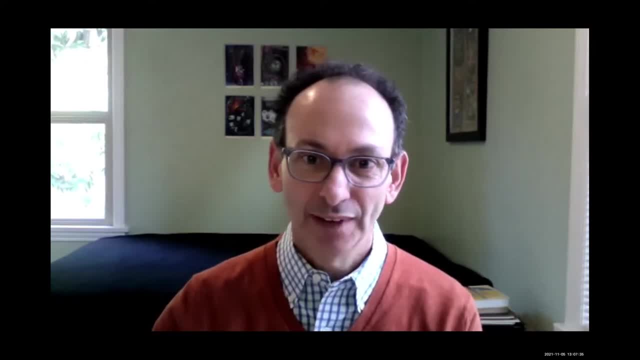 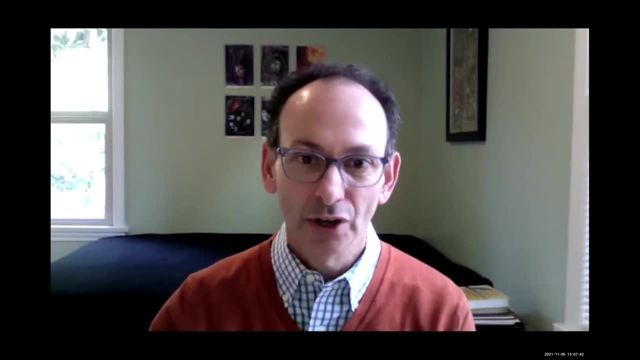 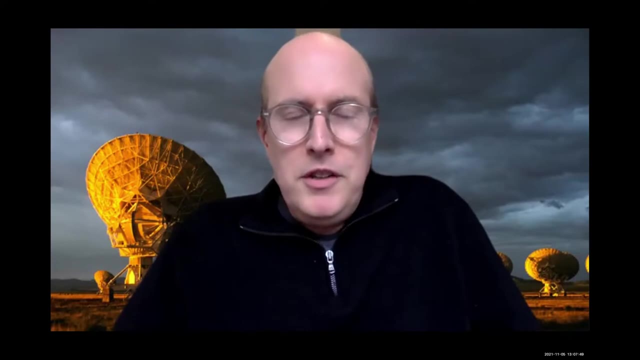 specializing in sensor systems and interesting ways to power them with applications for robotics and ubiquitous computing. his current projects include battery free mobile phones and rf powered cameras. josh, would you like to say hello? sure, happy to be here. yeah, i'm also a professor in electrical and computer engineering, and 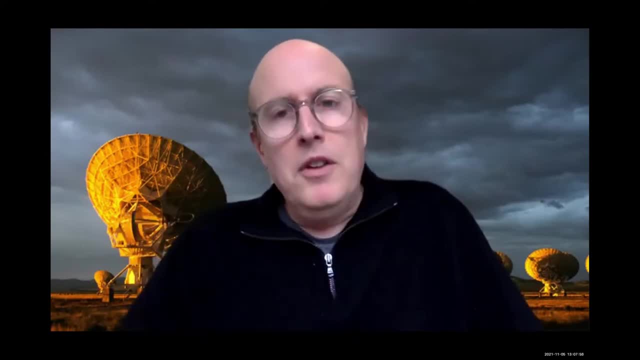 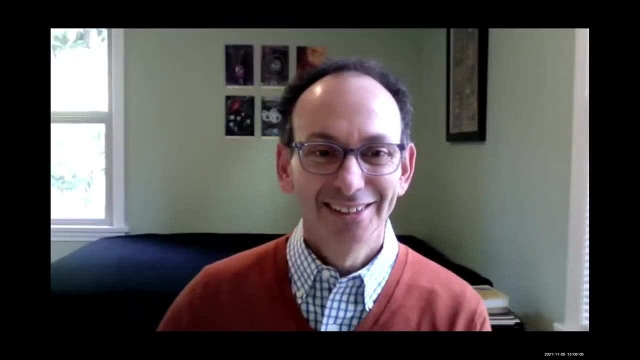 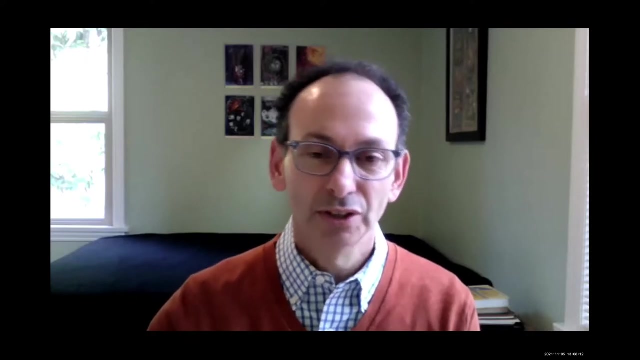 related to power in space- a little bit less propulsion, but I'll show you some of what we're doing on power in space context. Great, look forward to it. Okay, and with that I'll turn the floor over to Roger Myers, who will give a brief tutorial on the general subject of space. 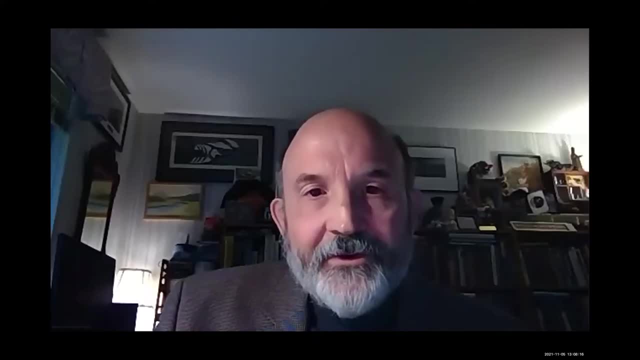 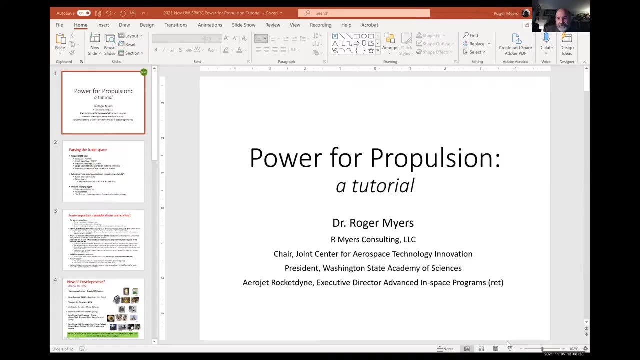 power. Okay, Roger, take it away. Okay, thank you, Yuri, appreciate it. I'm going to pull up my, I'm going to share a screen, pull up my charts and people should not panic, I'm not going to. 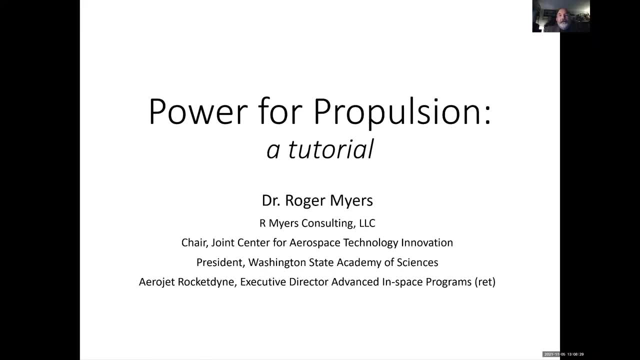 I'm going to go through it pretty quickly, but I do think it's important for us all to have some context and understand you know what it is that the field of space power for propulsion really involves. It's a very broad field. 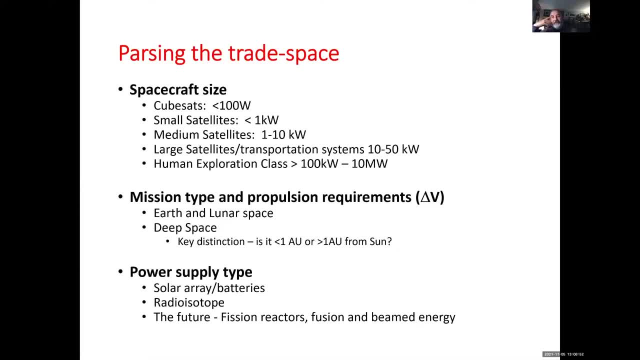 So just when we talk about this, this space quote unquote, you parse it into spacecraft size. We range from CubeSats to human exploration class missions. You know, CubeSats are are under 50 watts in many cases. We then we have small sats and medium class satellites. 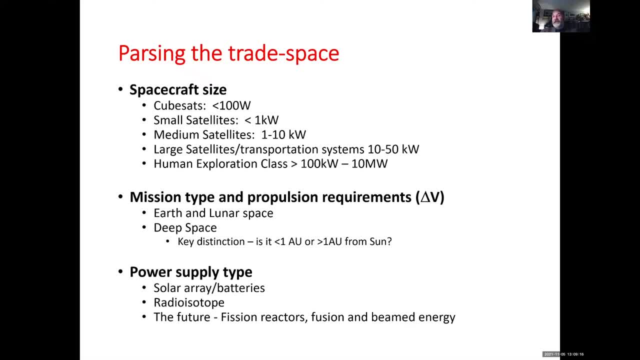 that are one to 10 kilowatts. We have large satellites, 10 to 50 kilowatts of of electrical power And of course then the human exploration class. you know really big, big exploration missions, like human missions to Mars, where there we're talking about hundreds. 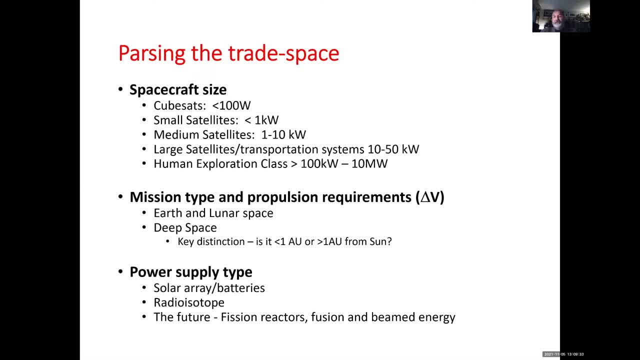 of kilowatts to multi-megawatt electric systems And it's important to realize that today we have primarily flying medium satellites and below We have a few satellites at the 20 to 25, maybe topping out at 30, to out at 30 kilowatts of power. 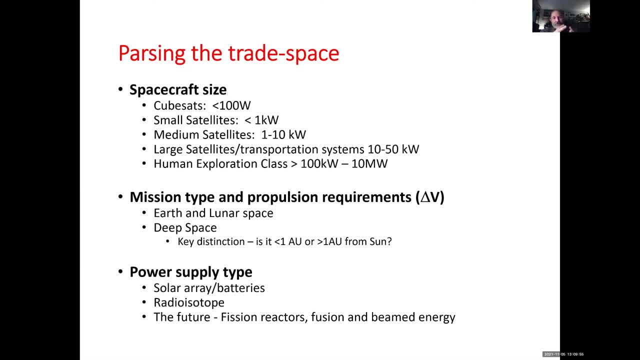 We do have the International Space Station, which is the highest power vehicle by far flown in space today, and it's at 200 kilowatts. Those arrays, the power system for that is big enough so that you can see it with binoculars from the ground. 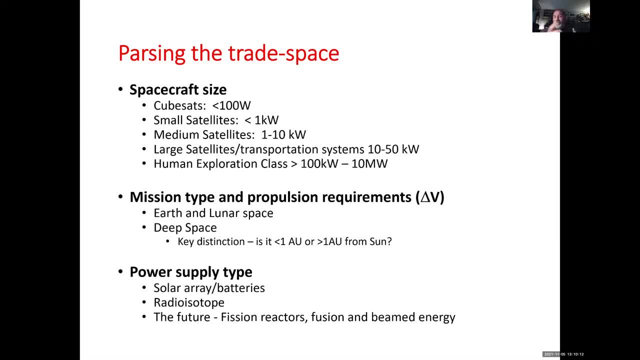 So they're very large solar arrays. I'll talk a little bit more about those as we go forward, But it's really important to realize that we fly a lot of spacecraft today and they top out at about 10 to 30 ish kilowatts. 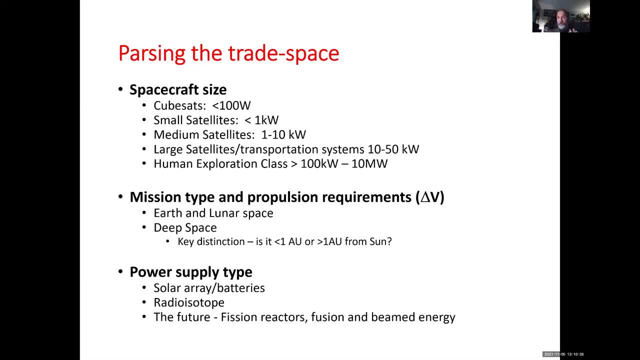 of electrical power. So that's spacecraft size. that's one way to parse it. Then mission type and propulsion system requirements are. it's a different way to look at this parameter: space. Is it an earth orbit mission, a lunar mission, or is it deep space? 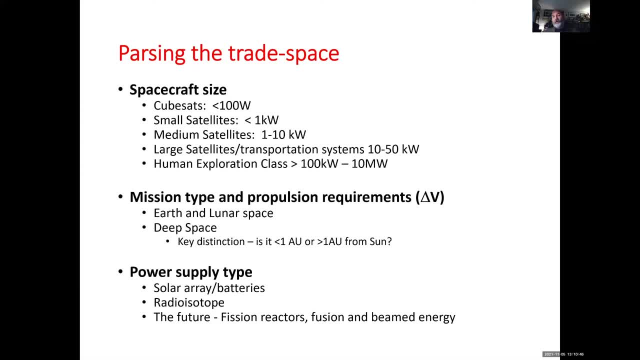 And if it's deep space, are you going toward the sun? where you're, the power from the sun will increase as you get closer to the sun or away from the sun, where the power of course drops as one over R squared from the sun. So we got to understand what the mission type is. 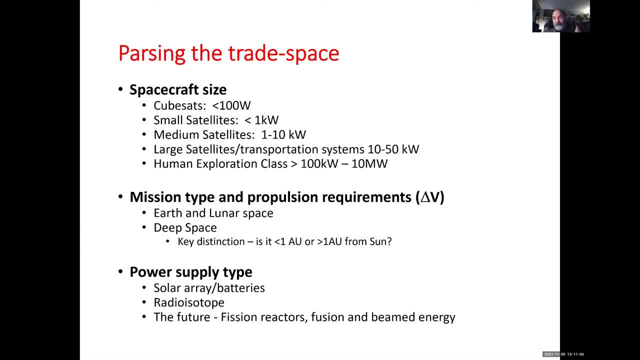 And then, what are the propulsion requirements? Is this a fly by mission for deep space, where you essentially are just doing attitude control of your vehicle as it goes by your target, Or are you going into orbit, which requires a lot more propulsion to go into orbit? 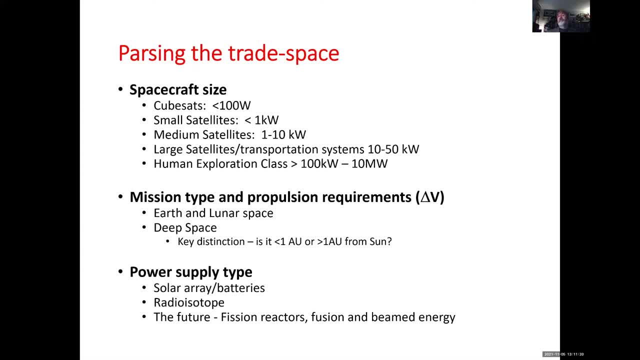 and control that orbit? or even more, are you going to land on the surface where you need even more propulsion requirement? So again, understanding those are. it's another key set of variables that you need to assess when you're thinking about power for propulsion. 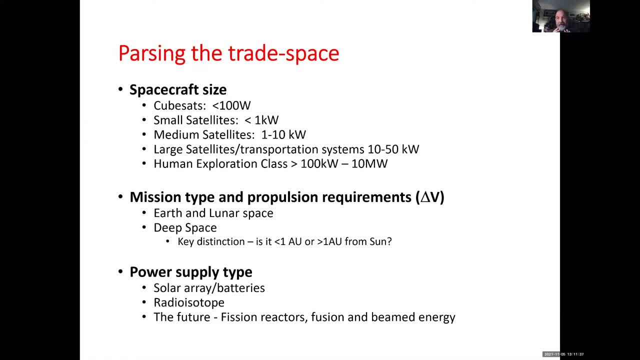 And then, of course, there's the power supply type. Today, everything we fly almost exclusively- and I'll talk a little bit more about the exceptions- are solar arrays with batteries, And you have to have batteries on solar power power systems because sometimes you go into shade. 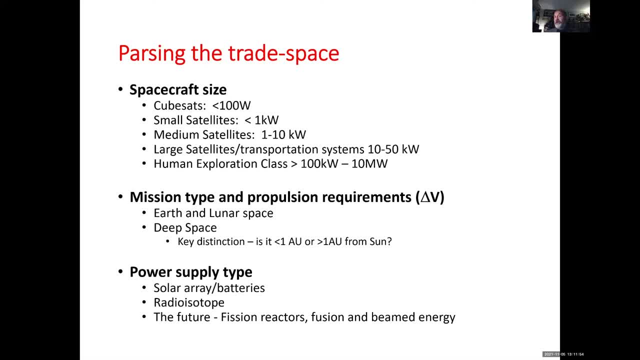 Even deep space missions that, for example, today are flying to Jupiter with very large solar arrays to deal with the increased distance from the sun. You have to have a battery system, because sometimes it goes behind the planet, your target planet, And that battery system has to enable your spacecraft. 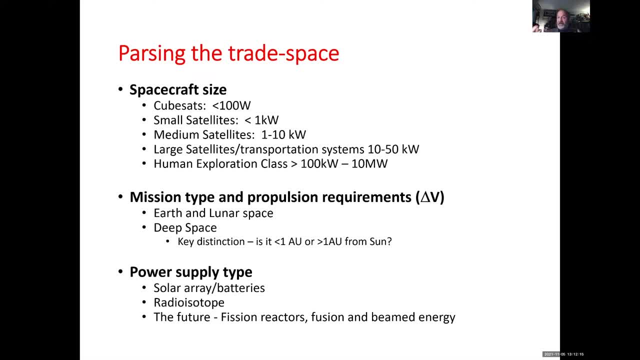 to stay healthy and do its job when the solar arrays are not illuminated. So solar arrays and batteries, they're radioisotope power systems, like those on Curiosity or Perseverance, the rovers on Mars, but those same systems are gonna fly a quadcopter on Titan. 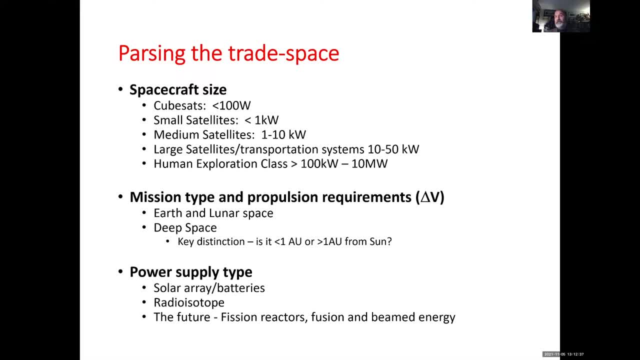 the Dragonfly mission, So those radioisotope systems today all use plutonium- I'll talk a little bit more about that- And there are all kinds of costs and issues associated with using plutonium. And then of course, we have the future. 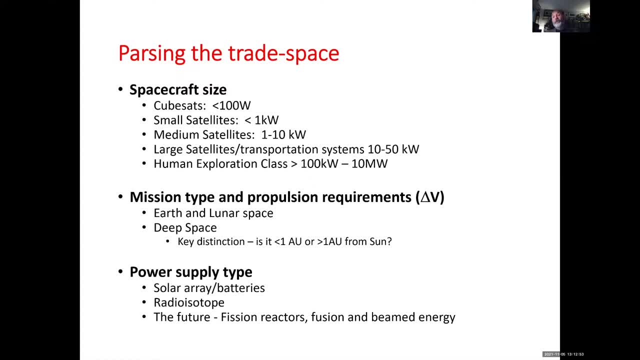 As Yuri mentioned during his intro, I just co-chaired a committee with the National Academy looking at fission-based propulsion systems, either nuclear thermal or nuclear electric. But then of course there are also emerging fusion and beamed energy systems. Those are all pretty futuristic. 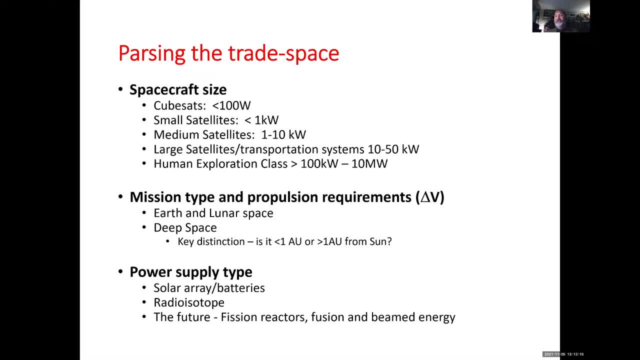 I mean, I don't know if you saw the paper today, but even today for terrestrial power systems there was a big headline in the Seattle Times that an Everett company, Helion, got a very large, a nice chunk of change for their system. 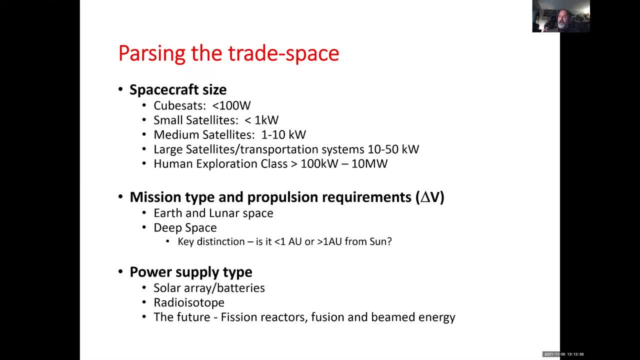 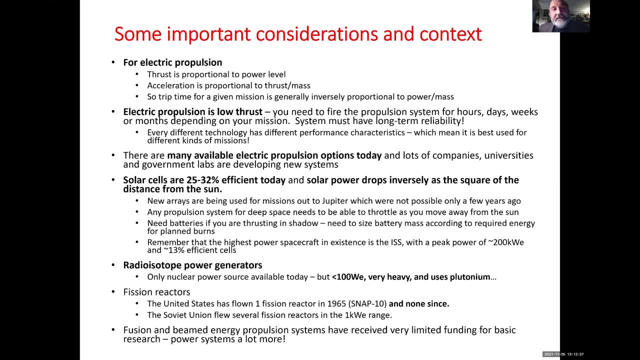 So that's very exciting for terrestrial power systems. But applying those systems to space propulsion is a different set of challenges. So I just again- I'm not gonna read everything here, but wanna emphasize some considerations. Again- electric propulsion thrust is proportional to power level. 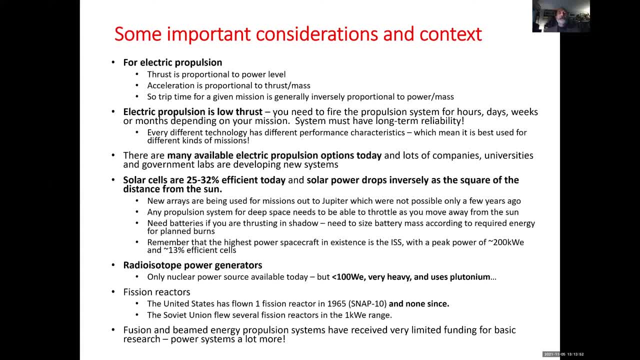 So if you want more thrust, you have to add power. Acceleration is, of course, proportional to thrust divided by mass. This is just Newton's law, And what that means is that trip time for a given mission- the amount of time it takes you to do a certain mission. 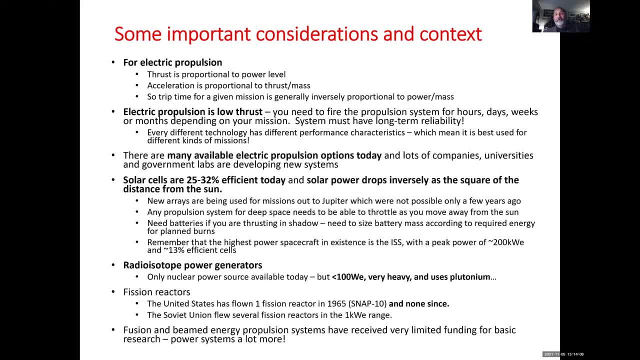 whatever that mission is, is generally inversely proportional to power divided by mass. So the power to mass ratio is a very important scaling criteria And for electric propulsion systems. Another important thing is that electric propulsion is low thrust. These systems have to last a long time. 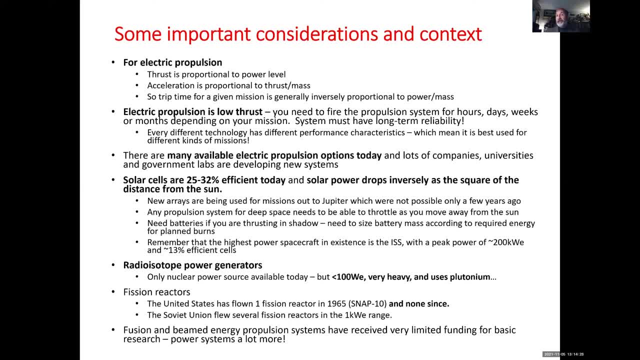 They're not like chemical rockets that fire for seconds or minutes. They fire for hours, days, weeks, even possibly years, depending on the particular mission And every different system, and I'll give a quick introduction to them, to the options. 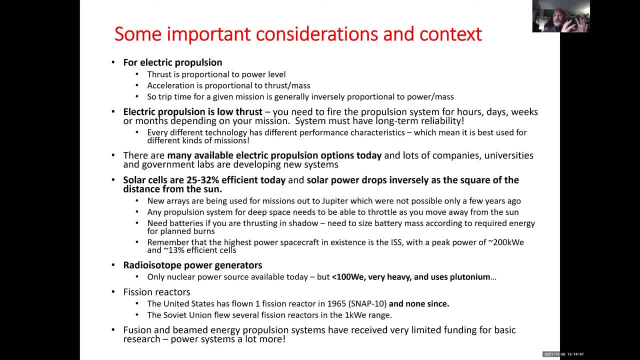 have different performance characteristics, And so what you do is you first parse your mission according to spacecraft size, mission type, requirements, et cetera, And then you look at the options that you have. What are the technology options? What is their current state? 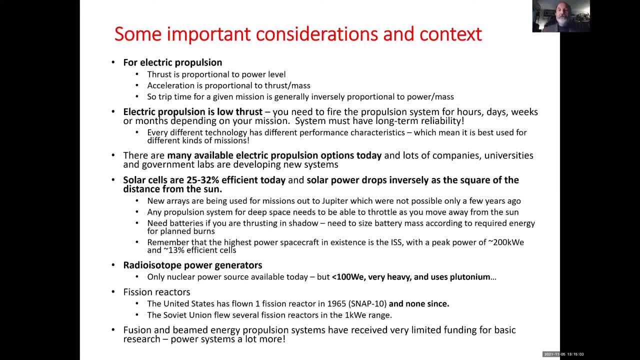 How are they qualified? Do they have flight heritage? Are they you know, et cetera? Okay, so that's on the propulsion side. On the power side, you have solar cells. Well, solar cells today are 25 to 32%. 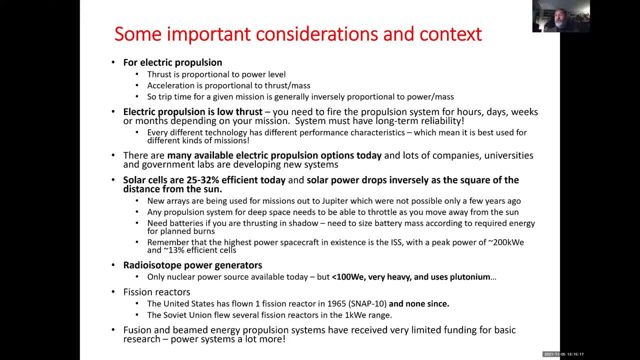 efficient give or take depending on how much money you're willing to spend and the cover glass requirements. And, as I mentioned before, solar power drops inversely as the square is a distance from the sun. So you gotta think about those factors as you are designing, as you are picking your power system. if it's a solar power system. Radioisotope power generators last a long time And, of course, do not depend on solar illumination. So they're great in the shade, but you only get about a hundred Watts from the state of the art radioisotope generator. 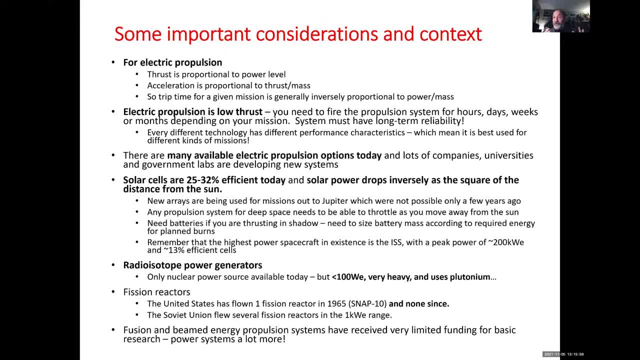 They use thermoelectrics and they use plutonium and thermoelectrics are not very efficient. So you know. you're talking about seven to 10% conversion efficiency of the thermal energy in a typical radioisotope power converter that exists today. 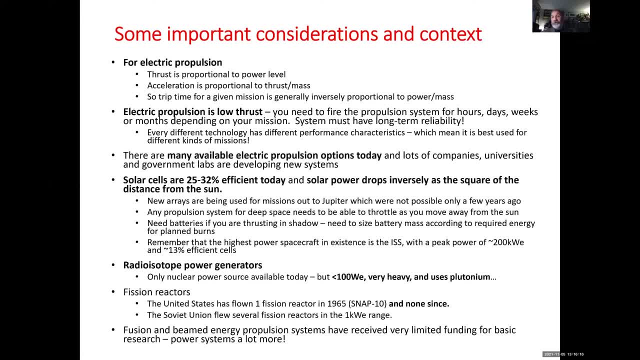 They use plutonium, and plutonium has all kinds of regulatory issues, all kinds of challenges associated with it. it's very toxic, It's, it's dangerous, very dangerous stuff. And then, of course, there are fission reactors. Well, you know, much as we like to talk about the wonders, 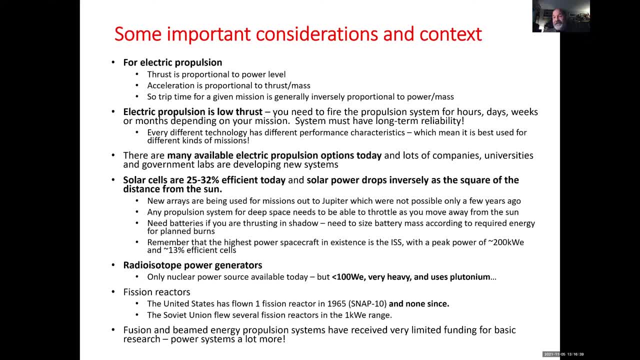 of the potential for nuclear power in space. the United States has flown one in its history in 1920. 1965, and we have not flown a fission reactor since then. Very important to realize that the technology maturity for fission reactors- I don't care what the application is either- nuclear 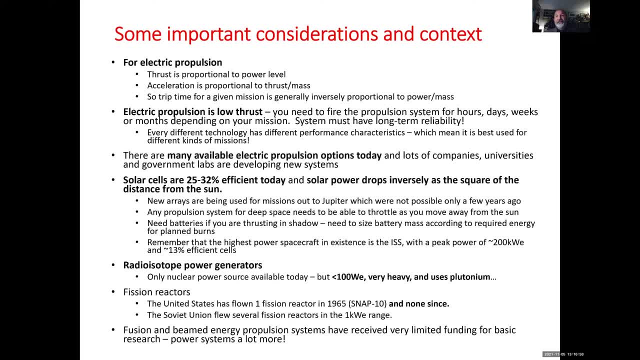 thermal or nuclear electric is. you know that technology is not very mature and there are lots of risks and opportunities, and I refer you to the National Academy's report for more details. I'll talk a little bit about it. The Soviet Union, by contrast, has flown a few Fusion and 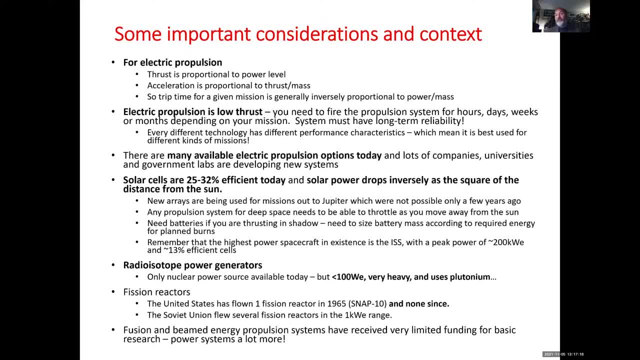 beamed energy systems have received very limited funding for basic research, for propulsion, For power systems. they've gotten a lot more and you know URI has done some outstanding work at the University of Washington and the Zapp Energy and you know there are lots of companies looking at. 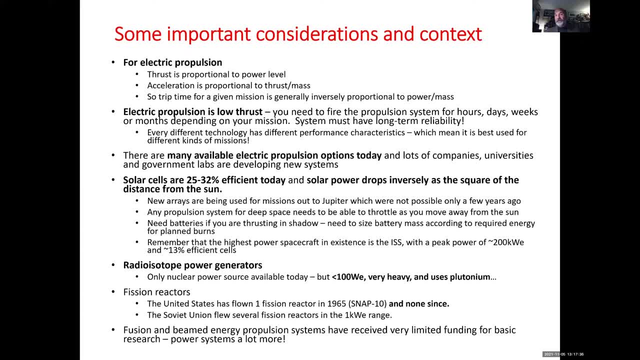 terrestrial power systems and there are several universities looking at the potential for fusion based. So now I'm going to quickly go through some propulsion system, a little bit more detail on the propulsion and power systems and then the tutorial will be over. So just really quickly. 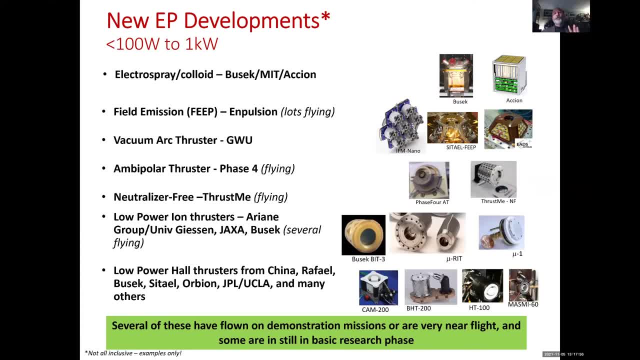 I want to highlight here the diversity of options for very low power electric propulsion systems. right, We range from electrospray, colloid field emission. There are pulse plasma thrusters of different types. Lots of them are flying today on QC. 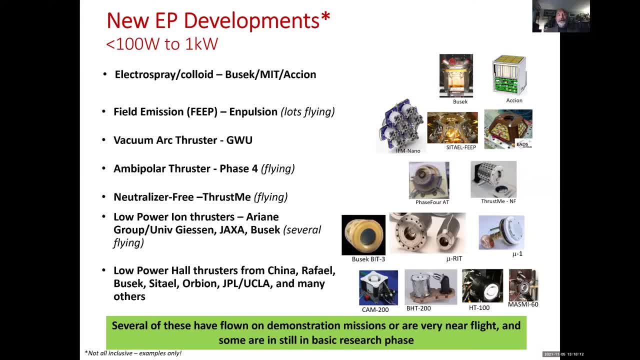 There are very small spacecraft Hall thrusters are flying today, very small ones, and there are many companies and universities working in this area. So again, there are several you've got to remember. they are not interchangeable for different missions. I'll give you a specific example. 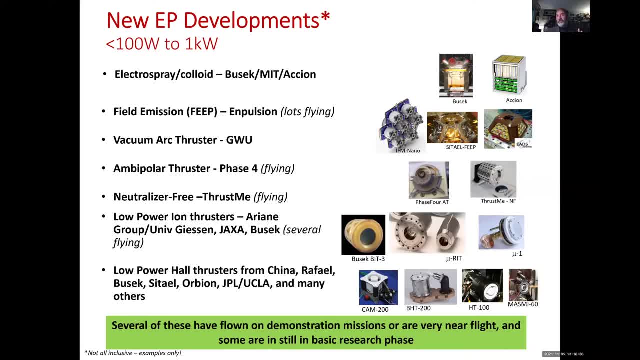 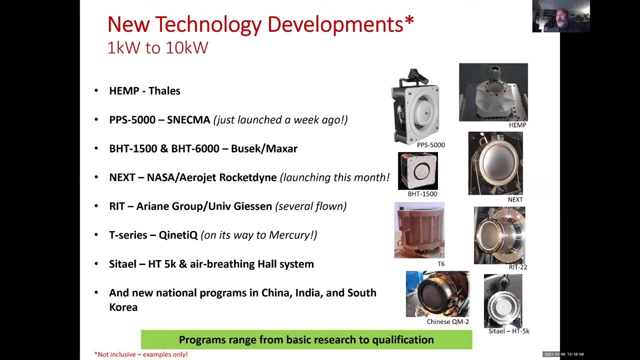 Hall thrusters have lower specific impulse But higher thrust at a given power level than, for example, field emission thrusters. Field emission has very high specific impulse but lower thrust than a hall thruster. And so you've got to understand what your mission requirements are in order to make a selection. Similarly, in the 1 to 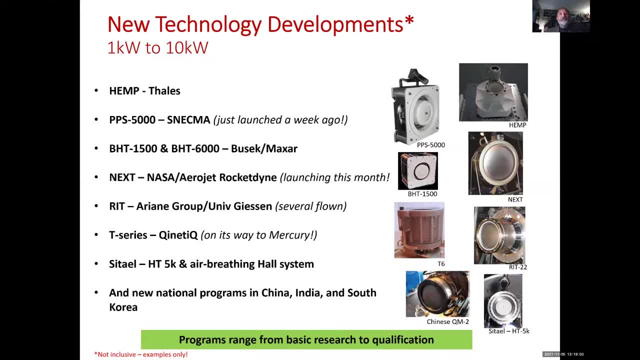 10 kilowatt power range. there are again lots of options. The SNECMA PPS 5000, I pictured it here- launched two weeks ago on a French military communication satellite for the first time. So very exciting for SNECMA and that team, The Aerojet Rocketdyne you know, just here in Redmond. 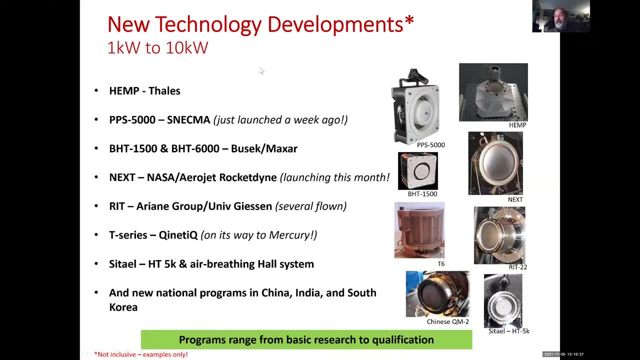 their gritted ion thruster, operating at seven kilowatts of power, will launch next month, this month on the DART mission, So that propulsion option will be flying in a month. There are several options here that have flight heritage. Aerojet Rocketdyne has flown the XR5. 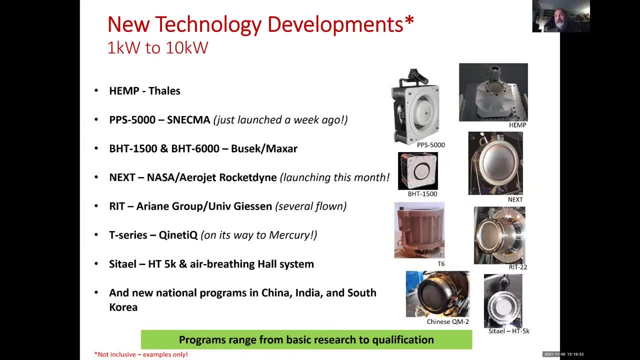 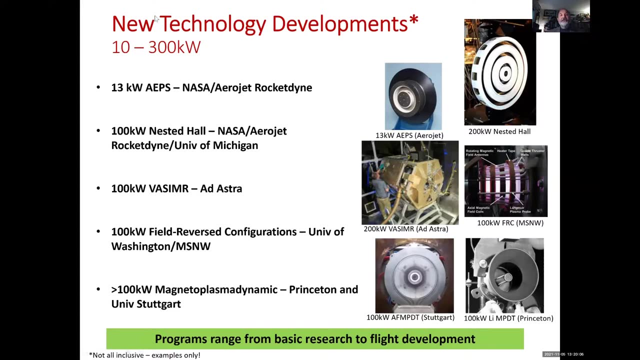 I don't even put a picture of that here. That was actually a system that I led the development of, And there are 40 or 50 of those flying. So again, lots of options. As we go to higher power, there are fewer and fewer options. Right now, Aerojet Rocketdyne in Redmond is developing a 13. 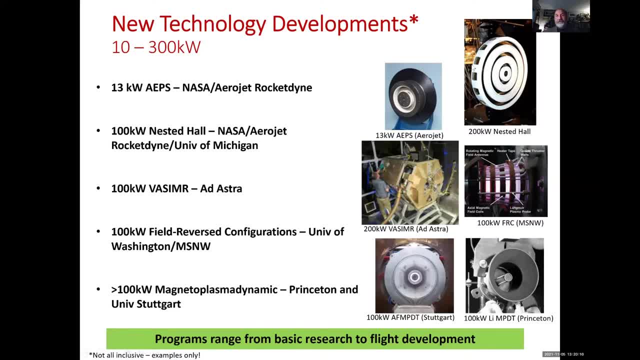 kilowatt hall thruster And the SNECMA PPS 5000 will launch next month. So again, lots of options, And Aerojet Rocketdyne is developing a 13 kilowatt hall thruster And they also worked with the. 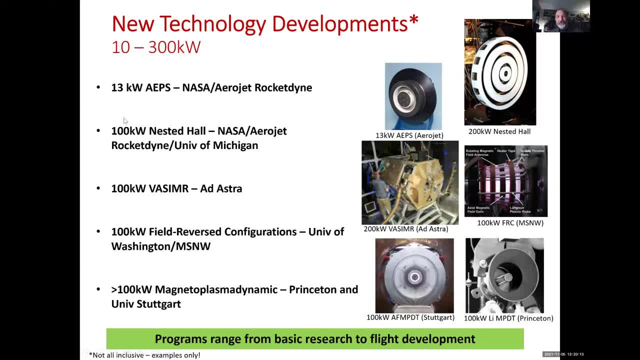 University of Michigan on the 100 kilowatt hall thruster. Ad Astra, led by Franklin Chang-Diaz, has the VASIMIR thruster, And there was some work at the University of Washington on the field reverse configurations. So all good stuff. And then Princeton and the University of Stuttgart. 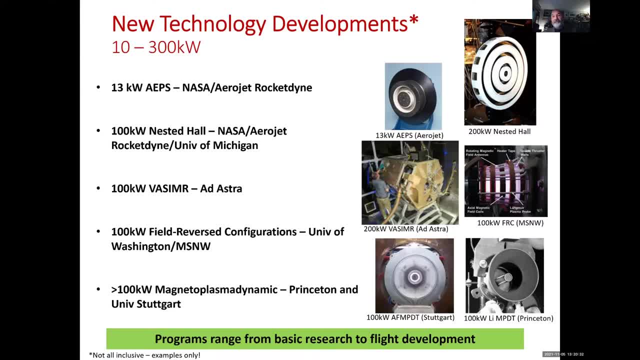 have done a lot of work on applied field or just magnetoplasmic dynamic thrusters: Paul Krugman, MD PhD, PhD, PhD in Mechanical Engineering, MD PhD, PhD, PhD, PhD, PhD, PhD, PhD. 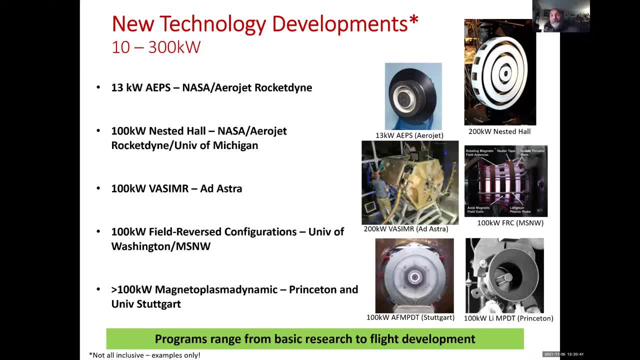 Again, as we go to higher and higher power, there are fewer and fewer options. Why? Because there are fewer and fewer emissions, So there isn't the pull. The market is not pulling in this direction yet. It's just starting to. 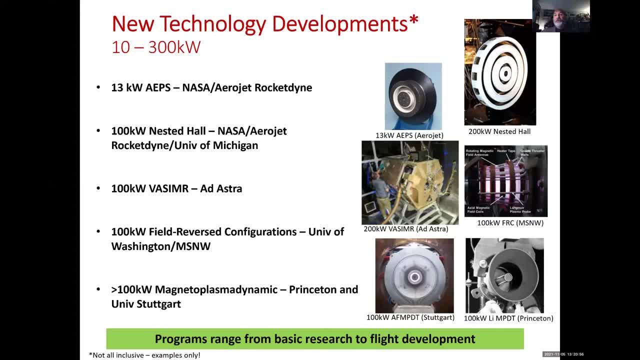 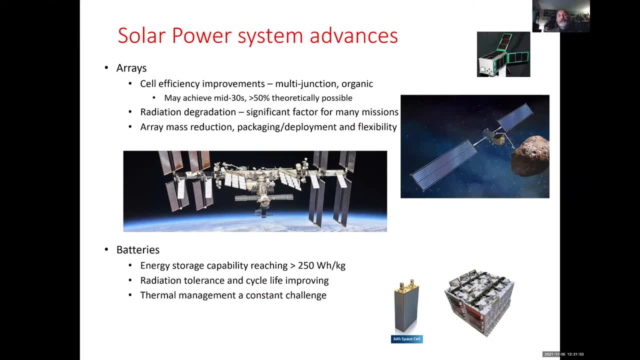 So primarily this is university research or a small company. So now switching gears to the power side. I mentioned already the solar power. you know, typically between 27% and 32% efficiency, but there is theoretically opportunity for over 50% efficiency in solar cells. 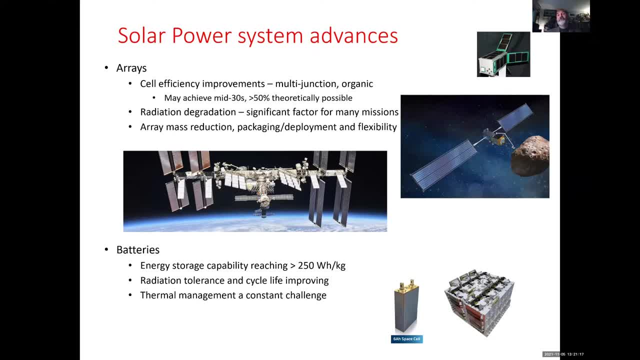 That would be super exciting and truly game-changing if that happens. But there are some real important things: Radiation degradation. As you know, one of the challenges of Earth space is that we have the Van Allen belts And if you use solar arrays to move up and down through the Van Allen belts, you take 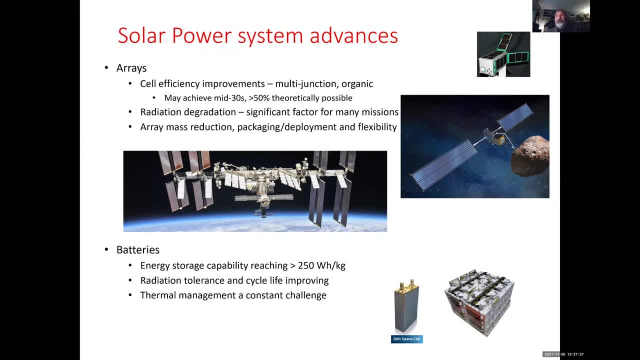 about a 10% Hit in the performance of a solar array every time you transition the Van Allen belts. It's sensitive to cover glass cover, glass selection et cetera, But it's a significant factor for many missions. It's one of the big challenges of Jupiter solar arrays. 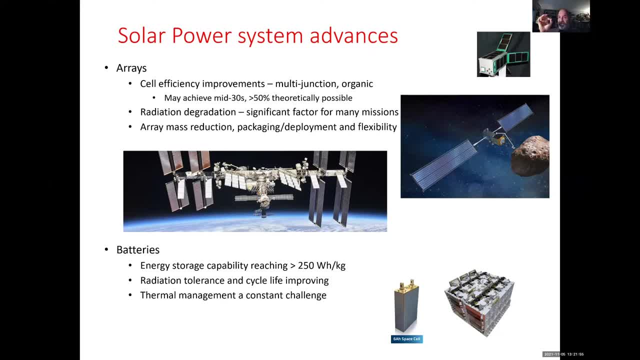 Lots of work going on now in array mass reduction. It's not just about the solar cells but about the array structure, how you package these enormous solar arrays and how you deploy them. Are they flexible? Those kinds of questions. I've shown here a picture of a CubeSat with body-mounted solar arrays. 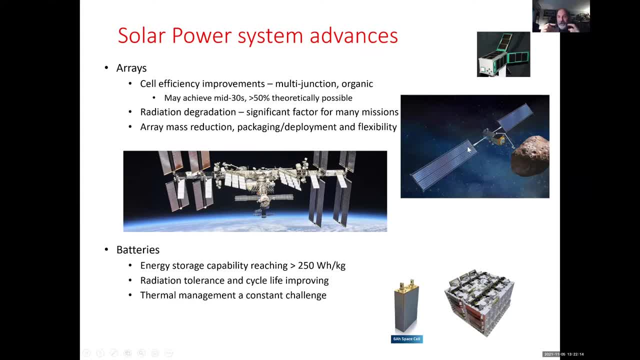 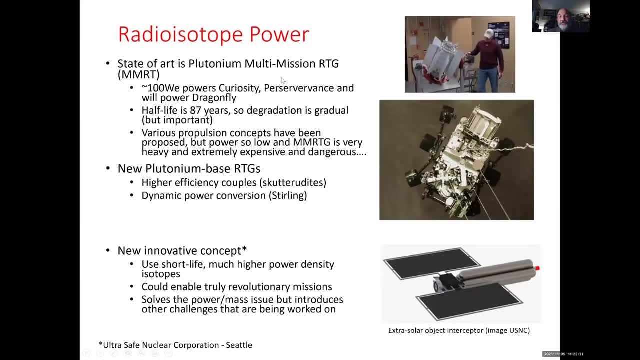 And then this is a much larger. this is actually a rollout solar array, where the solar array is rolled up into a tight package and it unfurls after launch. And then here's the International Space Station with all of its large, enormous solar arrays. 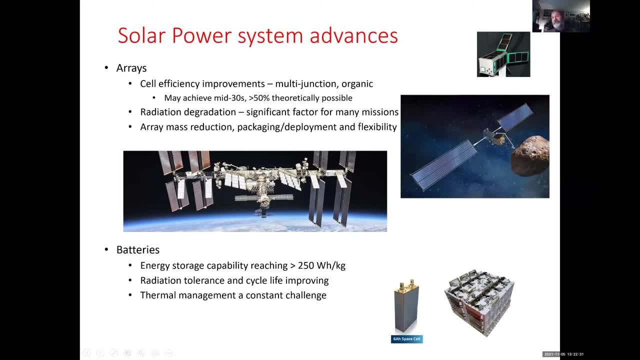 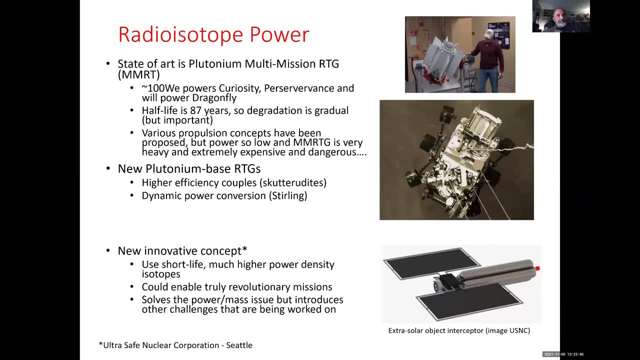 And batteries are very important. They're a significant fraction of the mass of any spacecraft power. You've got to worry about radiation tolerance, thermal management, right? They get hot when you release the energy, So radioisotope power Again. I'm trying to go fast and just introduce you to this very broad topic. State of the art is the MMRTG. It's built by the US government and Aerojet Rocketdyne- Aerojet Rocketdyne actually does the manufacturing of it, And here it's pictured on the Perseverance rover. 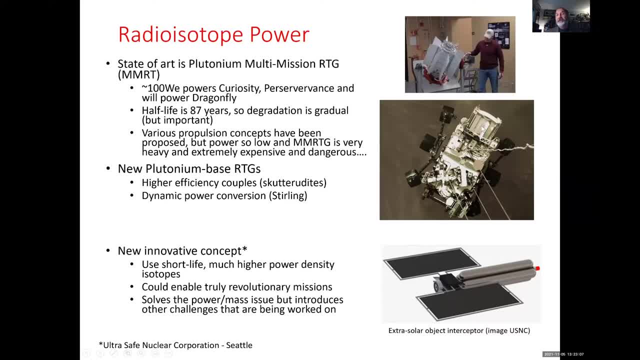 It's the Perseverance rover. It's the Perseverance rover. It's the Perseverance rover. The Perseverance rover is lowered to the surface of Mars And you can see how big it is relative to this person in the top picture. 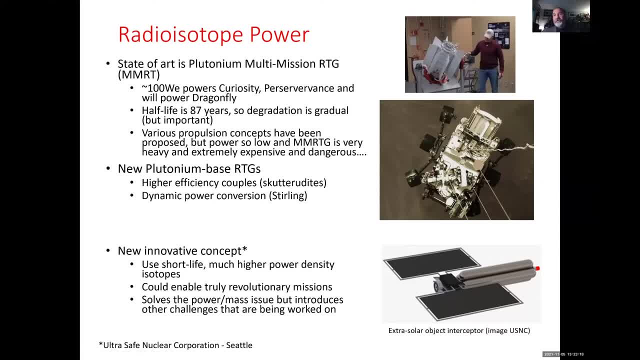 There are some propulsion concepts that use the RTGs. The problem is the RTG is very heavy and not very efficient and only produces about 100 watts of power. So you're talking about the low end of those propulsion options that I showed. There are some new. 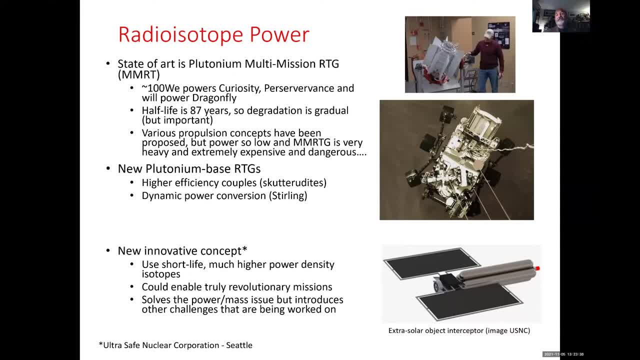 So you're talking about the low end of those propulsion options that I showed. There are some new technologies for RTGs, There are some new, more efficient thermocouples to produce the power And there's a dynamic power conversion system that has been proposed. 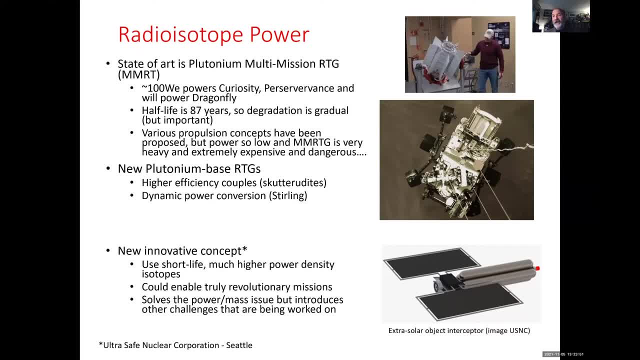 A lot of work happened about 15 years ago. That program did not succeed. Now it's coming back because technology has advanced and we hope it will. I did want to point out a Seattle-based new concept which is very exciting, And that's using non-plutonium isotopes. 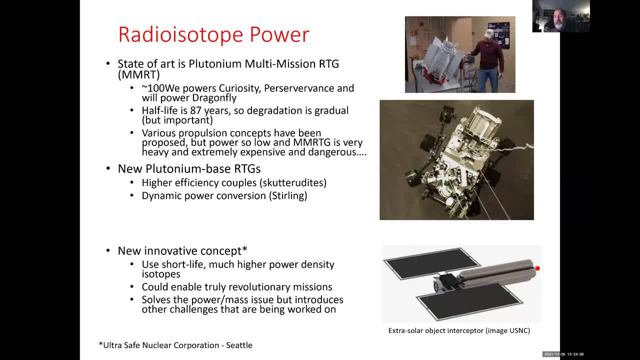 So other isotopes that are short life but much higher power density, And this was recently funded by NASA through their NIAC program And it's here at the UltraSafe Nuclear Corporation here in Seattle, And they have proposed an extrasolar object interceptor. 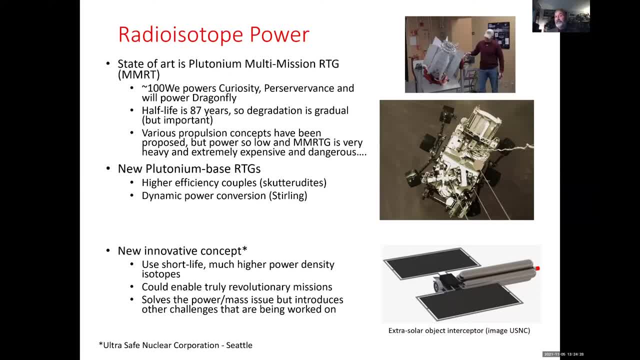 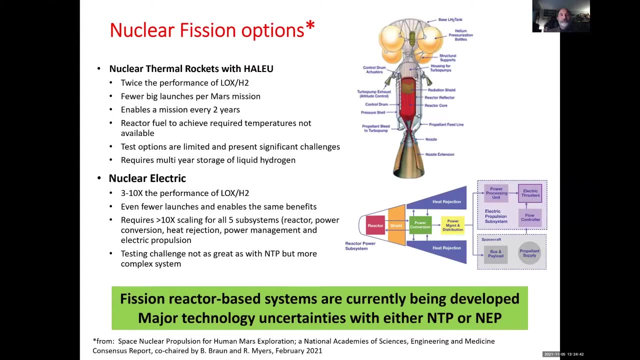 In fact, if you can read about this online, the capabilities are amazing. actually It's very low TRL, but it is a very exciting project And it's creating innovation in radioisotope power systems, Fission concepts. There are two nuclear thermal rockets, where, and Jake Leachman will tell us- 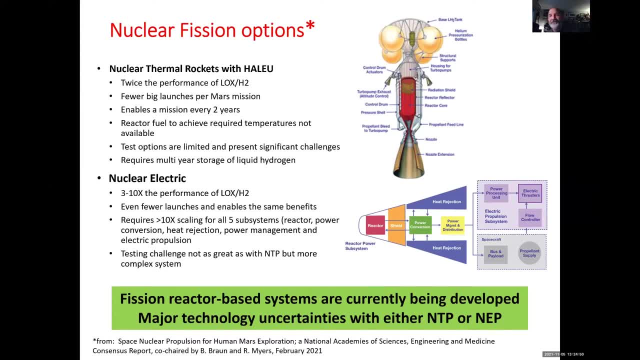 about the challenge of storing hydrogen to support a nuclear thermal rocket. But fundamentally, a nuclear thermal rocket is like a chemical rocket, except you've replaced the combustion chamber with a nuclear reactor. The challenge is that you have to have a nuclear reactor. You have to have a nuclear reactor. 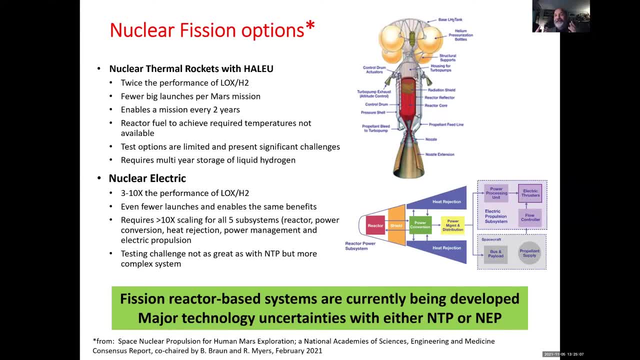 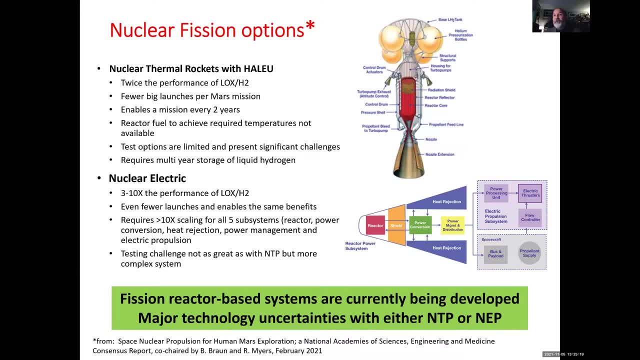 There are, lots of there are, and also we have to test it. How are we going to test a nuclear reactor? I'm sure that one of the other panelists will talk about the challenge of testing fission systems on the ground and then launching them. 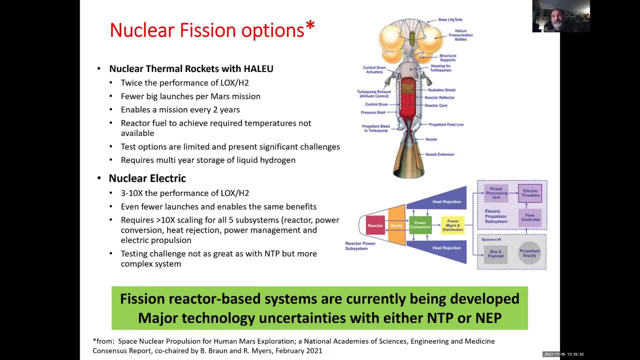 I should remind everybody that fission systems will be launched cold. They will not. they will have at most undergone a few seconds of testing. So the radionuclide products in the fission reactor prior to launch will be very, very small. 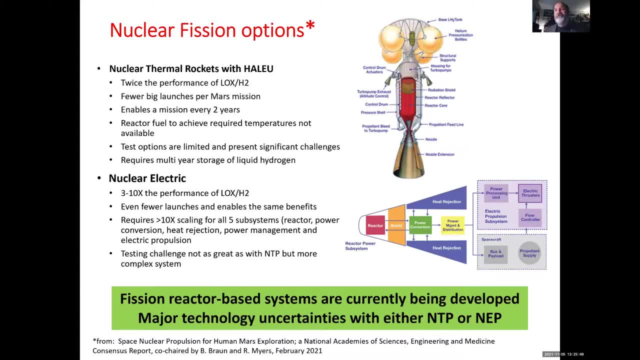 So they're. they're at a. it's pretty low risk to launch fission reactors, And I would contrast that to plutonium reactors where the plutonium is quite, quite nasty. So, but the test options are very limited. How do you qualify these systems? 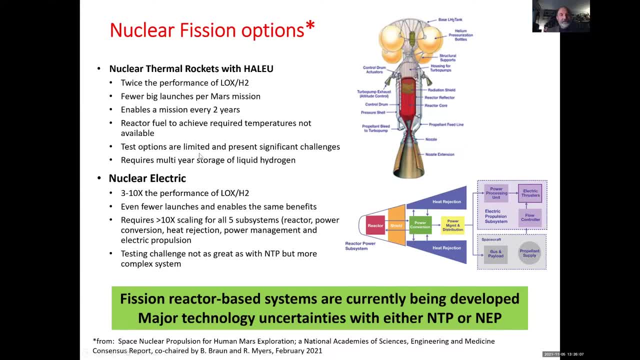 How do you qualify these systems? How do you qualify these systems? And, as I said, Jake will tell us about multi-year storage of liquid hydrogen to support that. Then there's the nuclear electric option: Offers even higher performance, even fewer launches, but it's a more complex system. 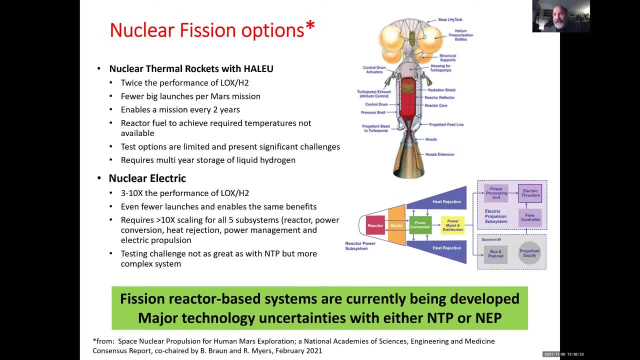 Instead of having a simple thing that looks like a chemical rocket, you've got a reactor or a power conversion system. you've got to manage the power- You're talking about a few megawatts of power. You've got to reject all that heat, so enormous radiators are. 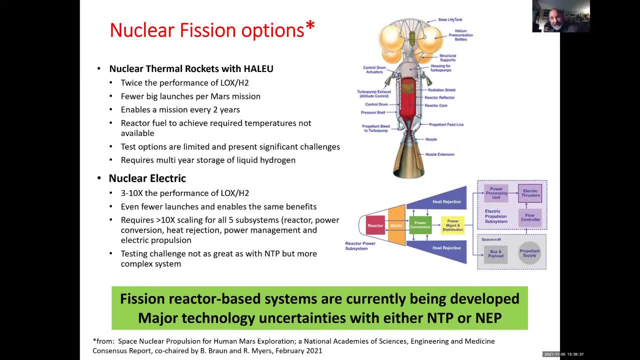 involved, and then you have the electric propulsion system in addition to that. So there aren't the fundamental challenges, the materials and testing challenges that you have with nuclear thermal rockets, but there are a larger number of potentially small, of maybe smaller challenges. 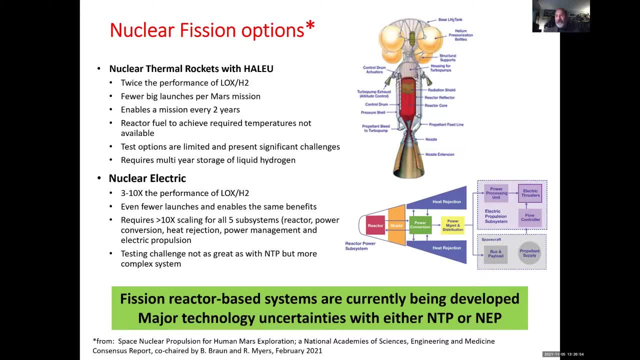 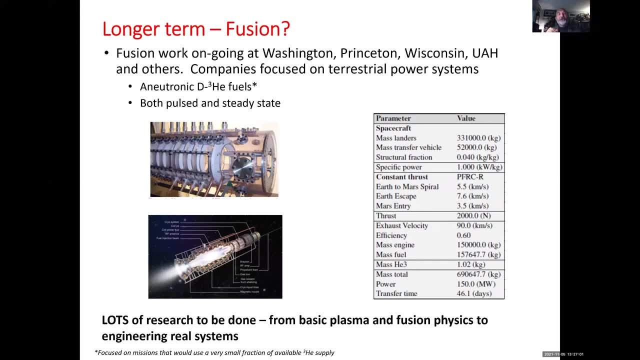 So that contrast, again, we talk about it quite a bit in the National Academies report and I refer you to that for more details because I'm sure Yuri wants me to finish up. Longer term, there's fusion and you know, as I mentioned, 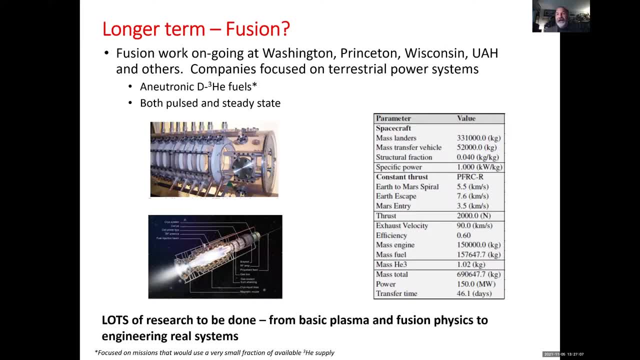 there was a big headline today in the Seattle Times. you know great work going on terrestrial power system. but working on converting those systems from terrestrial power to space propulsion is a challenge in and of itself. But there is work going on. Yuri's done some. Princeton Wisconsin, University of Alabama, Huntsville. 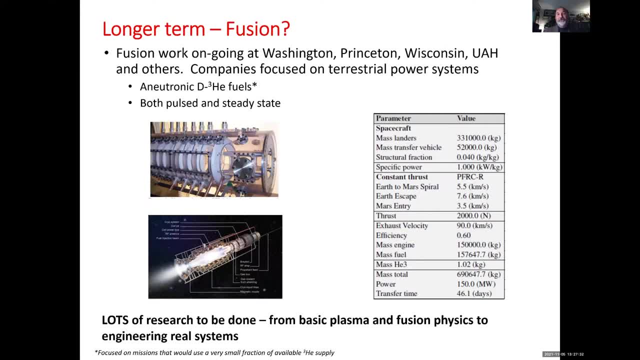 There are several universities looking at fusion systems And Primarily we're focused on aneutronic fusion- and I- perhaps somebody will talk about that, another one of the panelists- and there are both pulsed and steady state systems. 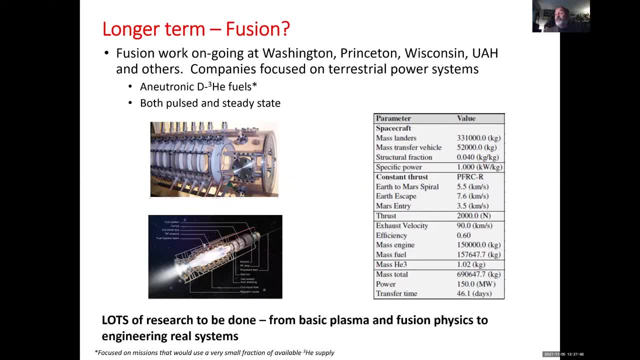 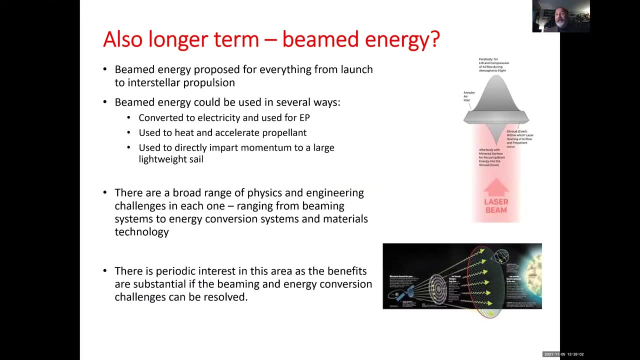 If this can be solved, if these challenges can be solved, of course, fusion would be truly revolutionary, And there are several basic research efforts ongoing now that, if successful it would be, it would be amazing and very exciting. And then we have the last concept. 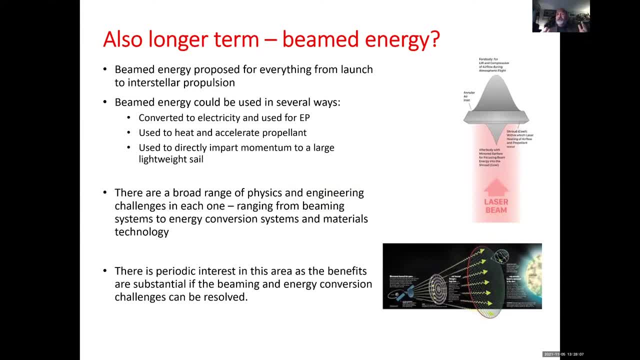 The concept that I'm going to talk about: beamed energy. It's been proposed for everything from launch- That's what this picture is here, using a laser beam to heat gas inside an open nozzle- to interstellar propulsion, and that's what the image is down below. 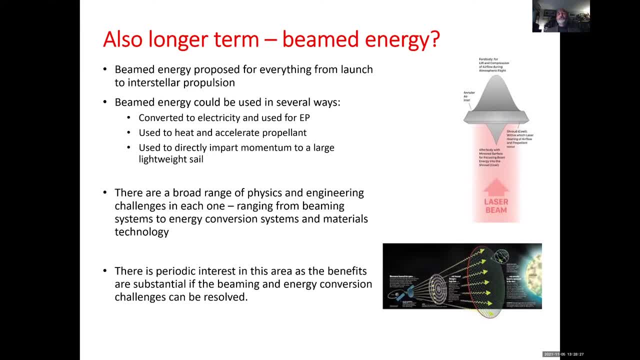 You can use it in several ways. You can use it to convert the beamed energy to electricity and use it for electric propulsion. You can heat the propellant directly, or you can impart momentum just through photon reflection onto a large light sail. So there are lots of ways of doing it, but there are also huge challenges. 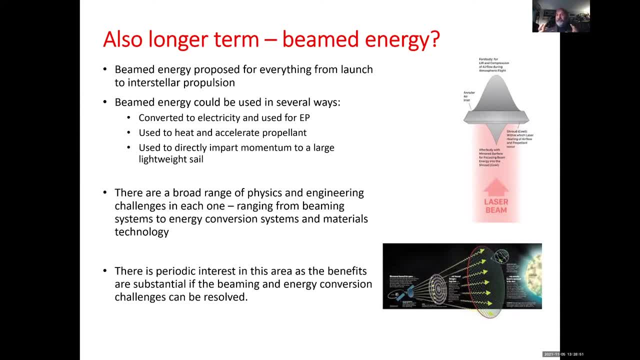 And right now these are very immature concepts. They're again. they're very interesting physics, but making any of these beamed energy? I've done quite a bit of work in this area myself and have not succeeded in finding a way to make it work. 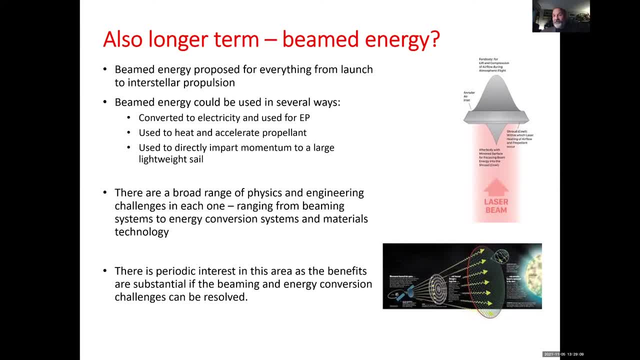 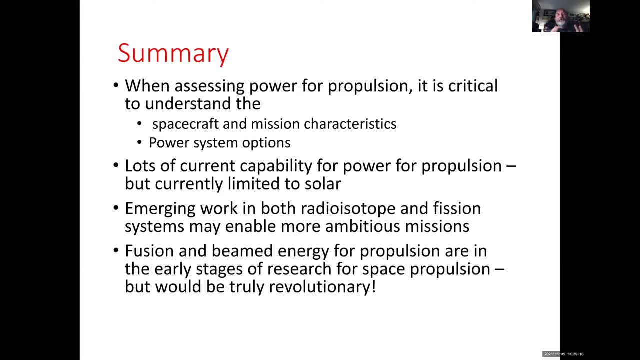 So I. but again, if we can resolve those challenges, it's a great opportunity. So, to summarize, just hearkening back to the very beginning of this tutorial, when assessing power for propulsion, it's critical to remember how big is your spacecraft. 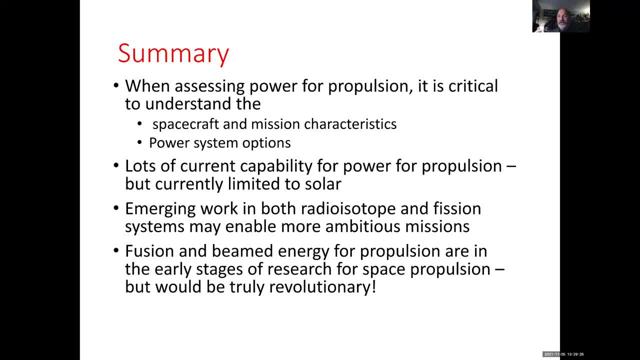 that you're talking about and what are the propulsion requirements that you that you're trying to satisfy and what are my power system options? right, And there's solar radioisotope And fission potentially. how near-term are we talking right? 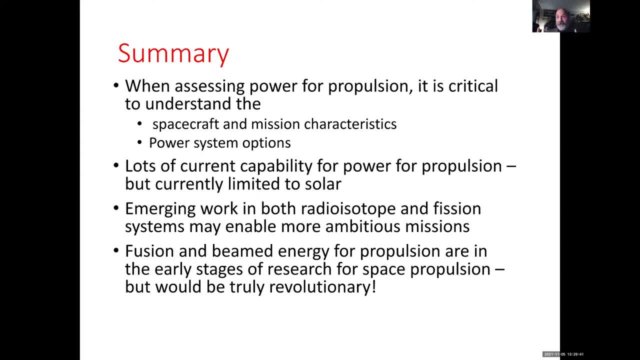 All of those questions come to bear. There's lots of current capability, but it's all solar and batteries. There's emerging work. There's a lot of new technology being developed, but it's low technology readiness level. So we have a lot of work to do in order to finish development, testing, validation. 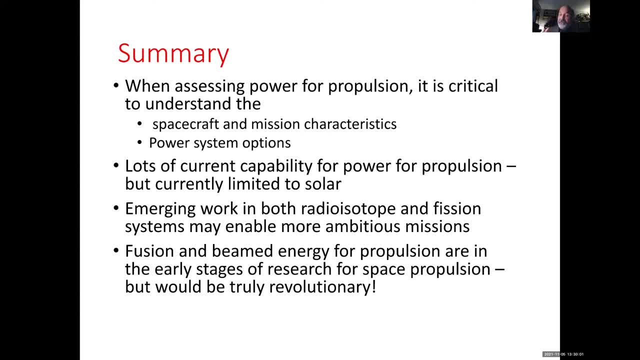 qualification and then go into production- Very exciting. We're looking forward to the future of our strategic projects and where we can start to amplify those opportunities with many of the advanced concepts. So that's my tutorial. I hope I at least set the stage for some of the other discussions. 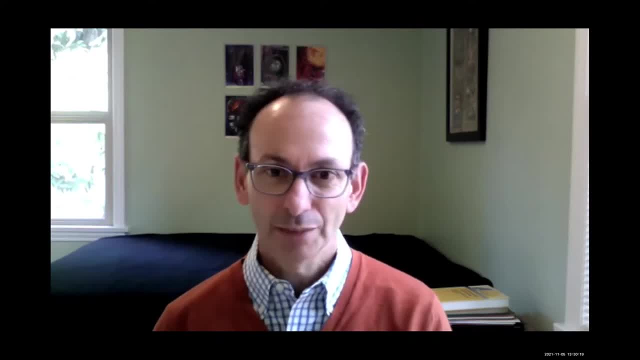 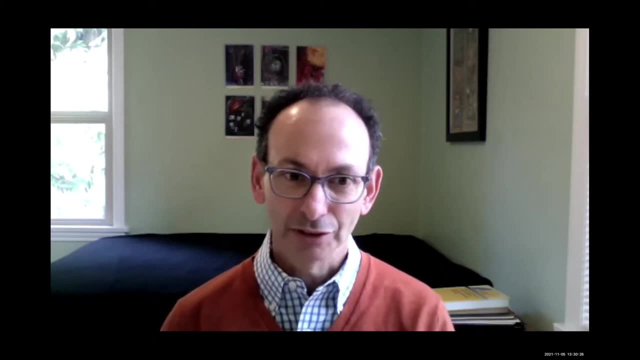 Thanks. Thank you, Roger, That was really great. Yeah, I think you did an excellent job of really establishing a foundation and it's really going to set the context for our panel discussion. So I mean you touched on many interesting topics there. 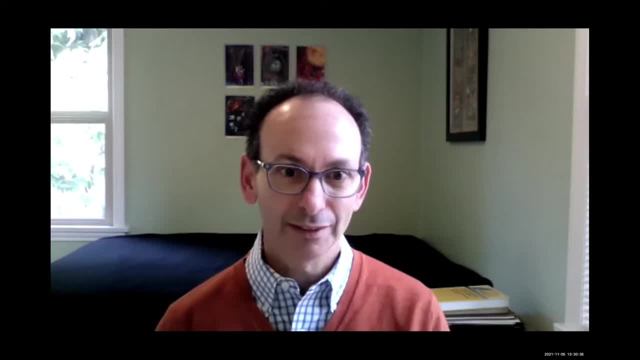 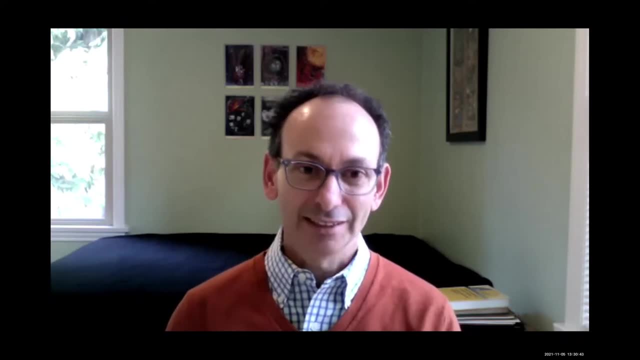 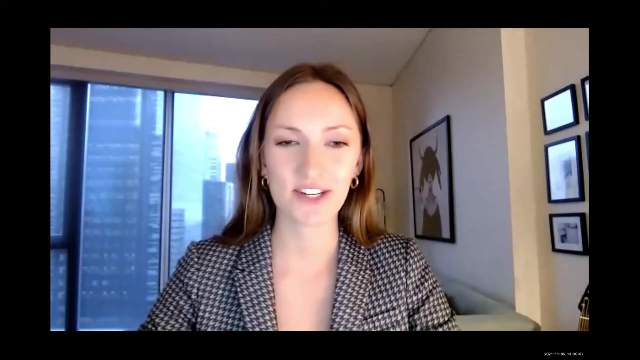 I'd like to turn over to Jess for an opening statement, I think in particular in the context of some of the challenges that you laid out for testing and just flying nuclear materials. So, Jess, would you like to make an opening statement? Thank you, Yuri and thank you, Roger. So, like Roger said, power for propulsion is a very broad 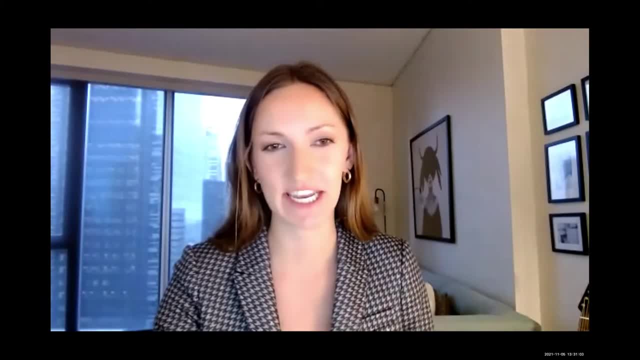 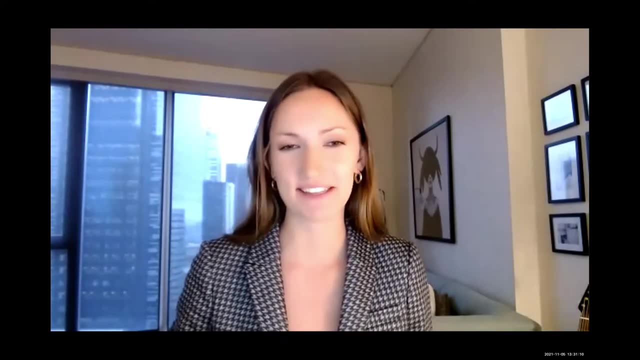 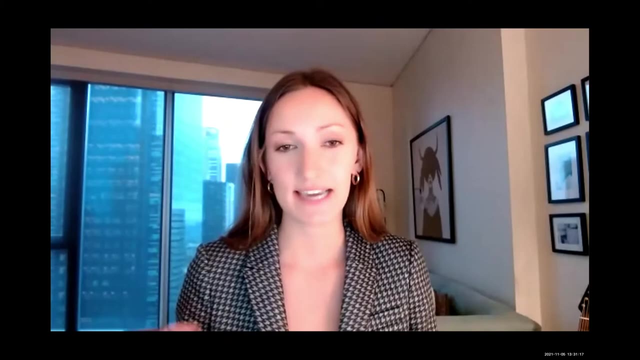 field and I'd like to take a closer look today at the use of nuclear thermal propulsion for deep space exploration, which Roger already correctly said comes with several risks. So the reason I'd like to look at this is because for propulsion, NASA is initially focused on 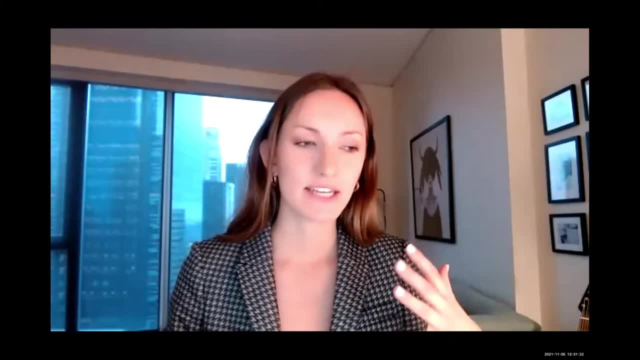 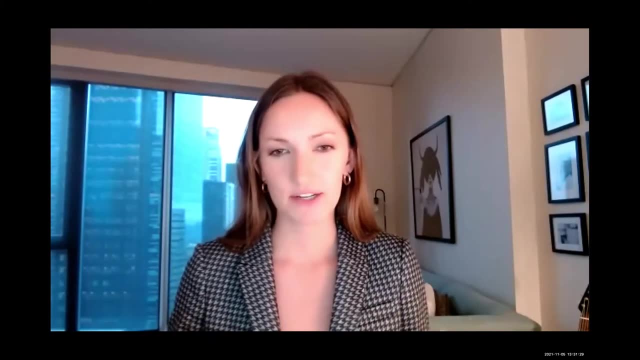 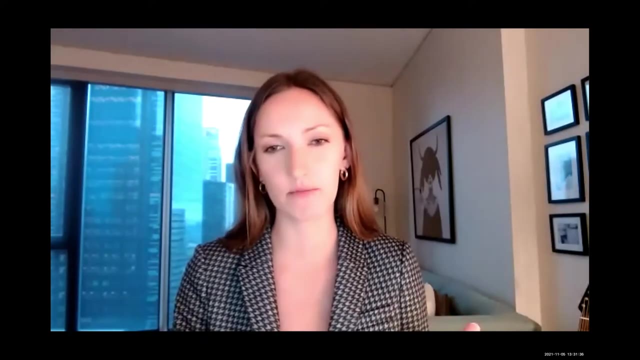 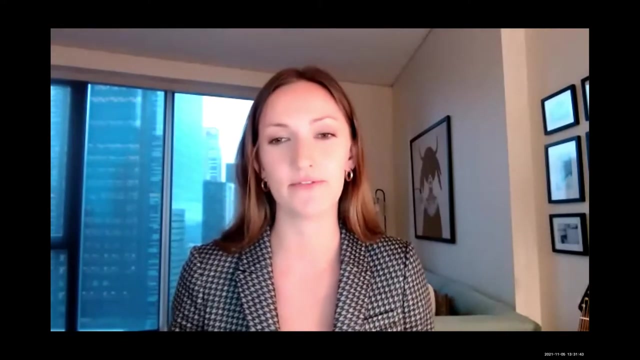 nuclear thermal systems and in this technology- so Roger already gave a brief summary- the heat generated by the reactor is transferred to burn hydrogen fuel in rocket engines, and so the thrust is similar to that of the conventional liquid fuel rockets we have today, but it has the potential to double the fuel. utilization efficiency, So that's why it's really attractive for use to getting us to Mars. So there are a few missions like these deep space missions which a lot of people believe we will need nuclear propulsion, for It's faster and more efficient and the Moon is only 400 kilometers away and Mars is 64 million. 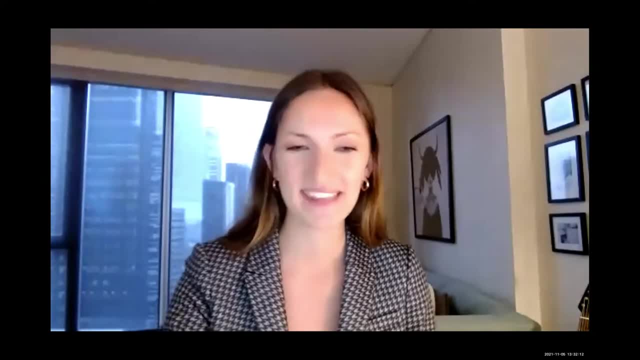 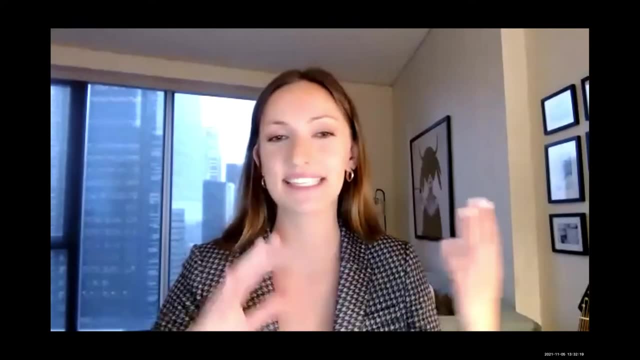 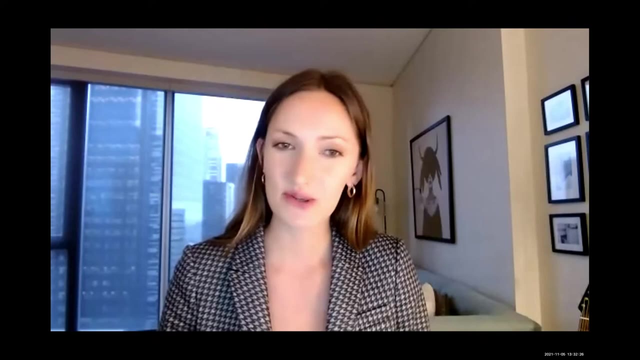 kilometers away, so we need to up our game a little bit. And then me at PNNL and personally, I've been thinking a lot about how these ambitious space activities, and especially our goal to get to Mars, are likely to increase the use and amounts of nuclear material in outer. 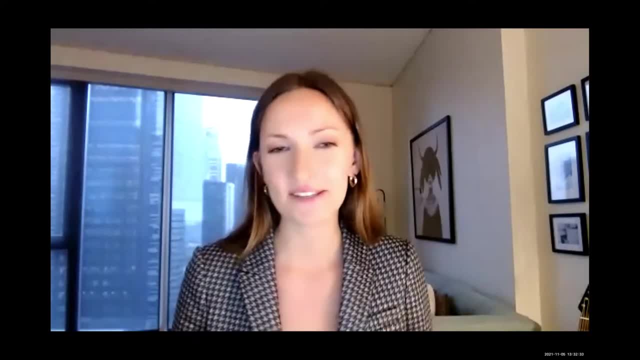 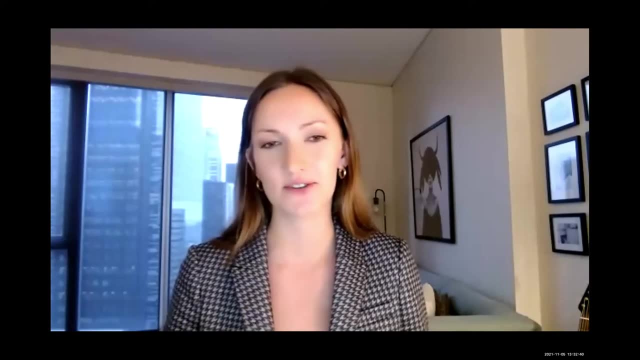 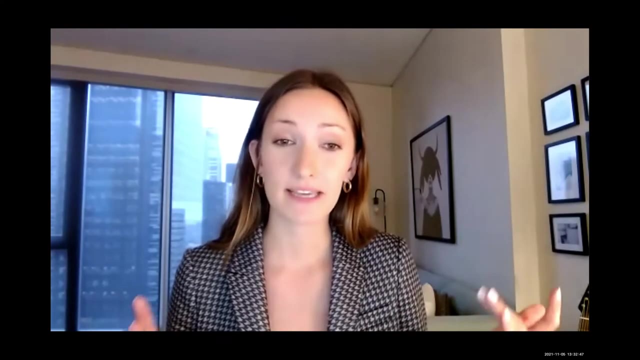 space. So I'd like to add a little bit of a policy perspective to start us off with today, And the main question I want to address is: how do we ensure peaceful and responsible use of nuclear power for space? What are the risks and how can we mitigate them now to really ensure we're going to 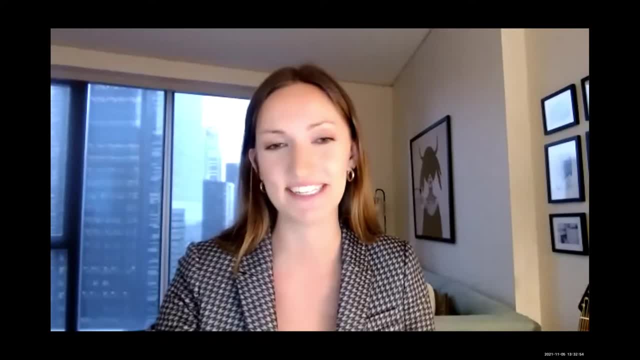 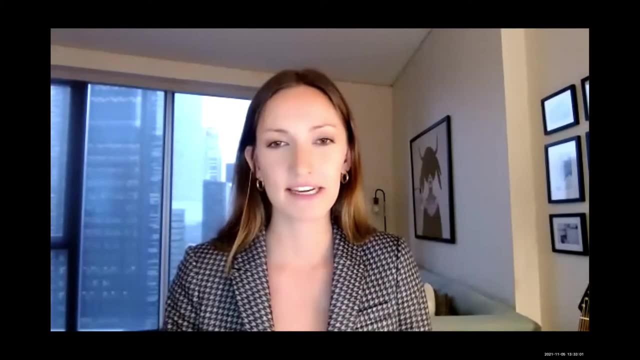 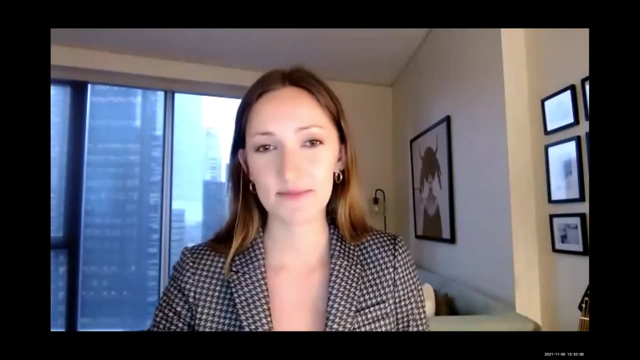 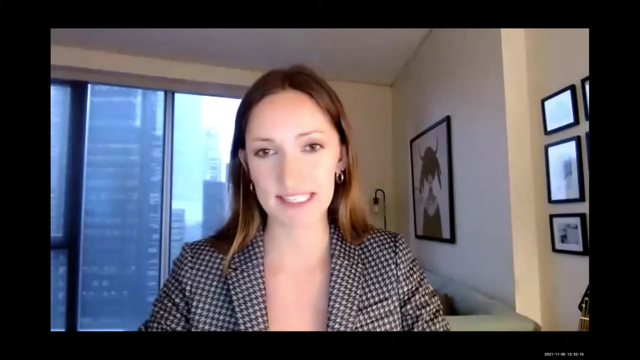 successfully pursue our space propulsion endeavors without any unintended consequences. So currently, only nuclear weapons states like the US and Russia are pursuing these nuclear propulsion systems, but we might as well, in the long term, see non-nuclear weapons state actors pursue these systems, And we also have increasingly commercial actors who are now actually 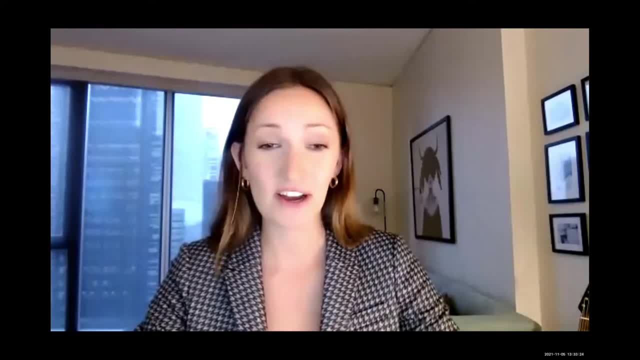 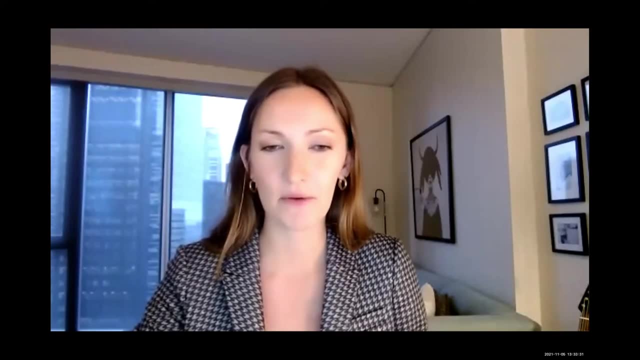 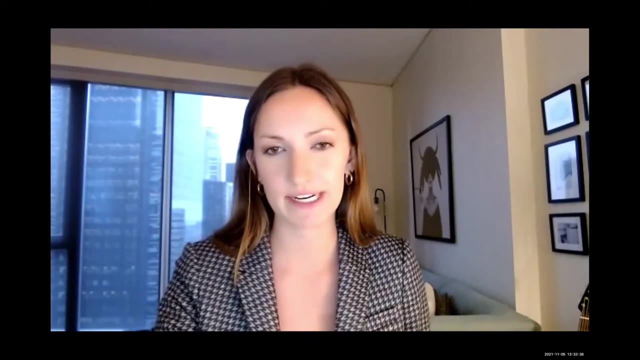 the majority of actors who launch into space, And so, with these new actors, I think we really need to talk about and think about what are the challenges that might be different to those we've had before and what are risks we should really be considering and mitigating at this point already. So 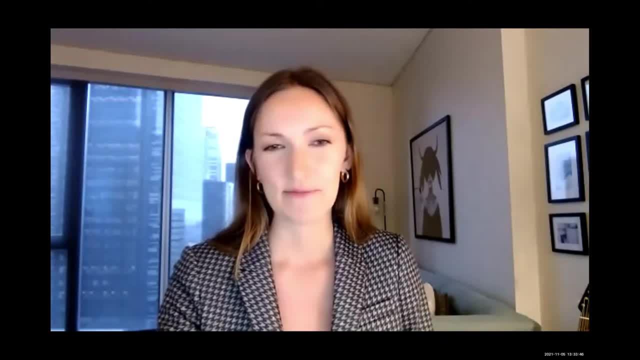 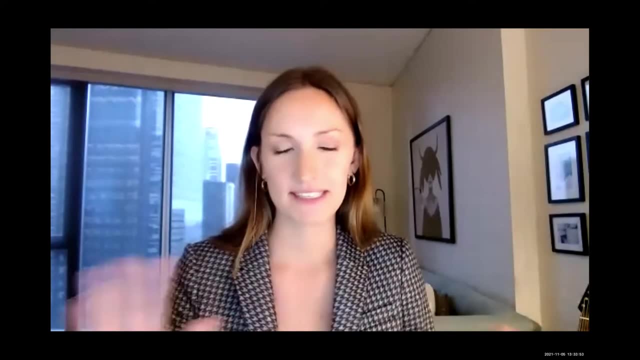 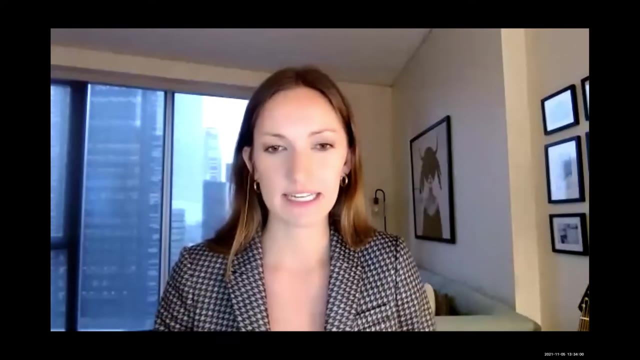 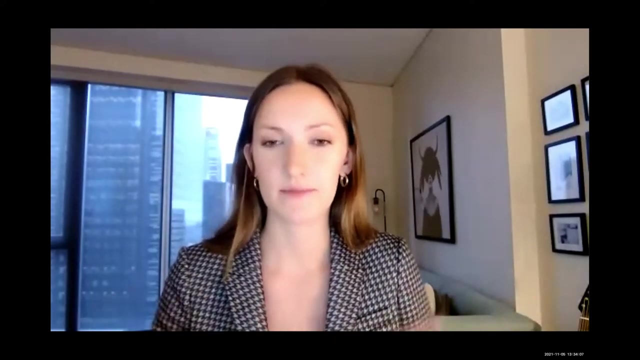 there are a couple of legal framework and policy questions. I want to briefly get your attention to Number one, obviously safety. Like we already said, launch failure is an issue, even though it might be not as big as compared to other types of propulsion, other types of nuclear stuff in the 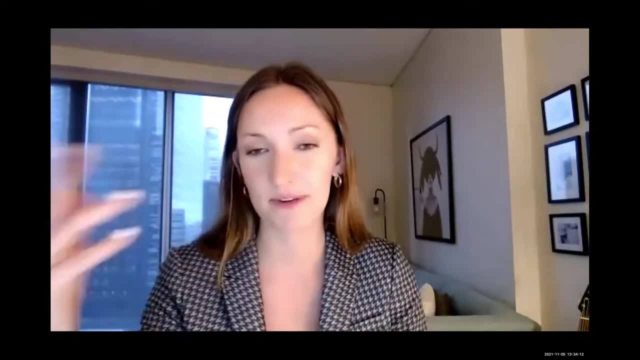 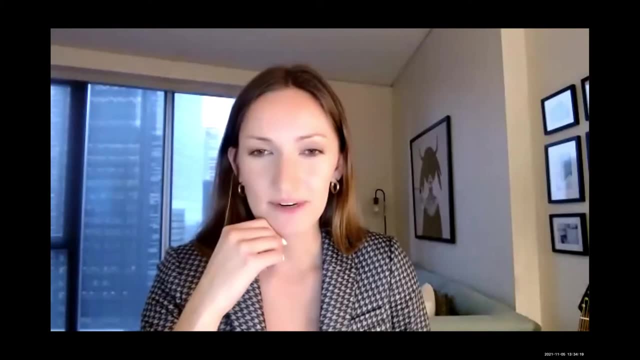 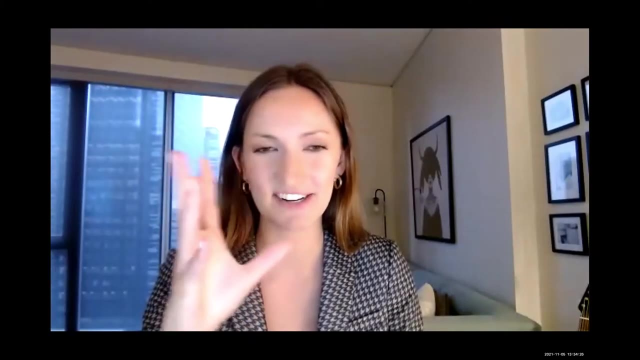 sky, But still we do want to consider what are the potential risks of using this type of fuel in a space reactor, And we do need to keep in mind that about 20% of launches, I believe, still have failures. So that's just something to start us off with the safety aspect. 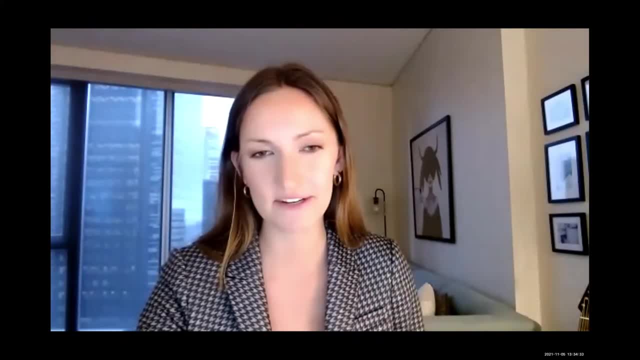 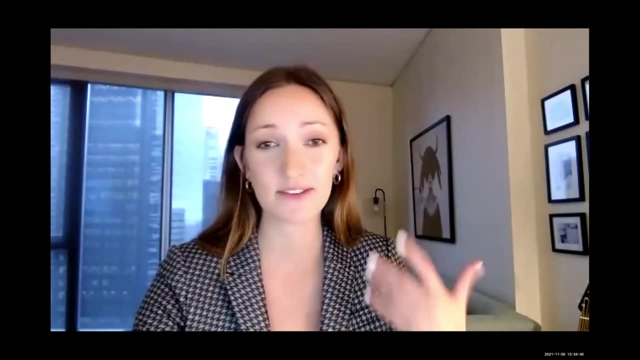 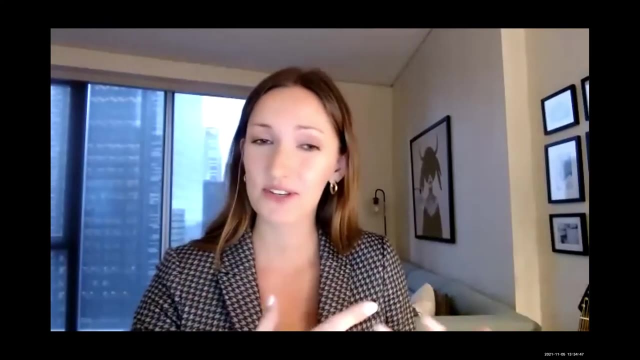 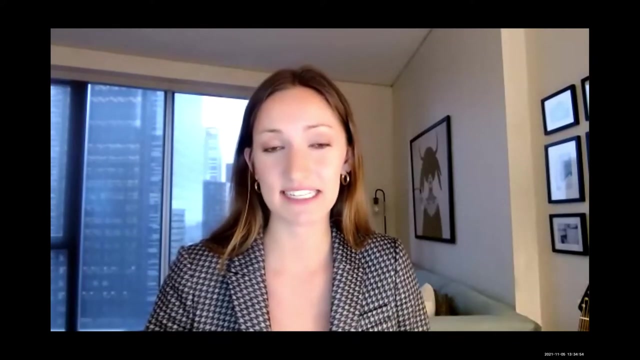 And then the security aspect, which I'm really passionate about. We have space reactors that pose two unique concerns. So first we have the incentive to actually use highly enriched uranium, because it is simply lighter, You need less of it, And so that saves you a lot of technical difficulties, And this might be. 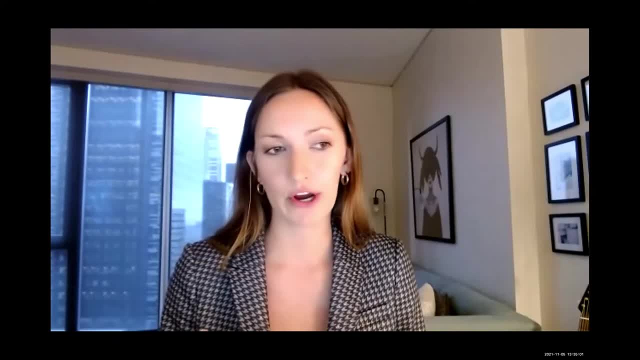 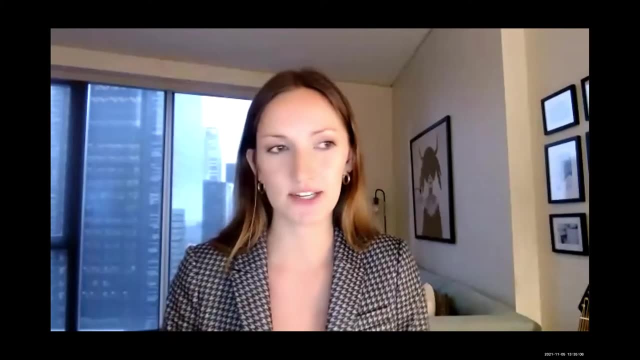 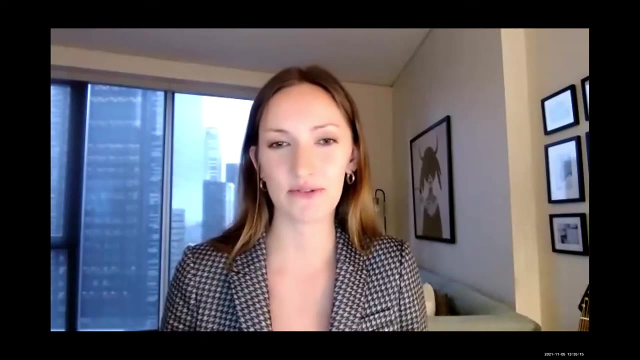 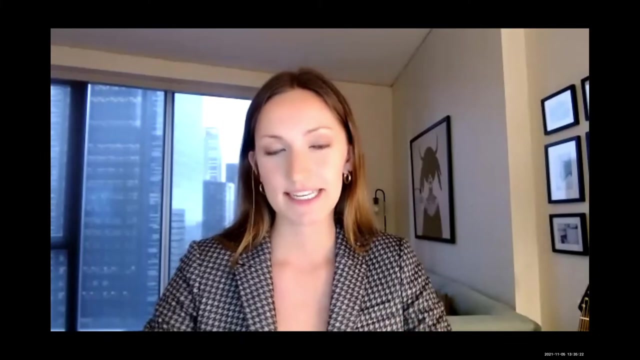 an option that more developing nations are interested in. Currently, the US government policy has been updated to focus on low, or at least high assay, low enriched uranium. But other countries who might not have as highly developed technological possibilities they might revert back to. 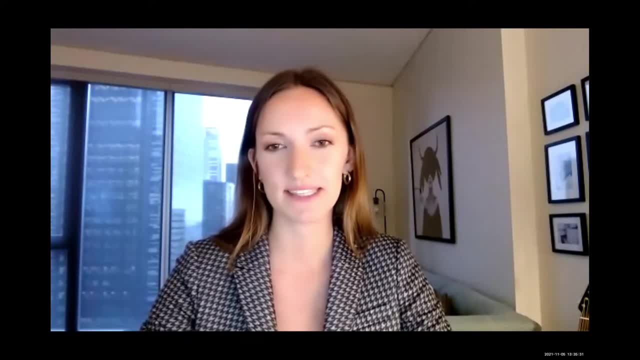 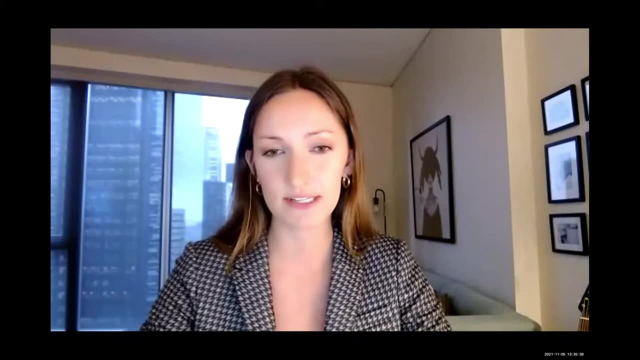 the use of highly enriched uranium and be interested in that, pursue that And that's really a big concern to me because that comes with a lot of safeguards and security concerns. Generally it's been the US policy in the past to really make sure we're using 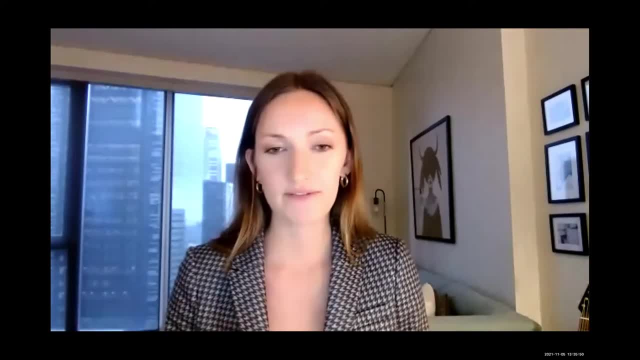 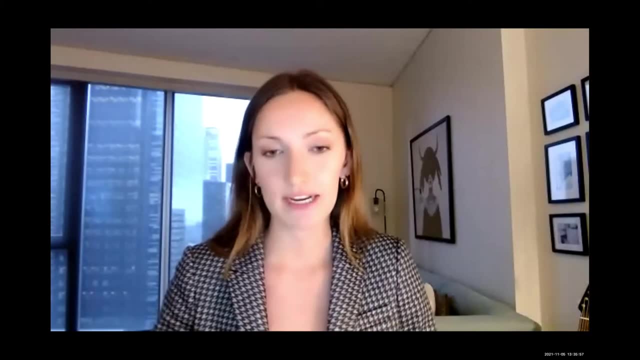 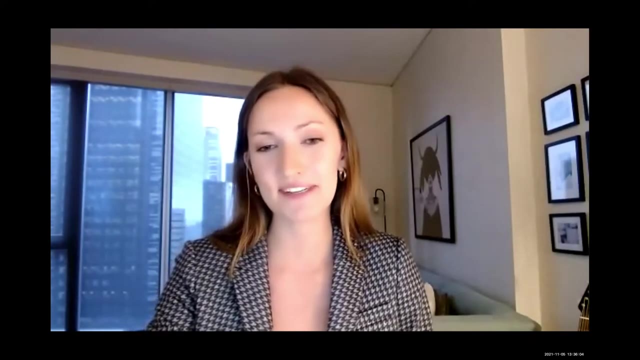 low enriched uranium in the world. get rid of that high enriched uranium which just poses too many issues because it has this potential of being diverted and used for nuclear weapons. So that's one big concern. And then the other point is that highly enriched 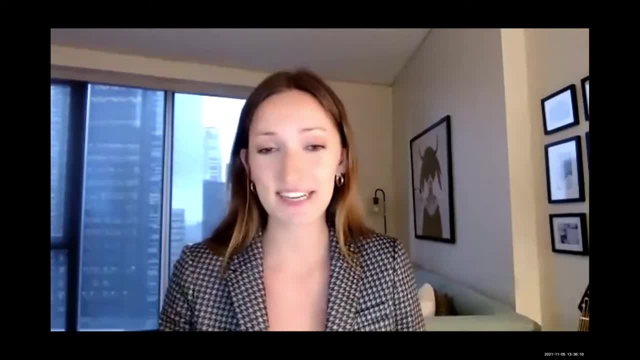 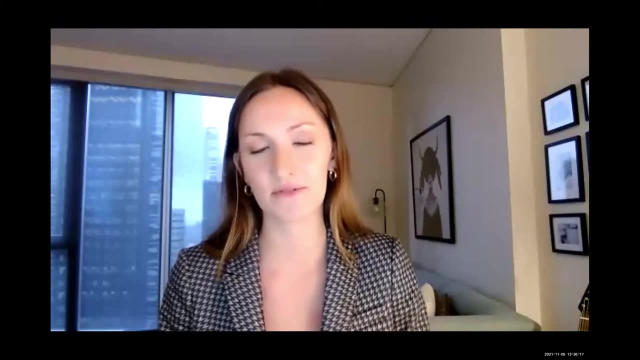 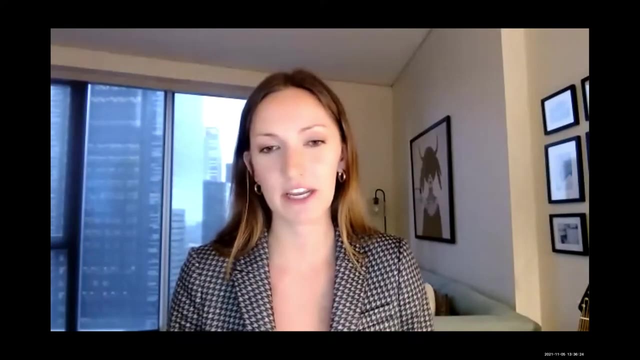 uranium does pose more costs because of these security concerns, It would be much more expensive to use it. So that's another reason why we're currently on the HALU track of using the more lower enriched uranium. And the other final reason for that is really the pushback from 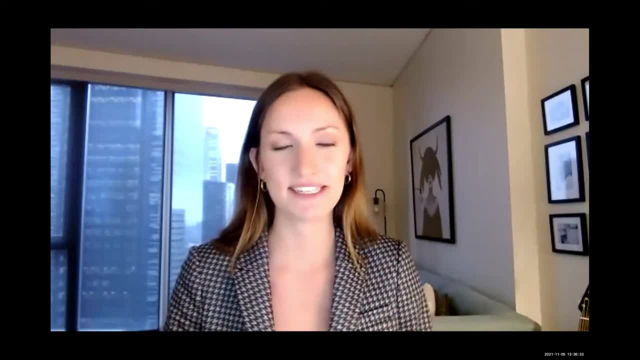 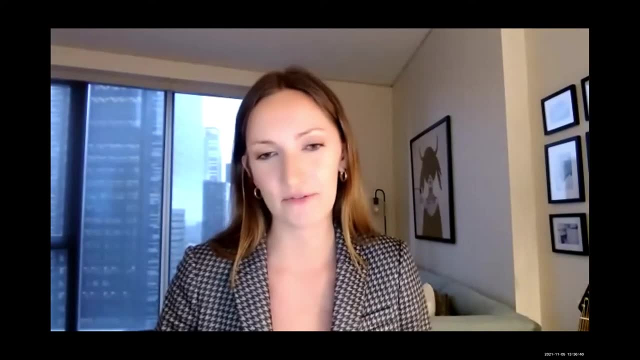 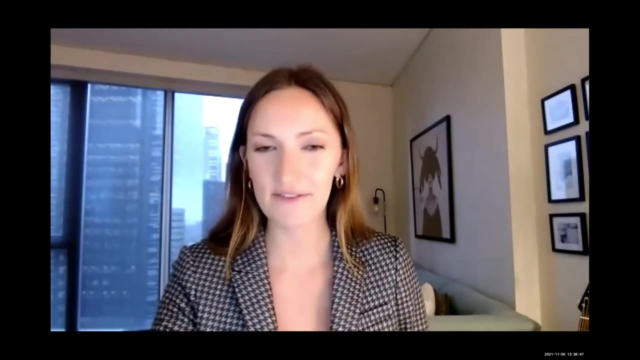 the public, which often doesn't distinguish between different levels of enrichment and different levels of risk, And we want to make sure we still have the political support for our ambitions. that might include nuclear power in space. So I know I only have five minutes. 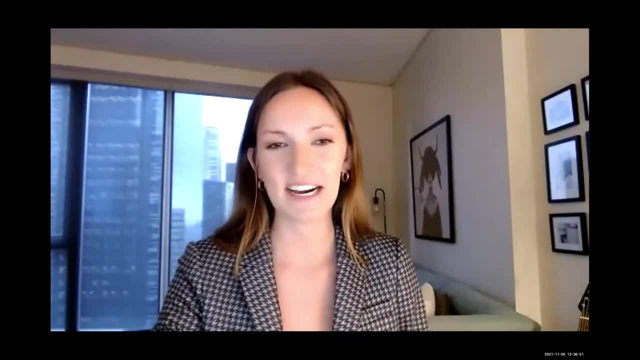 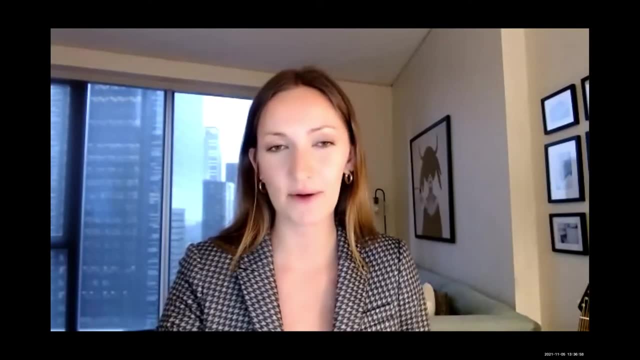 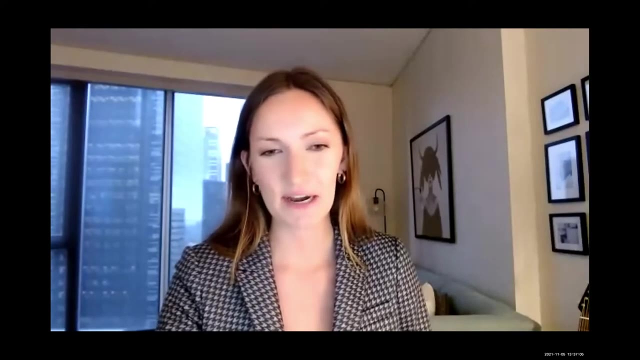 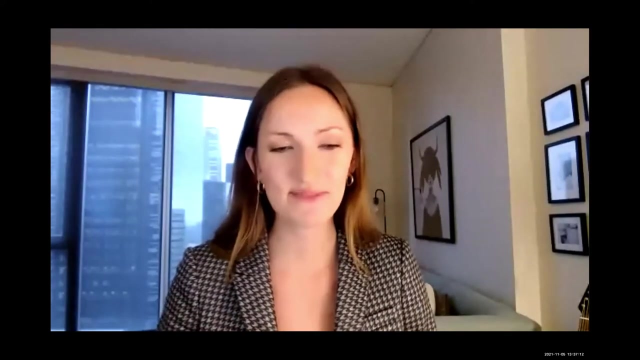 but I'm more than happy to expand more on the concerns and the difference between the two. I think there's a lot of potential for the commercial sector and the government sector to work together here to find solutions to mitigate these risks, And I'm really happy. 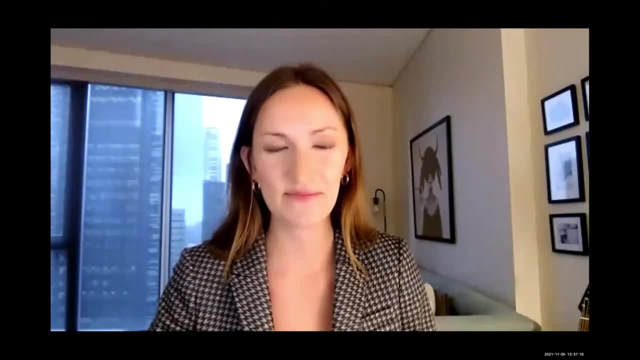 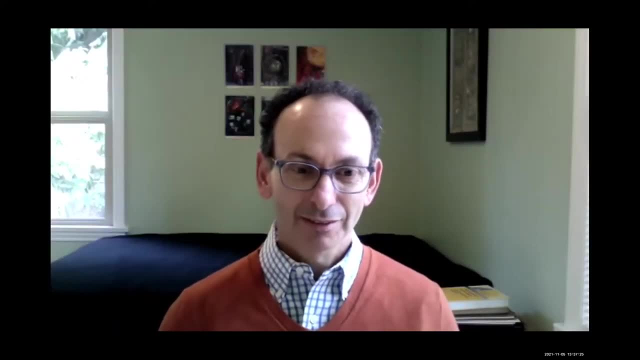 to talk about it more and also hear your ideas of the other panelists. So thank you very much. Great. Thank you, Jess. Very interesting. So now I think it's going to flow quite nicely if, Jeff, if you give your opening statement with. 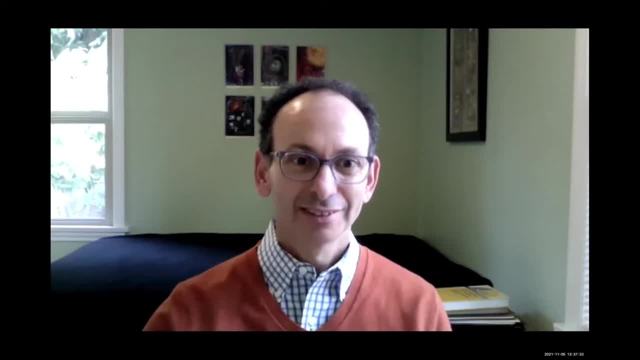 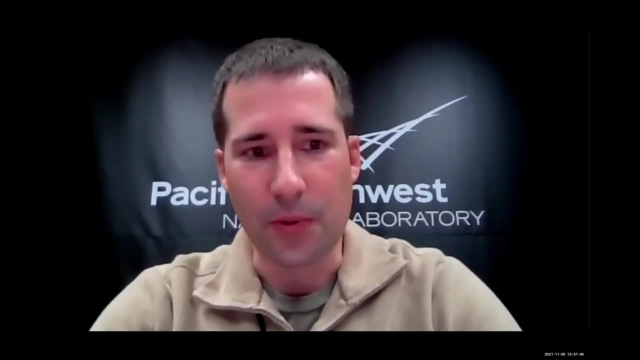 your expertise in nuclear systems. So go ahead, please. Yeah, sure, Yuri. You know I really got my start in space nuclear about 14 years ago through the Center for Space Nuclear Research at the Idaho National Laboratory, And you'll probably run into a number of people my age, maybe a little bit younger, who have a similar story. 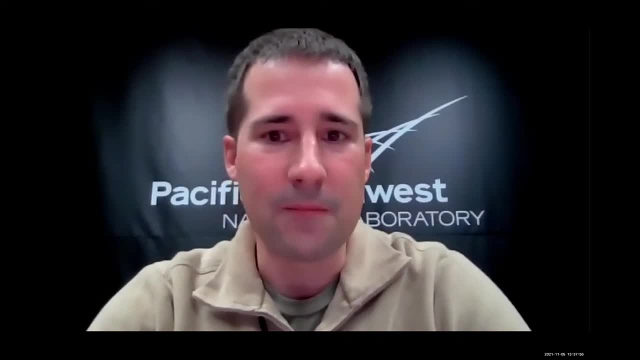 But there I started out looking at plutonium 238 production, radioized to power systems and high temperature energy conversion systems, And that eventually led me to do my PhD and my postdoc research looking at ways to process plutonium 238 in a way that decreases the hazards that are. 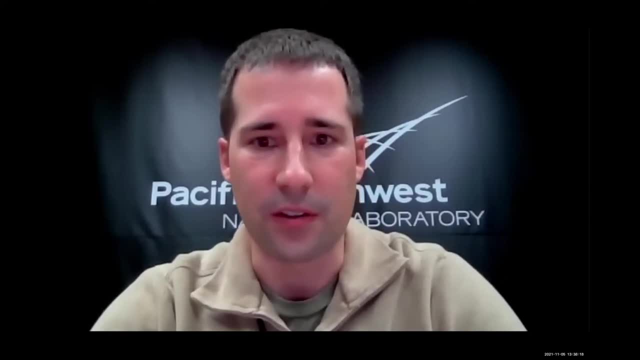 associated with that process, particularly the stage that occurs at Los Alamos. But I'm also very interested in space reaction And I think that's a really great question. I think that's a really good question, And I think that's a really good question. So I've came up with a great question about space reaction to be able to do that- and I think that's one of the things about space reaction: to be able to do that- and I think that's a really good question. But I'd like to know a little bit more about that, because with that I have to talk about the question that. we have all of a sudden. So I'll start with you and then I'll take it up to you. Sure, So I'm going to go ahead and share with you the last few minutes And then I'll go ahead and start the question that the panelists have also asked, And I also have a question. 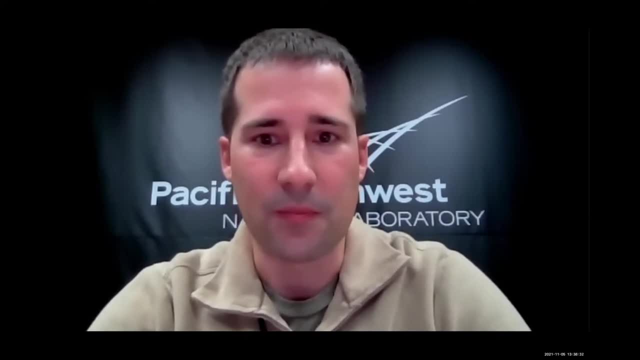 from one of our listeners who are a little bit more familiar with the topic, but which okay and they're very interested in doing, And I think I can answer that first. So let me give you the first question, a little bit more specialized on nuclear thermal propulsion. I thought maybe I'd speak a little bit. 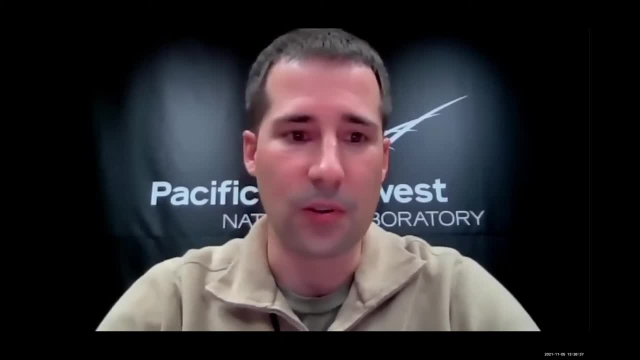 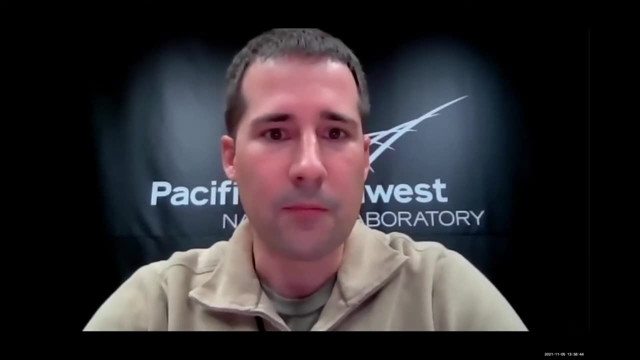 more about space reactors and nuclear electric propulsion today, So I did want to mention a little bit about RTGs just to start. Some of you may be familiar with radioisotope thermoelectric generators which the US has used to enable our space exploration missions. and regimes where the solar power just isn't strong enough. The RTGs, like Roger mentioned, produce on the order of tens or hundreds of watts electric to power spacecraft, with maybe the exception of the 1960s TRW poodle thrusters. that was the little. 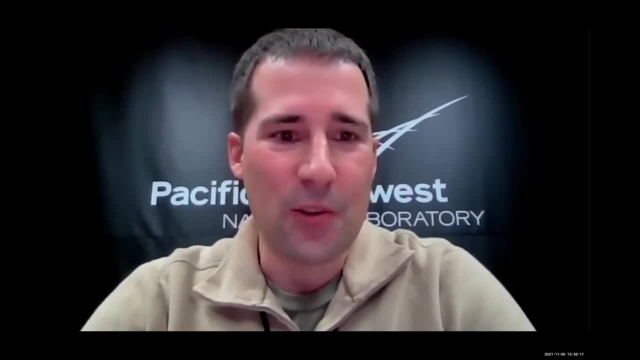 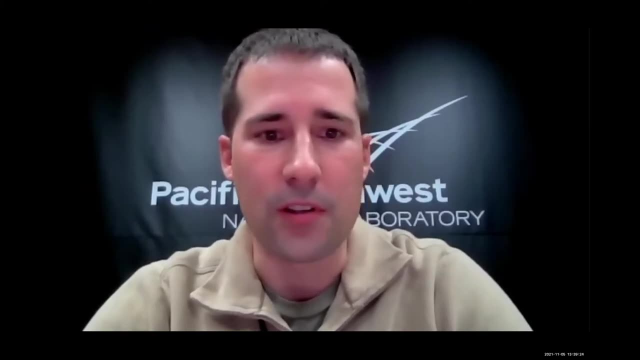 brother to the rover engine. Radioisotopes really aren't used for propulsion systems. Our exploration missions like Voyager and Cassini and New Horizons didn't use their RTGs to power electric thrusters, but rather their onboard electronics and sensors. These missions used 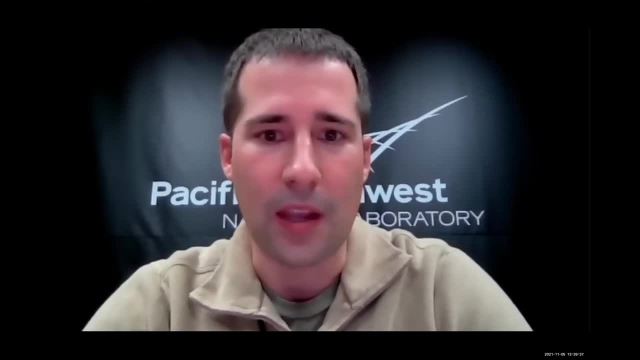 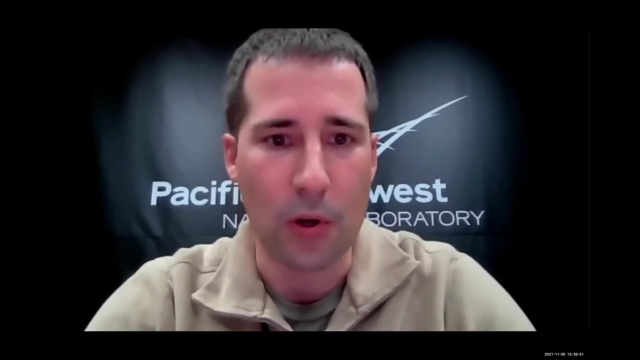 their initial launch vehicle energy and orbital mechanics maneuvers to accelerate them on their trajectories, and then use chemical propulsion systems, mainly in the form of hydrazine thrusters, to fine-tune their path and to orient their sensors where they wanted to point. 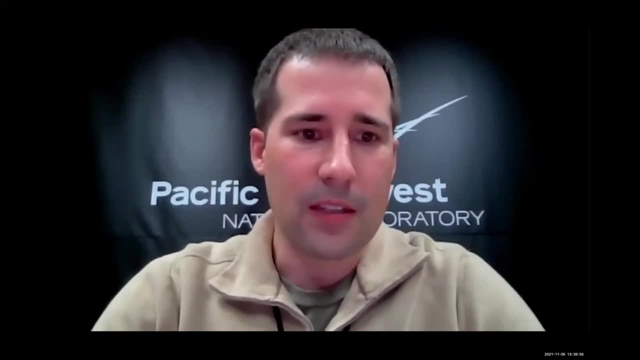 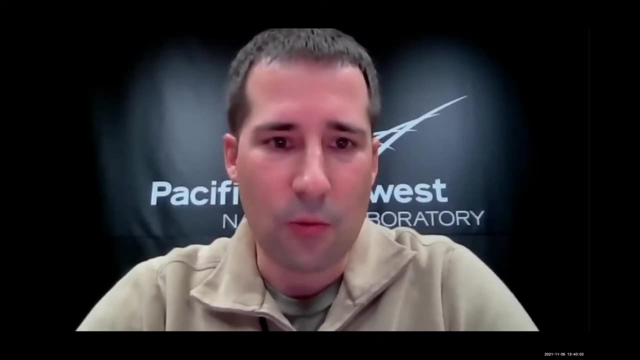 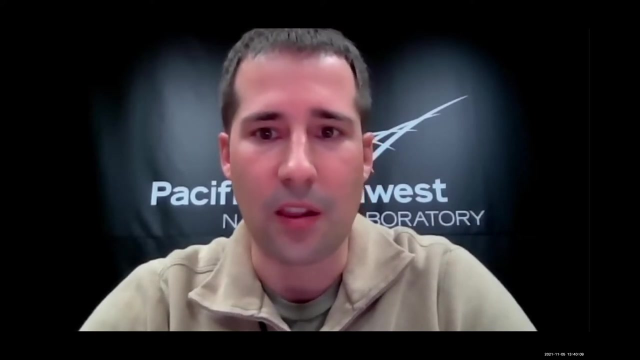 In the context of nuclear electric propulsion or NEP. I think that there's a lot of potential in the coming years. Like Roger mentioned, most of the electric thrusters today are in the neighborhood of five kilowatts electric, with some of them up to 10 kilowatts electric deployed in orbit. 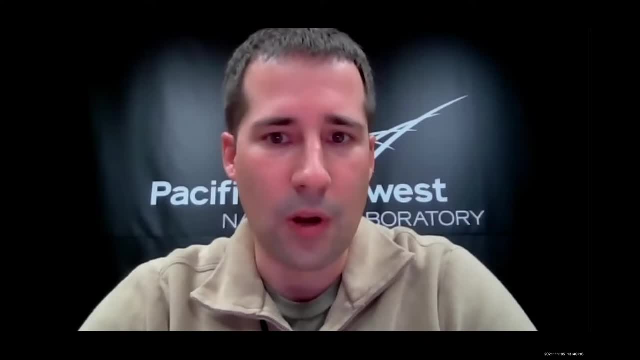 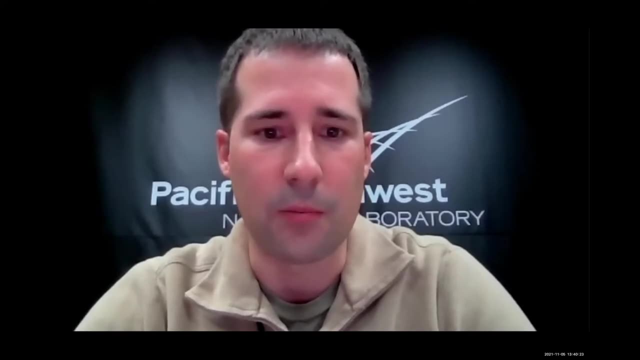 And higher power thrusters is not really a problem, but really, where you see them being limited to five to ten kilowatts is mostly based on the amount of energy that they produce. They're based on the power that's available on the spacecraft today rather than the the potential of the electric thrusters. 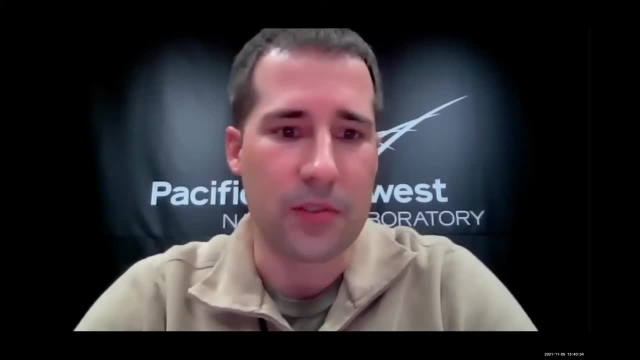 So these higher power thrusters, like the 100 kilowatt versions that Roger mentioned, are in development. they could be used, but really they they need a power source. So in the nuclear electric concept the reactor is coupled to an energy conversion system with. rejection and then powers those electric thrusters, with the main benefit being that you can get very high specific impulse. So a chemical rocket specific impulse may be on the order of, you know, 400, 425 seconds, while with nuclear, thermal rockets you may get somewhere around. 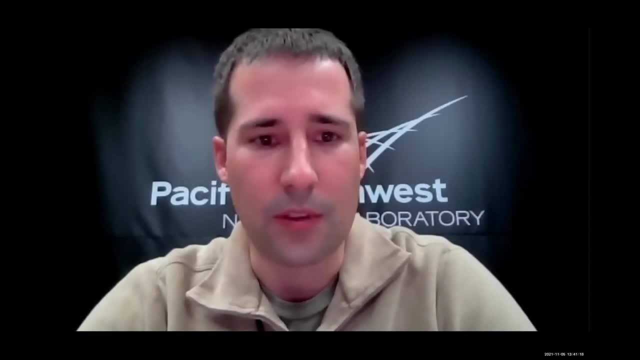 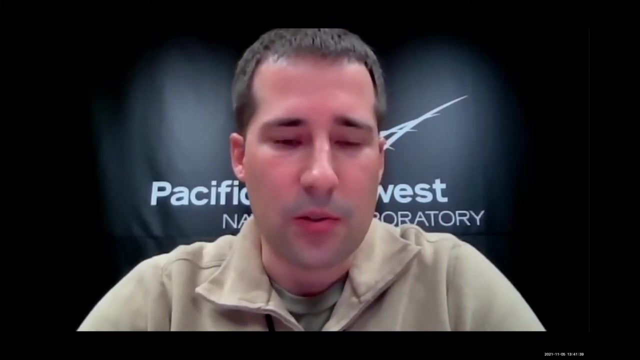 800 to a thousand seconds. With ion thrusters you can get well over a thousand or even thousands of seconds of isp, depending on the devices, which makes these sort of the ultimate in the space fuel economy for propulsion. So the issue is that to date, only a handful of space reactors have been deployed. and all of their power levels were below 10 kilowatts electric. These prior systems were built and flown in the 1960s, Cs through the 80s, but today there's renewed momentum to deploy space reactors with power levels of 10 kilowatts and higher. In the US, the commercial sector is developing space reactor. designs for applications such as a lunar base, and I've seen news articles about Russian work on space reactor. So we may see space reactors being deployed this decade. but there are a lot of associated challenges, especially for power levels of hundreds of kilowatts electric or more. 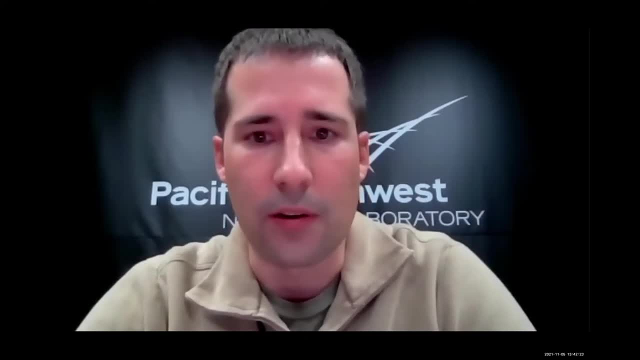 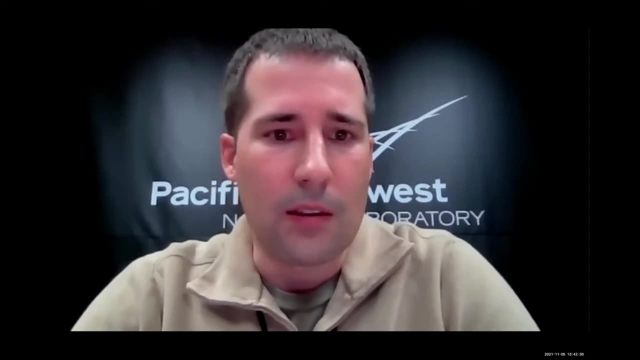 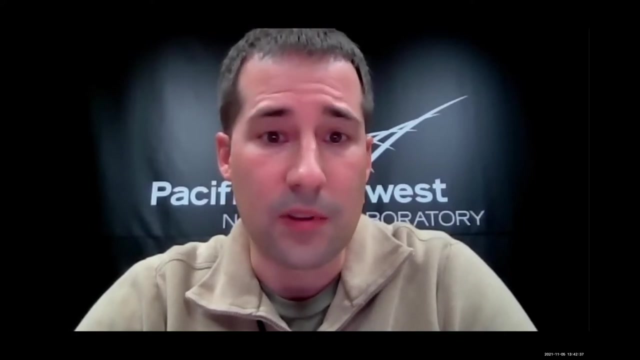 where the dynamic power conversion technologies are required and they have to operate reliably for years without maintenance, which is a real challenge in space. And if we deploy space reactors using HALU fuel, there are going to be some additional technologies that are needed to be advanced to make them mass competitive with the HEU systems like Jessica alluded to. 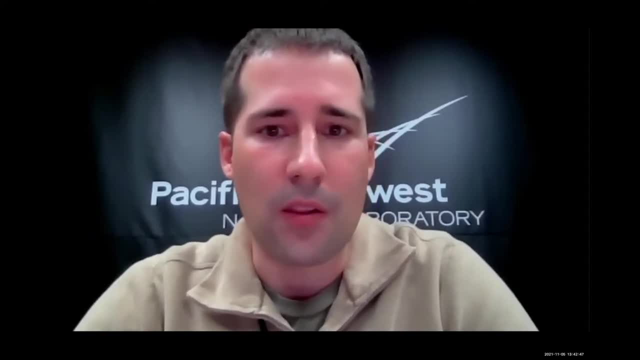 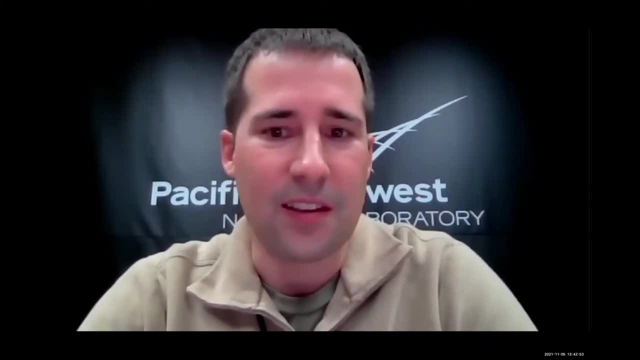 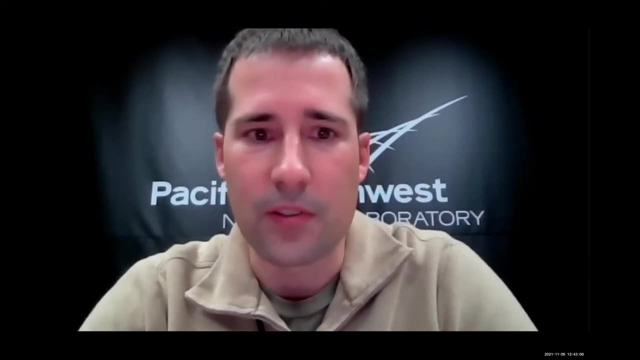 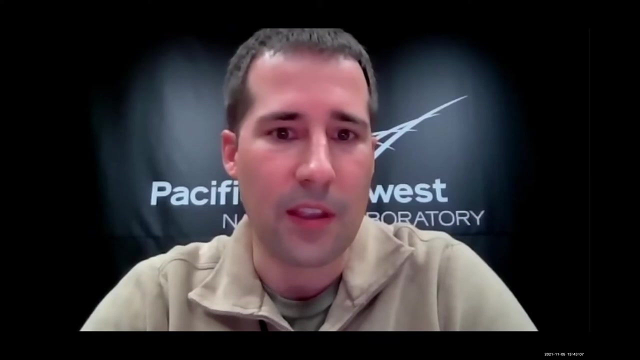 power, which I'm sure Jessica will discuss more if she has a chance. which is exciting to see, And although the president's budget proposal eliminates funding for vision-based space propulsion, I saw that both the House and the Senate proposed to continue funding it and that the House appropriators directed NASA to allocate. 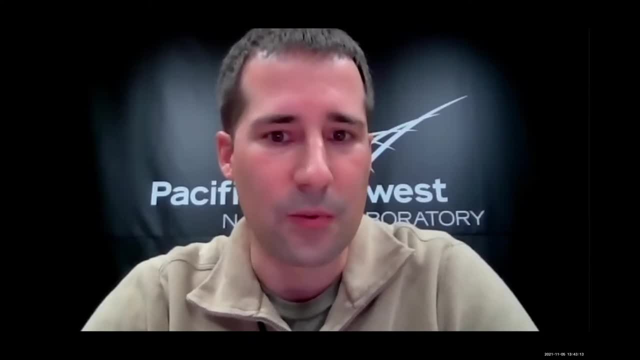 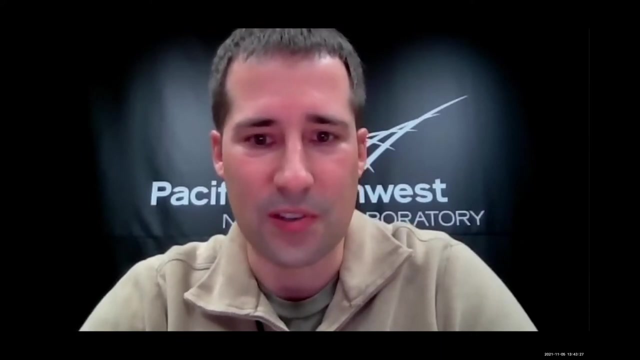 at least 10 million for nuclear electric propulsion based on the recent National Academy's report that Roger led. So we may see some new NEP efforts directed at a Mars mission. So I think this is a very exciting time for space nuclear and look forward to the rest of the presentations in the panel and the discussion. Thank you, 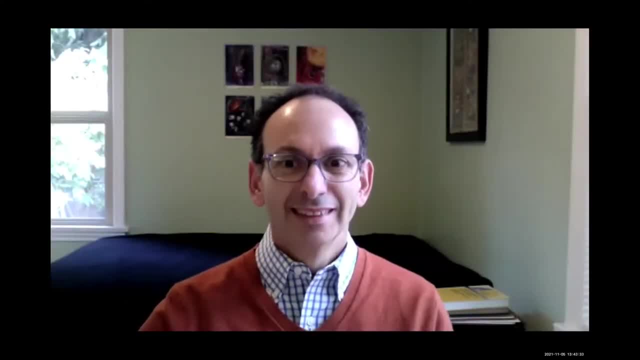 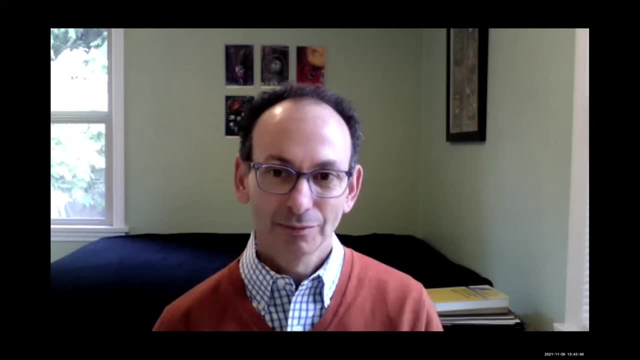 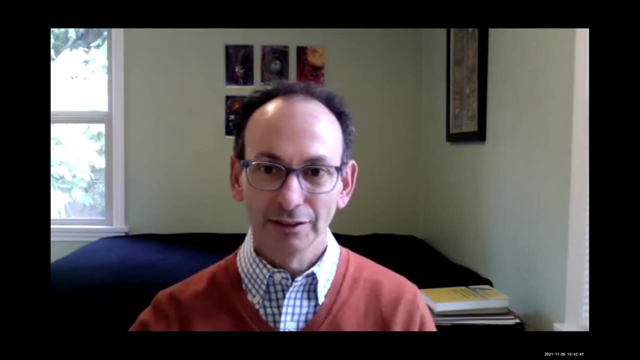 Thank you, Jeff. So yeah, I think that flows nicely into some of the work that Jake's been been doing with the nuclear thermal and perhaps even applications for fusion and how hydrogen fits into both of those locations. So, Jake, would you like to give an opening statement? 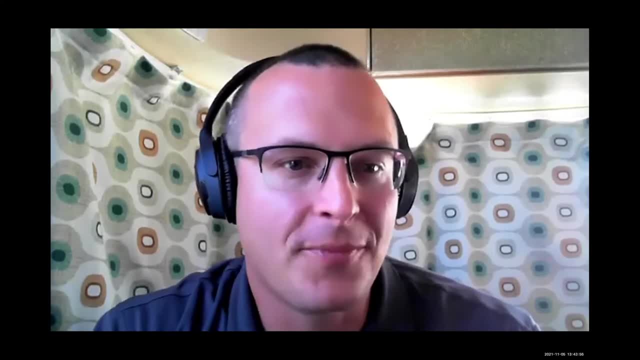 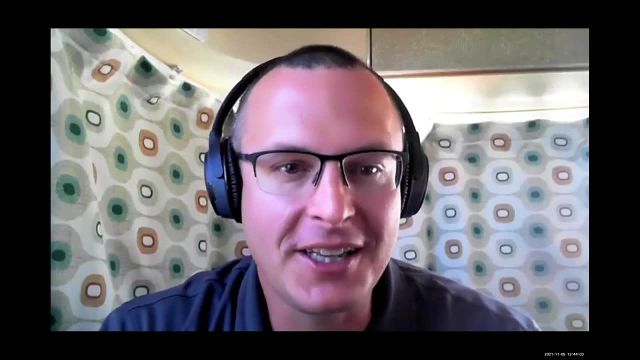 Sure, thank you, Yuri. I prepared slides, but in the interest of time, I'm just gonna make it real succinct and try to get the message across real easily. I mean, when you look at the universe, you look up at the stars, okay, 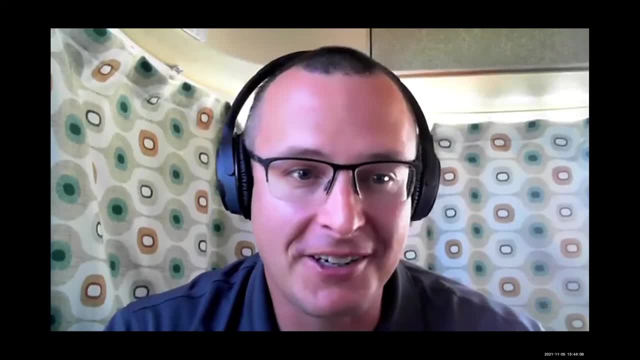 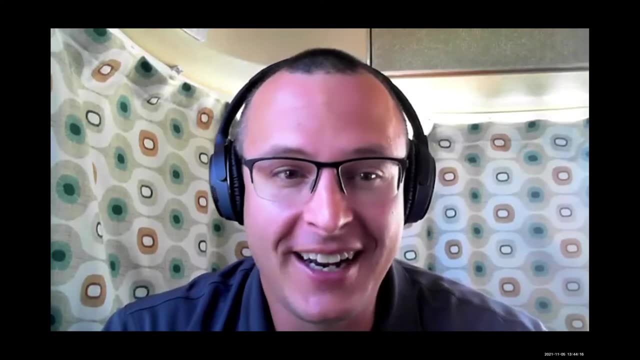 you're seeing light from burning hydrogen. It's 74% hydrogen by mass. If you think about hydrogen by number in the universe, I mean it's far, far greater than that. So, and even here on Earth, all chemical reactions. 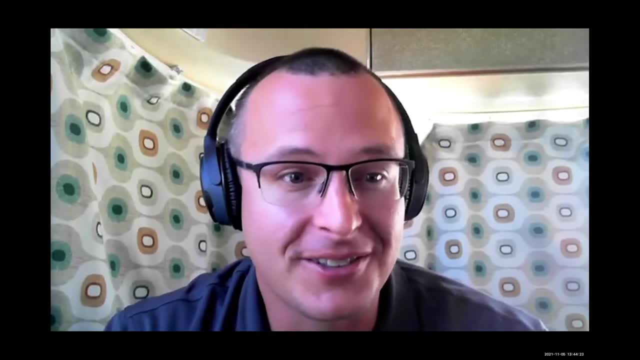 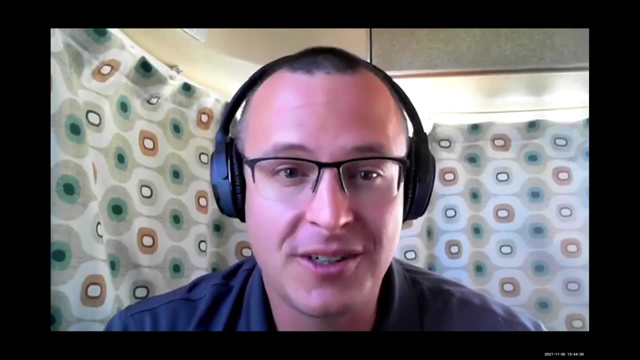 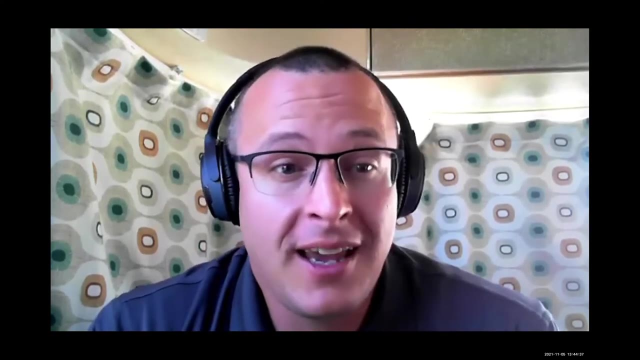 it's pondus, hydrogeni pH, the hydrogen potential that drives them. So I really think the logistical challenge, the storage and distribution of hydrogen, that's the biggest opportunity for space or clean energy here on Earth in space- Okay, whether you're running a chemical rocket, a nuclear fission rocket, a fusion rocket, or if you just wanna have a good, moderate-sized rocket, or if you just wanna have a good, moderate-sized rocket to keep from the space radiation. liquid hydrogen is where you wanna be. 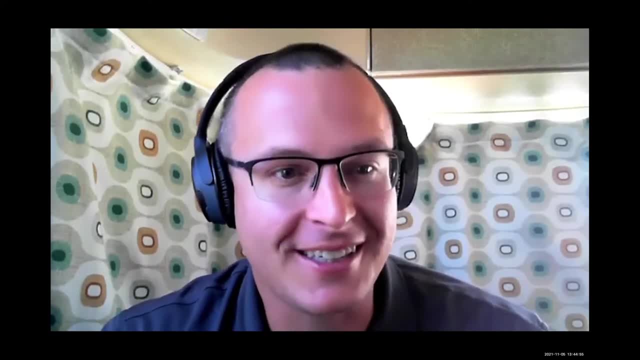 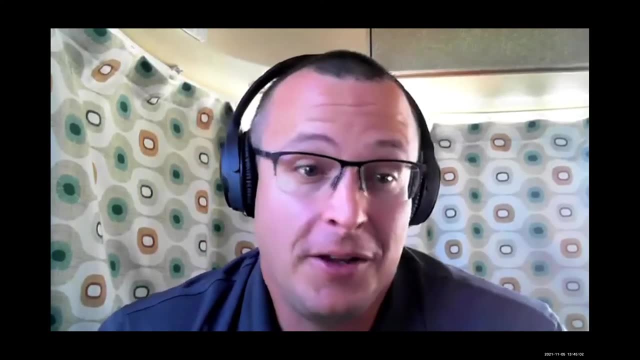 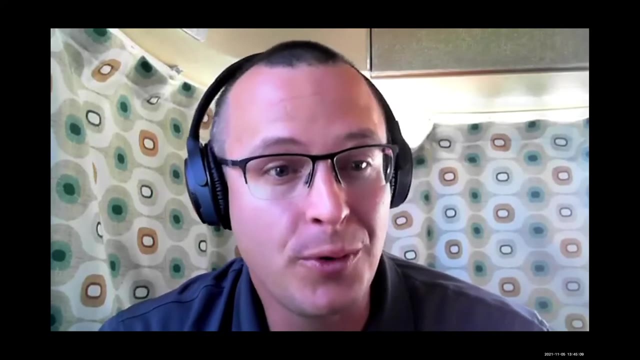 but it's always been the logistics that have prevented us from using it as a fuel, The SR-71, originally designed to fly on hydrogen. Hydrogen burns better in a turbine, but we could not get liquefiers distributed around the world. to everywhere, we would need to refuel the SR-71.. 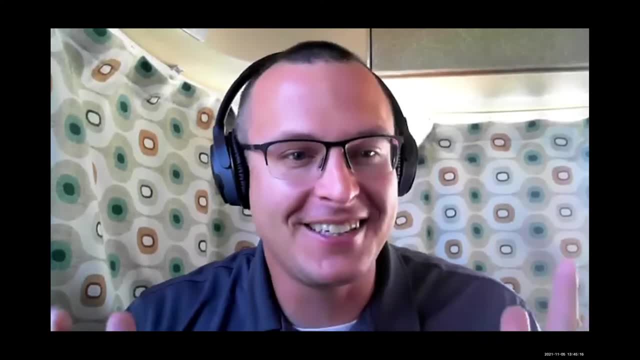 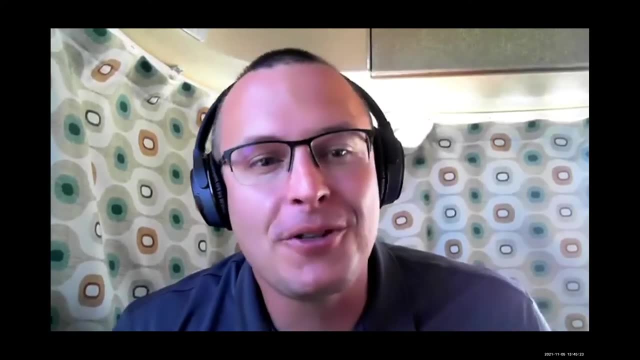 And so I get really frustrated today when I hear these challenges of we're gonna try to produce hydrogen for a buck a kilogram by the end of the next decade. We've always been able to produce massive amounts of hydrogen. It's always been our ability to store and distribute it. 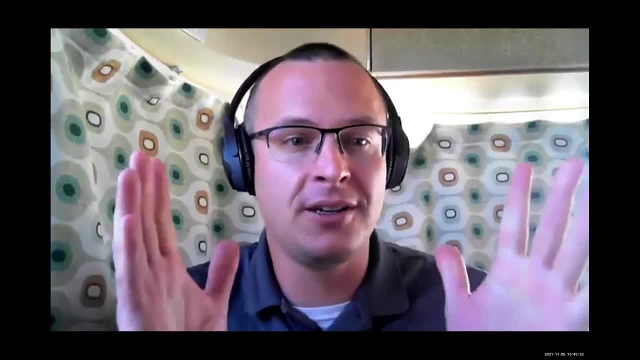 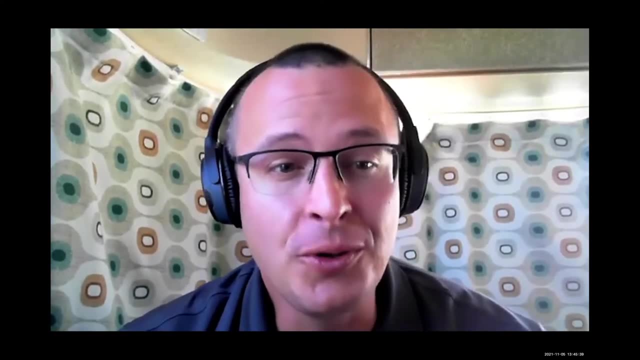 that's the issue. If you look, if you had $100 million put it down on the table today to say I want the best hydrogen liquefier money could buy, You would get a system. basically that's 1970s technology. 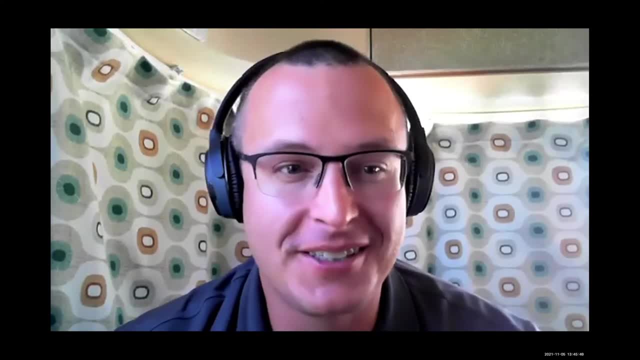 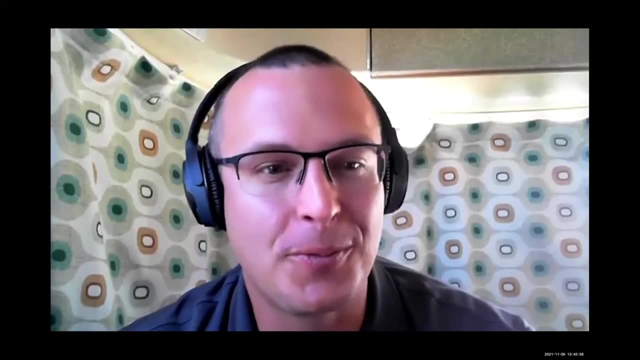 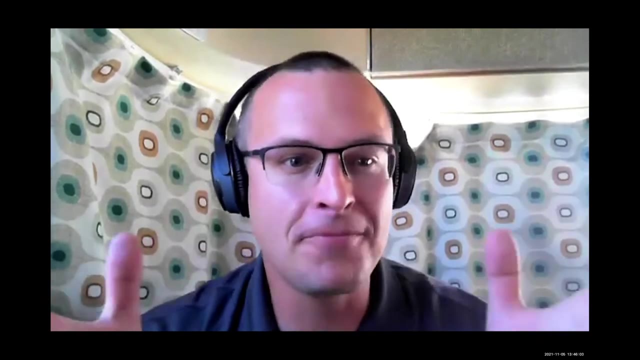 that is operating less than 30% of what is theoretically achievable, okay. And moreover, it can't scale down to be something useful for space rockets- okay. And you think about how many areas this impacts and that we haven't had a research program in this area? 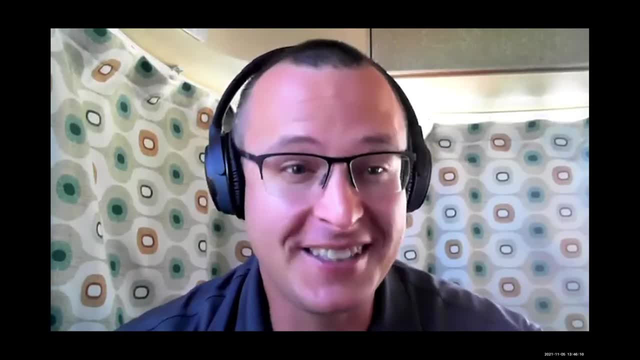 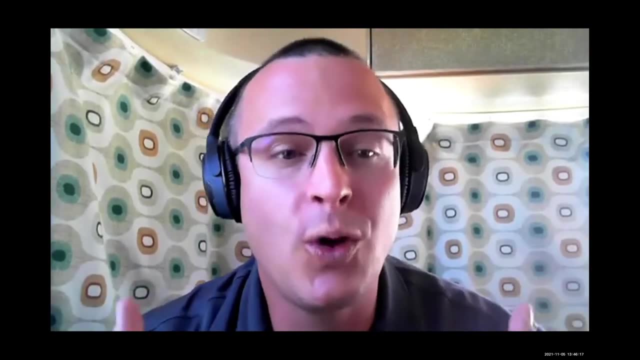 in the US for 30 years, 40 years, You can see why we're running into all of these issues and challenges. we can't figure out. So, anyhow, what we do and what we're doing about it in my lab right now, we're really focused on two things. 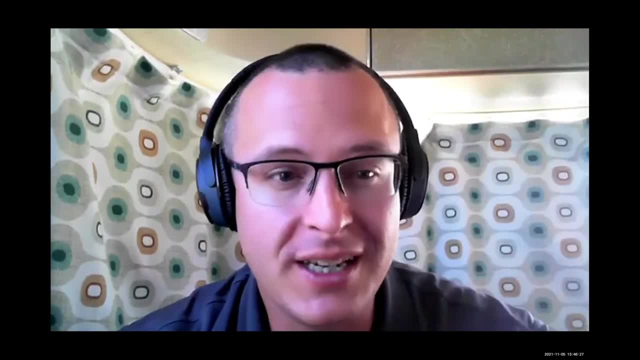 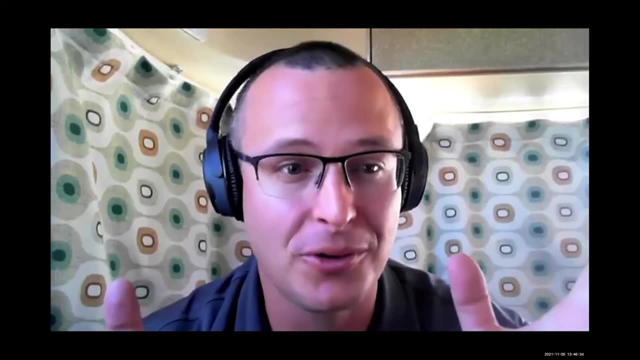 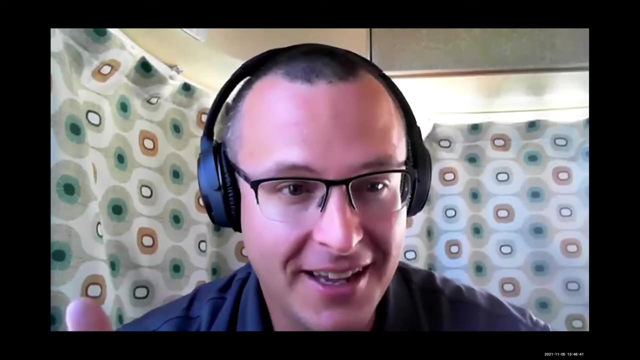 Efficient, scalable hydrogen liquefaction. We just completed the build of the first deployable hydrogen liquefier that you can drop on a beach front anywhere in the world. you want to plug in electricity and water. you have liquid hydrogen. We're looking at scaling that up. 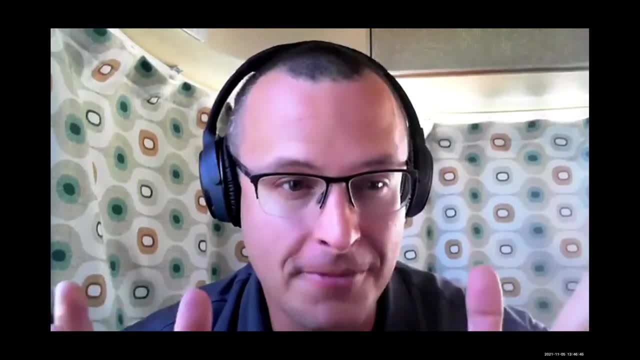 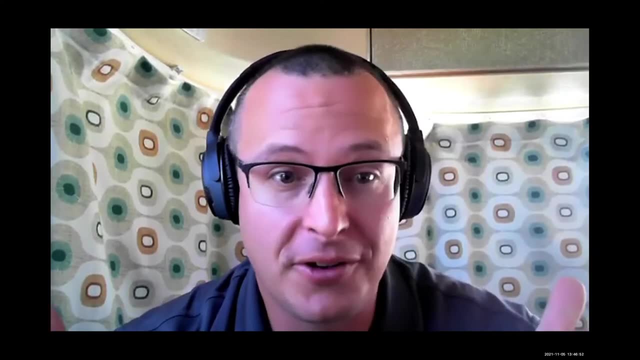 developing much more efficient hydrogen liquefier concepts. We have two that we're trying to find anybody to fund because there isn't a program we can go to at the federal level that's set up to fund this kind of thing- The one that was trying to get set up. 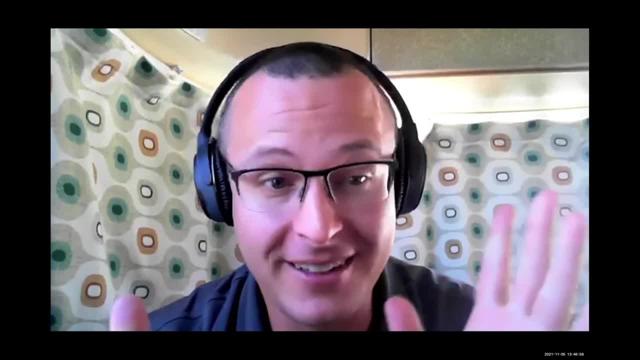 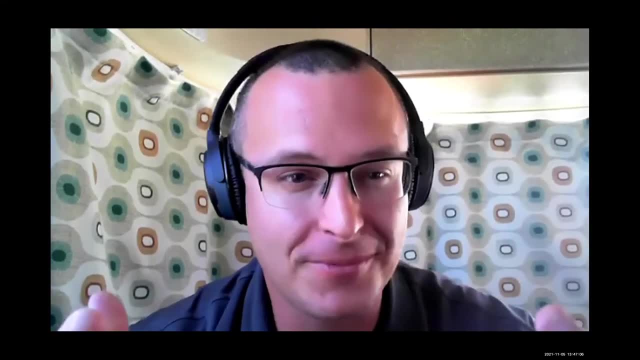 can't get interest at the federal level, But anyhow we're making those. We're also looking at liquid hydrogen storage. So changing the paradigms. If you put liquid hydrogen in space, it's not gonna settle to the bottom of a tank on its own. It's gonna be all over the place. You're gonna have heat leak, thermal soak from your nuclear hydrogen rocket motor burning in the back. it's heating up your tank. It's gonna boil. you're gonna have to vent a lot of it. When the Saturn V folks wanted to go to the moon, they had just a few hours to decide to make the jump to the moon because the boil off rate in their tanks was so high that if they waited they wouldn't have the fuel to make it there. Today it's the same problem. It's almost the exact same liquid hydrogen storage configuration going in the SLS. Technology has changed. We can make things so much differently than we have in the past, Yet still we're trying to fly liquid hydrogen storage concepts. 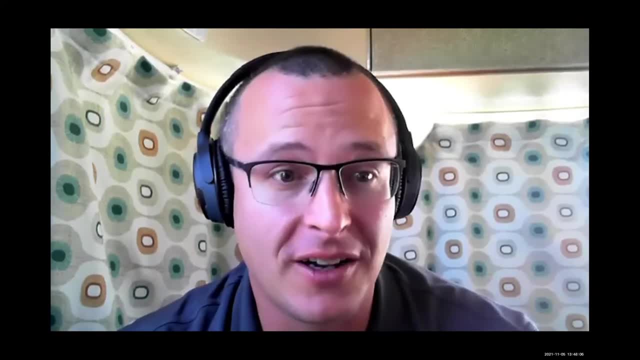 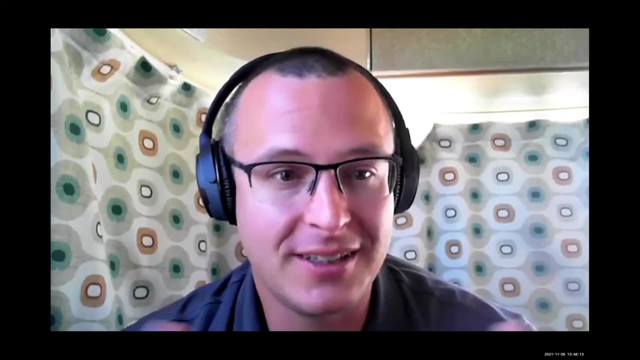 that were pioneered in the 1980s, just to test them, that have been on the backlog for that long. So this is where we're coming in: in the lab We're developing 3D printed liquid hydrogen tanks. We did that for drones. 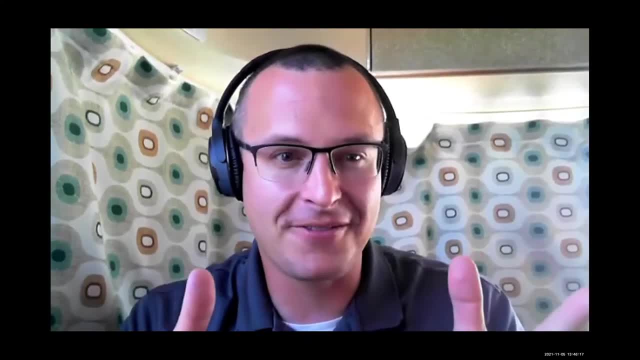 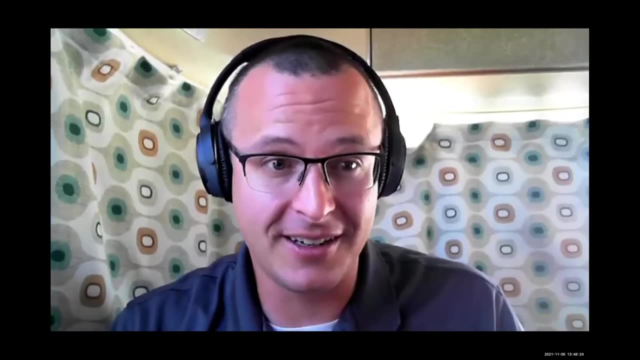 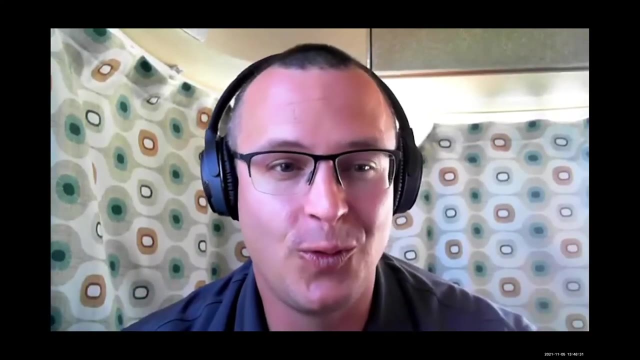 It's. some of the polymer composites that are coming out have a specific strength, like two and a half times higher than any of the metallics, but there are no property data out there just to decide how these materials perform in liquid hydrogen, So we're trying to do the measurements that way. 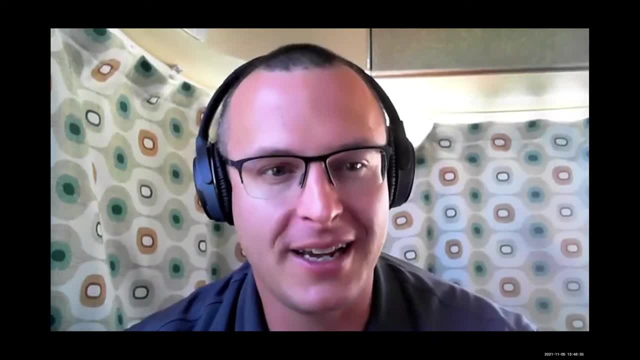 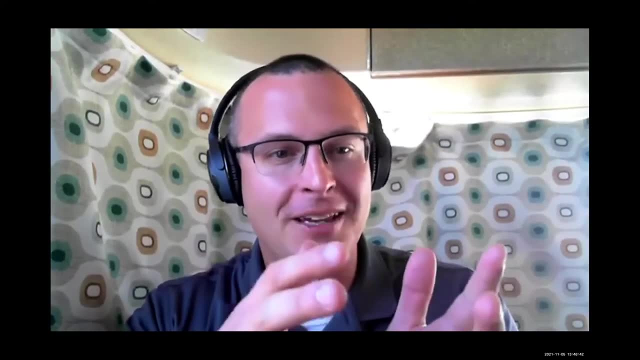 but that even there you're not getting really a lot of hydrogen per weight. So we figured out we could do something even better. We've got these bladders okay, Literally literally origami: thin film polymer bladders that everybody thought when NASA. 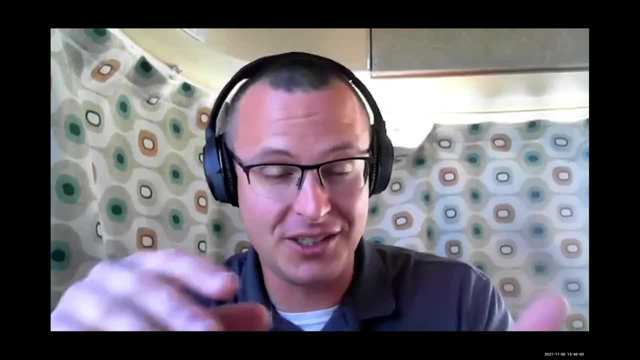 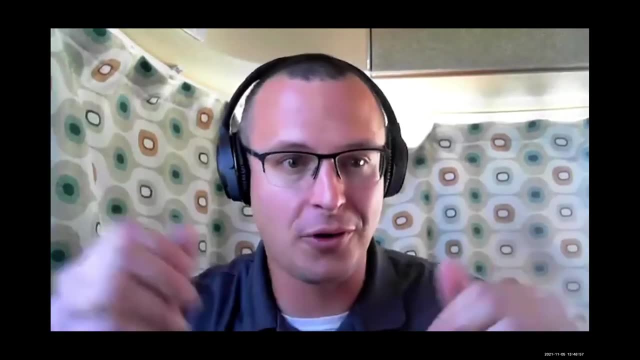 studied this in the 1960s. they shatter. No, you just have to fold them right And you can cycle these thousands of times And, moreover, you can make them double walled. We vacuum form them and you can cool the liquid hydrogen. 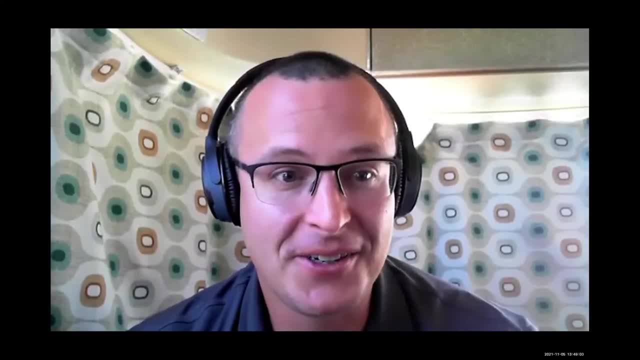 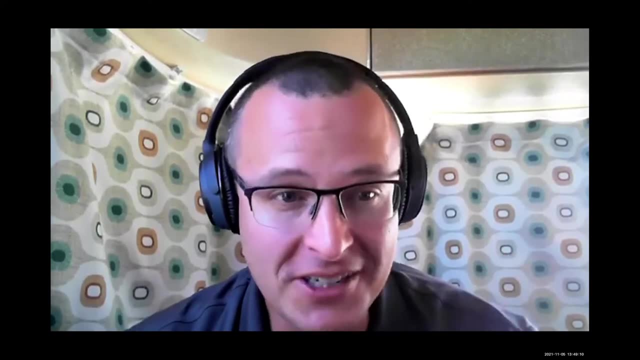 inside of these and you don't even need a metal tank anymore. So these are some of the things that we're working on, And I'll wrap it up with this. If you're interested in this, we have hiring opportunities, Openings at just about every level. 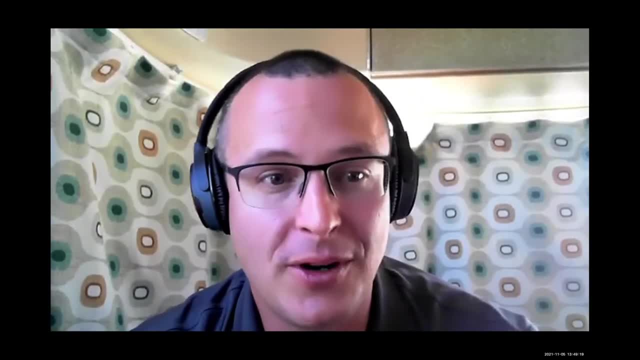 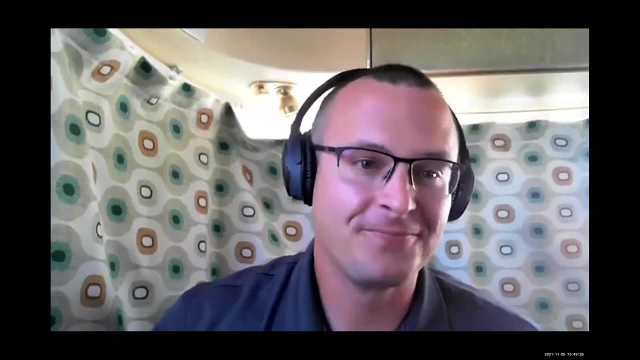 through the organization. Check out the jobs post here in the whoever app, And we need all the help we can get at this point, Thank you. Thank you, Jake, Very interesting. So now we'll turn over to Josh, who I think has some very interesting ideas about how. 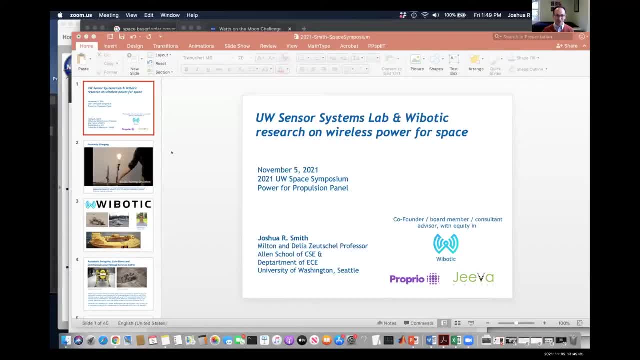 to provide space power. So, Josh, would you like to make an opening statement? Yeah, sure. So I'm just going to give you a little sense of some of the work that we do, Kind of adjacent, really, to the topics here. 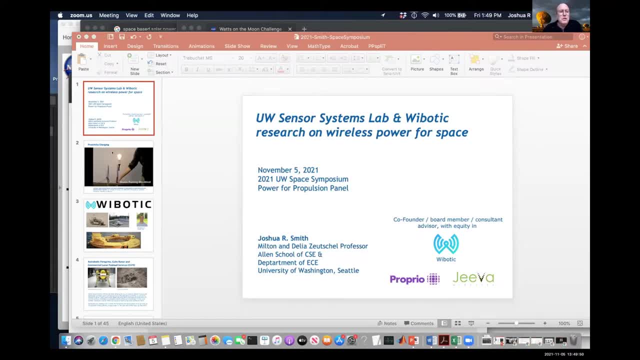 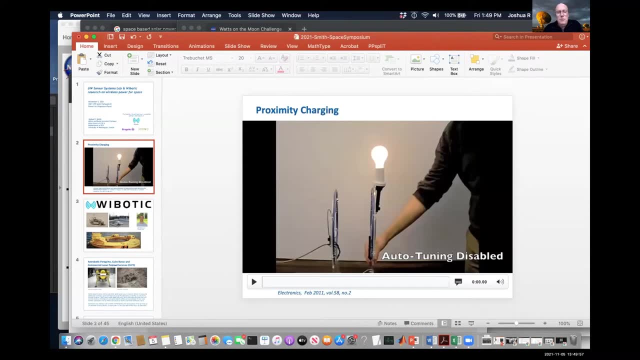 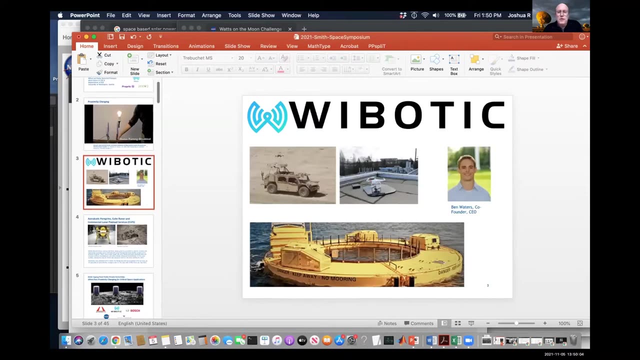 Less to do with propulsion specifically, and more about the distribution and management of power for space applications. So we've been working for many years on inductive power transfer And, in particular, there's a startup called Wibotic that my student Ben Waters and I founded. 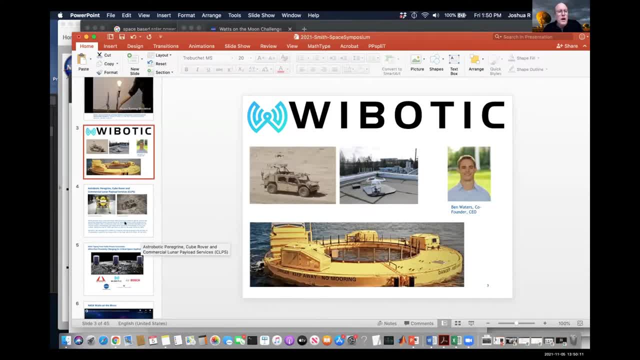 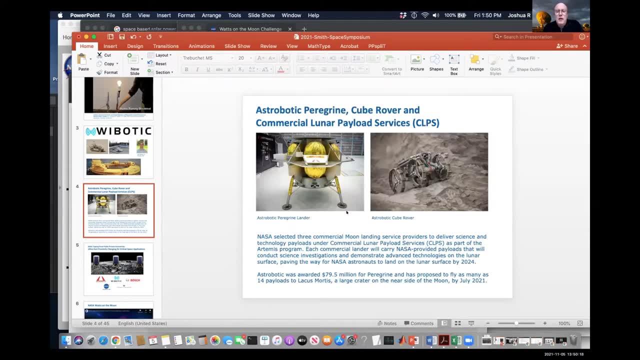 It's spun out of the lab to commercialize some of this work. Recently we've started working with say Astrobotic for a specific project called NASA's Tipping Point project, which aims to demonstrate wireless charging of these cube rovers, like you see here. 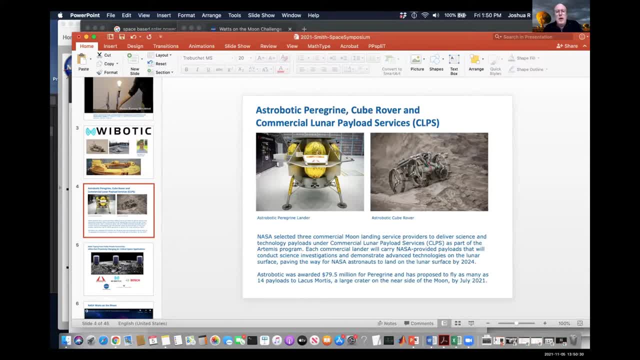 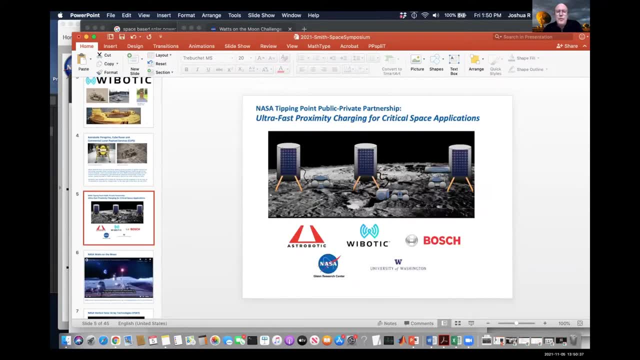 on the right on the moon. This is in conjunction with the Peregrine lander that you see on the left. that Astrobotic will be flying to the moon soon. So this picture kind of outlines the project. So you have power. 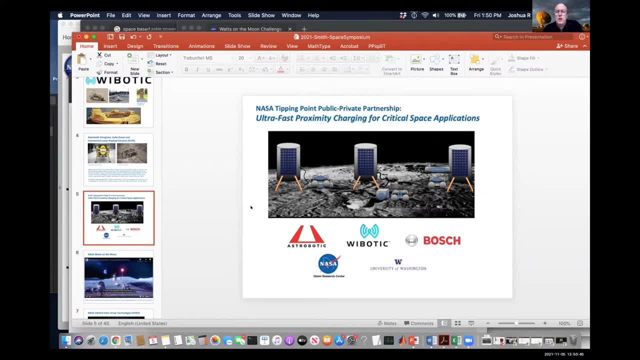 Yeah, Power sources such as solar. on the moon You have base stations that are sources of inductive power, And then these little cube rovers can move around, do their thing. In particular, one of the goals is to be able to survive the lunar night, which lasts three weeks. 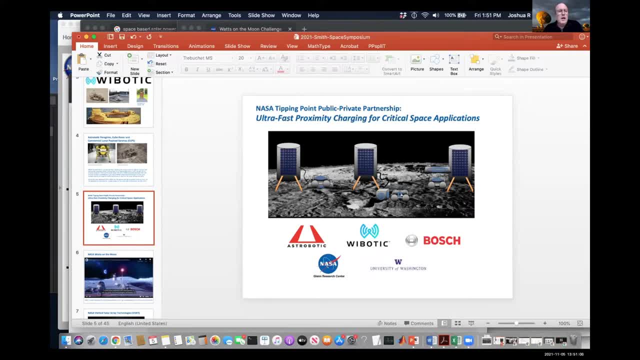 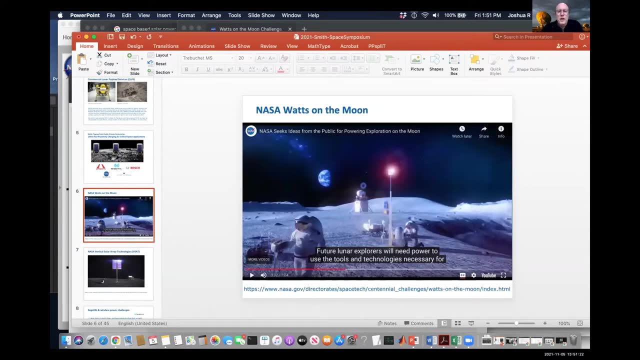 So it wouldn't necessarily be feasible for these cube rovers to carry their own batteries. but by having a larger power system and then distributing the power easily inductively, you can do more. This is also kind of: there are other adjacent things. 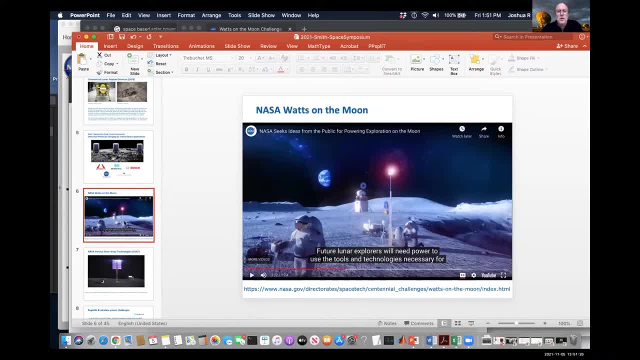 going on in this space. So NASA has a Watts on the Moon project that Astrobotic is involved with and some of these other collaborators, So they're looking at a variety of ways to distribute power on the moon, including beamed power solutions. 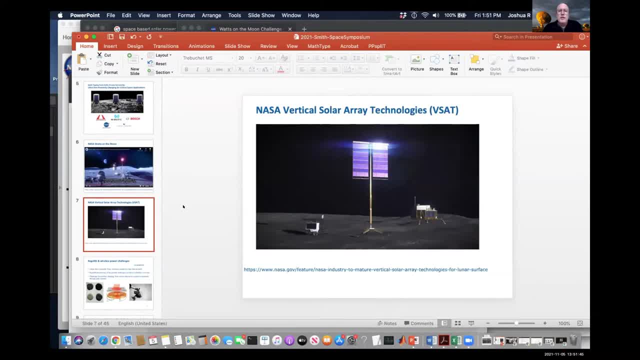 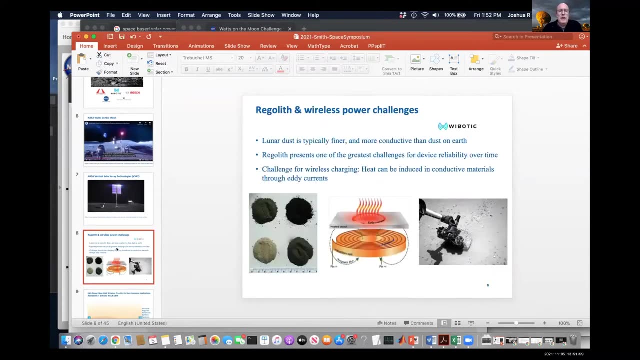 There's also the NASA VSAT Vertical Solar Array Technologies program that's going on. So this is aiming to build arrays of these vertical configurations for these applications. So one of the specific challenges we're looking at with the Tipping Point project is: will the regolith be heated by the inductive charging? 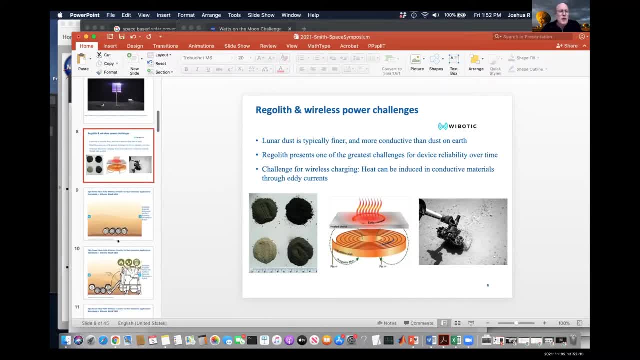 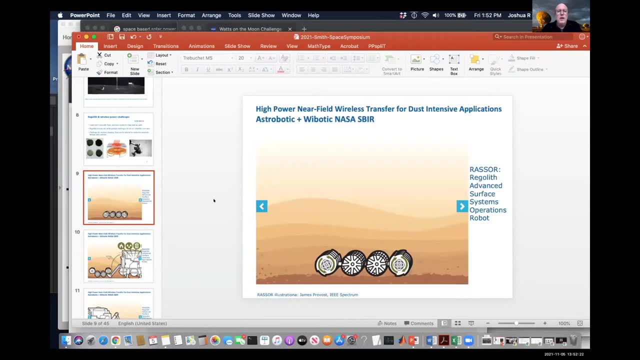 Yeah, Yeah, Yeah. So that's one of the things we'll be studying. The other thing, which actually Wibotic is also involved with, which sort of ties into some of what Jake is talking about, is in situ resource utilization. So we're working on this. 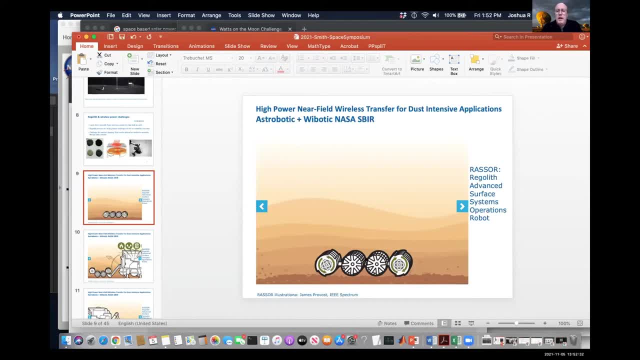 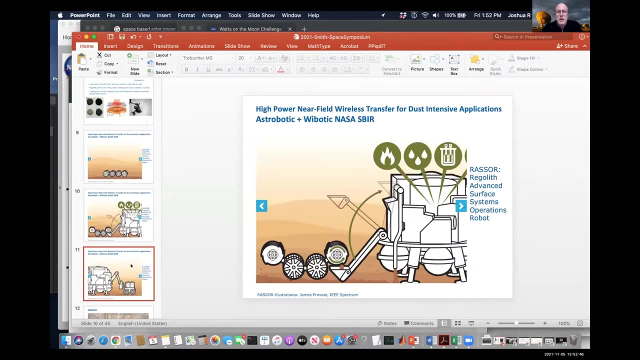 Well, Wibotic and Astrobotic are working on the RAZR, which stands for Regolith, Advanced Surface Systems Operation Robot. So the idea is that this robot will go around, collect dust on Mars or the moon And then it will be separated into hydrogen and oxygen. 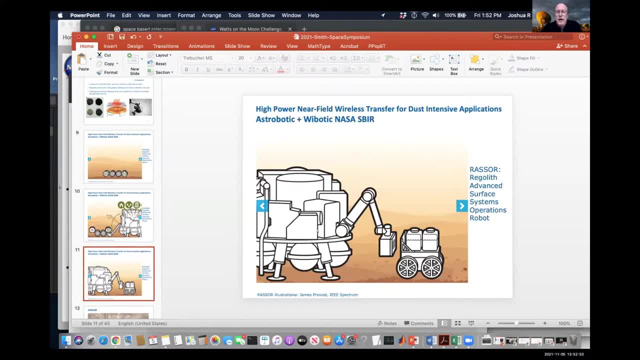 or hydrogen or oxygen will be extracted from it, And then that could be carried off and used as fuel. Now, of course that doesn't solve the problem of where does that energy come from, But it's more of a distribution issue which kind of ties into some of what Jake's talking about. 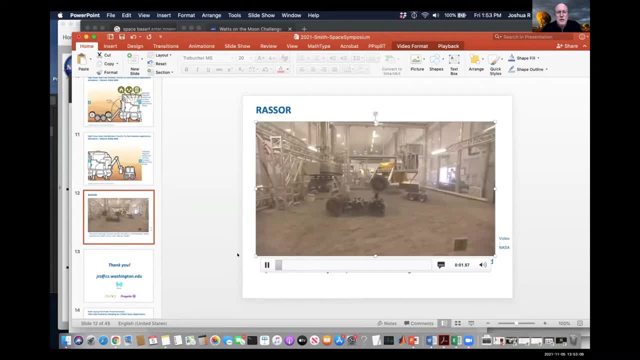 So our part of it is related to: if you have this dust handling robot, It's going to be very dusty, So how does that robot, the RAZR, actually get power? So we've been evaluating down at Kennedy Space Center, which 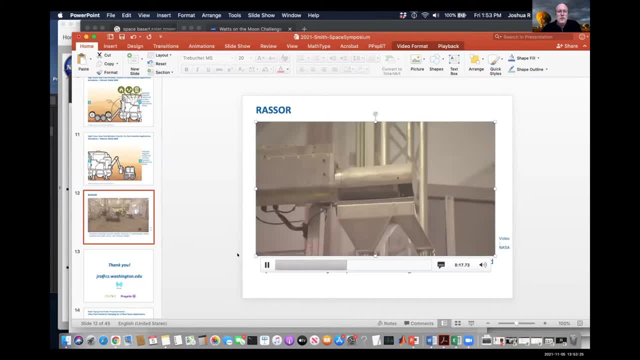 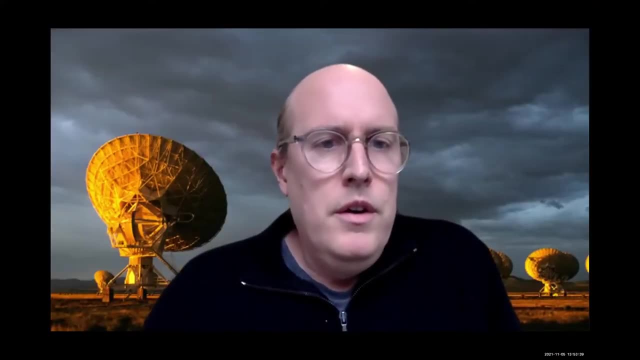 is where this video was shot. they've evaluated wireless charging of the RAZR system, So hopefully that will go further. So that's all I wanted to say for my introduction, Looking forward to the rest of the panel. Thank you, Josh. 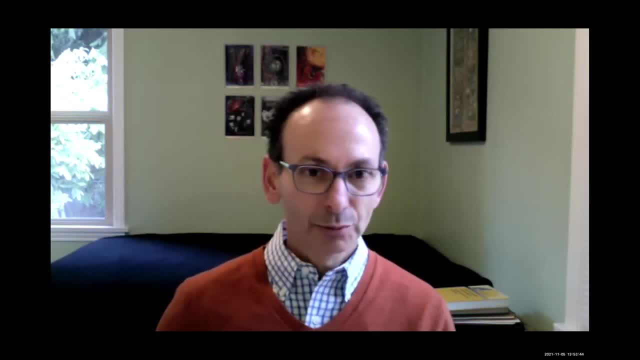 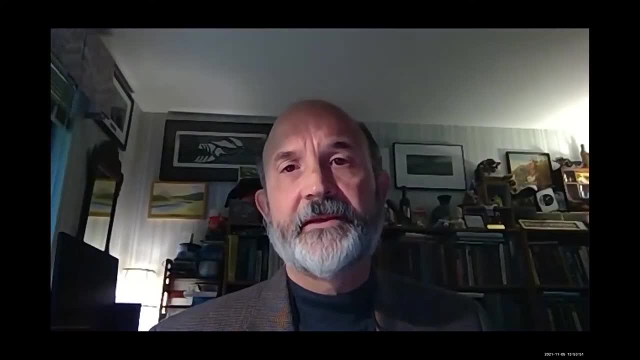 Very interesting. So, Roger, did you want to add anything in terms of an opening statement? Not really other than to just emphasize the points that Jessica and Jeff made about the challenges of fission reactors. I actually work with NASA some right now on their various programs. 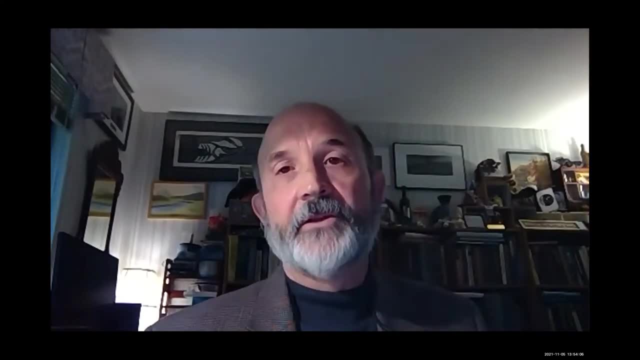 And they're really focused on the high assay, low enriched, the LEU approach, for the reasons that Jessica Jessica mentioned, And there's a big effort now to establish a testing approach for both, for either an EP or NTP, the electric or the thermal. 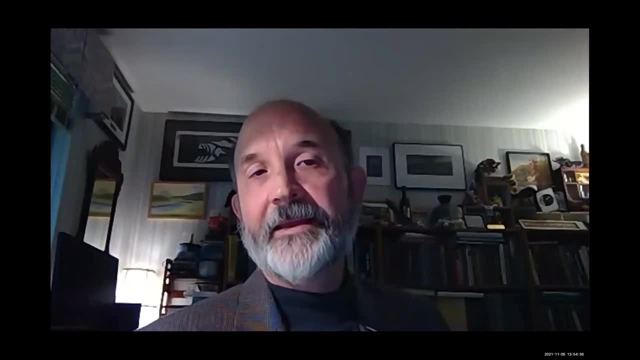 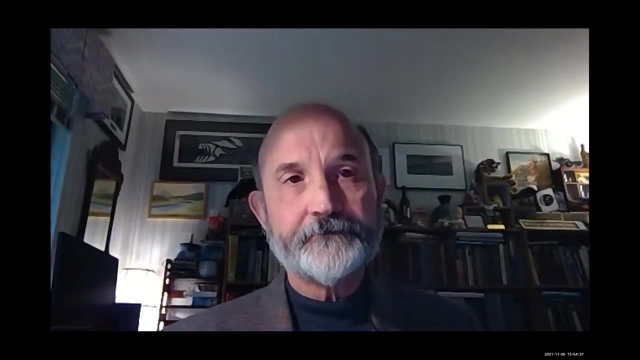 options. that is a credible way of qualifying and certifying for human missions, When you think about the requirements for these very big systems. Okay, It's very critical And it's really important. So, thank you, It's my pleasure, So thank you. 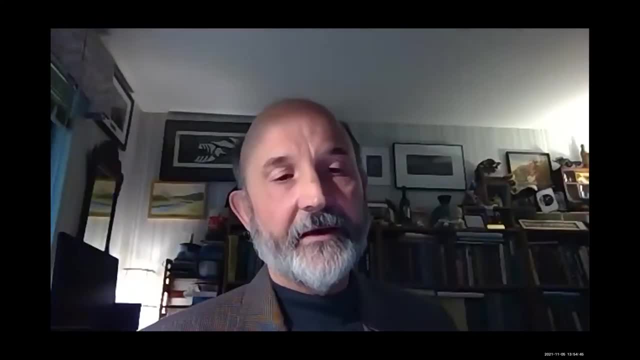 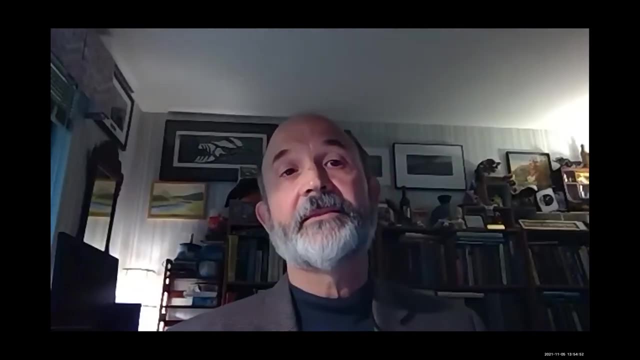 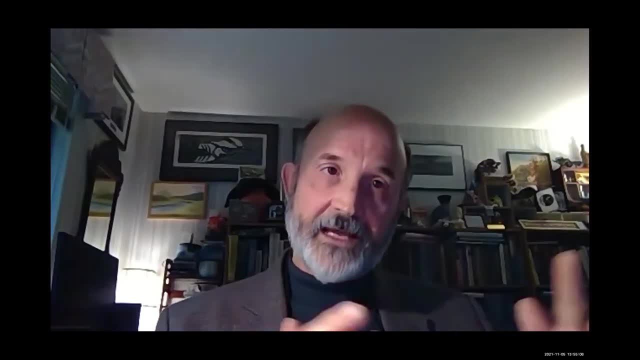 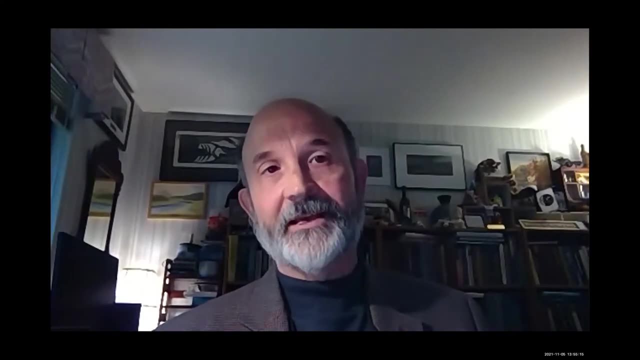 systems in particular. It's part of the reason that NASA is really focused on the high assay, the low enriched approach for that And, for example, making sure that when you launch the production systems, when you launch them, they're launched cold, But there's still the 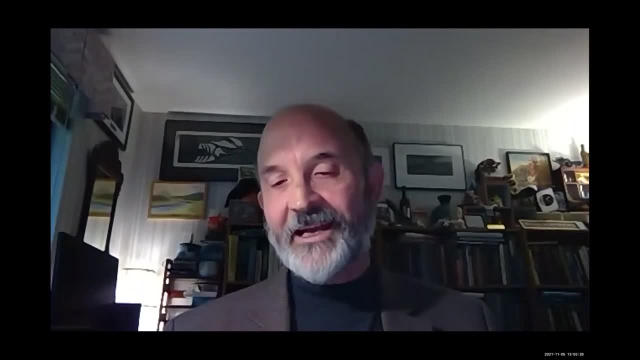 issue. for example, if there is a launch vehicle failure and you have an intact reactor that enters the water, there's the ocean. that lands in the ocean, there's. you know you got to have criticality, safety features, et cetera, And those designs are all. sort of underway at a relatively low level. But you know, in Seattle we have, you know, ultra safe nuclear. In Virginia there's BWXT And you know there are several companies there's. in California there's General Atomics. There are various companies now that are. 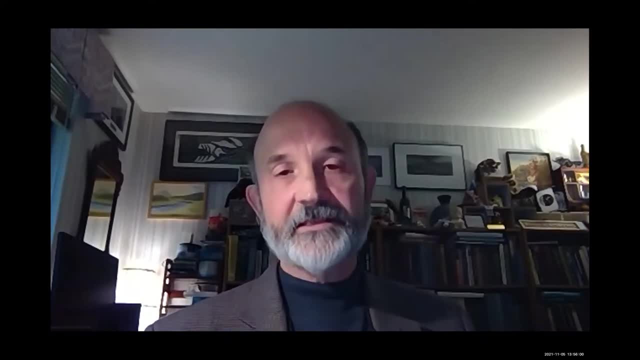 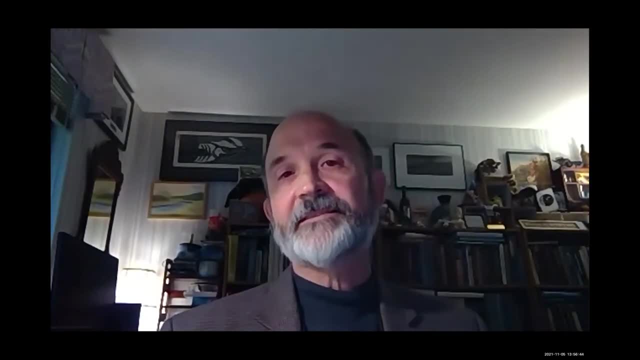 is something we should continue to think about. It's very complex, The packaging is very challenging, but we should continue to think about it, So I look forward to the discussion. I actually I love Josh's comments about wireless charging, the challenges of operating rovers and 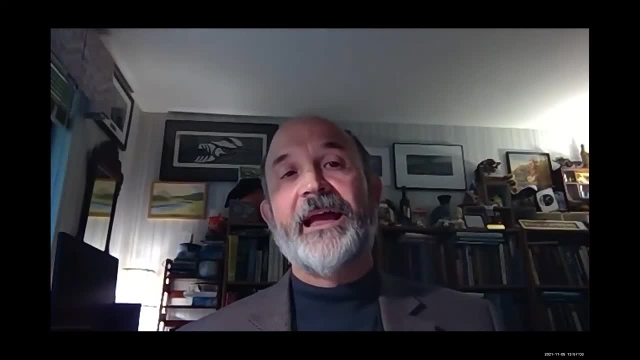 even for the fission surface power systems, for example. How do you get close to them after they've been operating for a long period of time on the surface of the moon, for example? That's a real challenge today. So enough said, we can move on to Q and A. 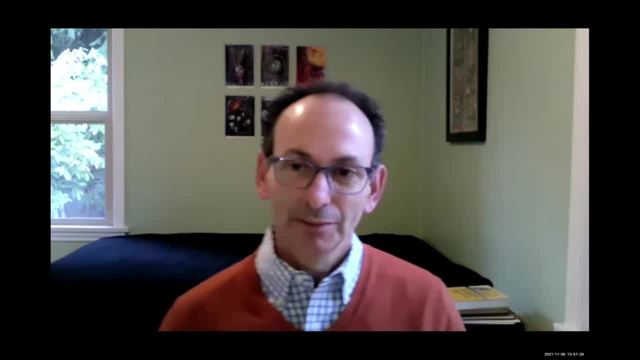 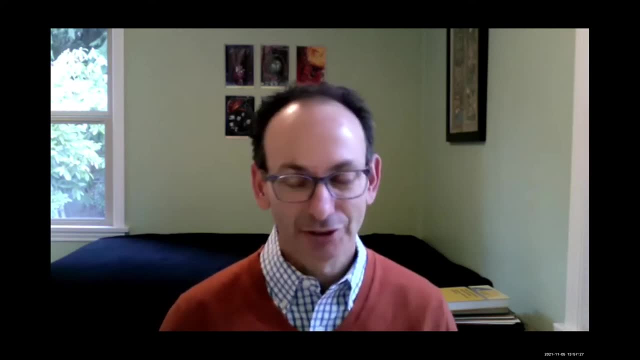 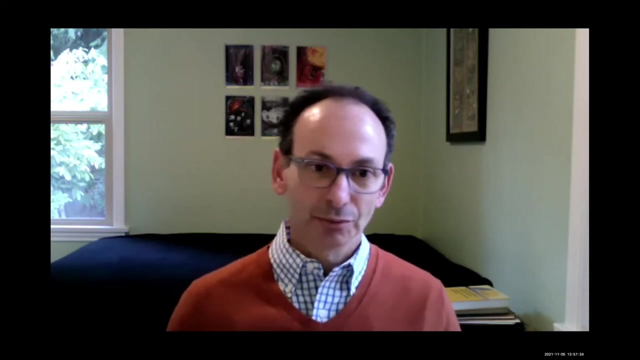 Great. Thank you, Roger. So I did want to throw out a question. So we've been focusing on nuclear power, which is also my interest, But I do also want to bring up maybe the other facet, maybe another facet which is as environmental awareness and 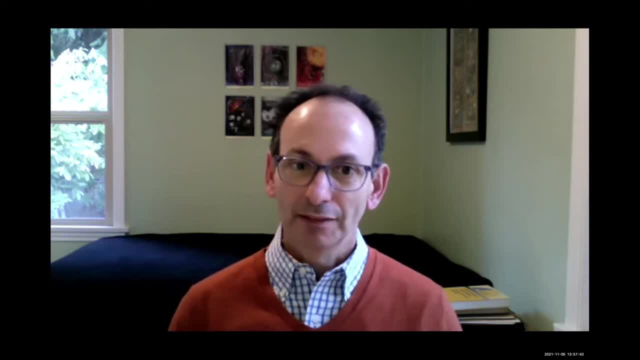 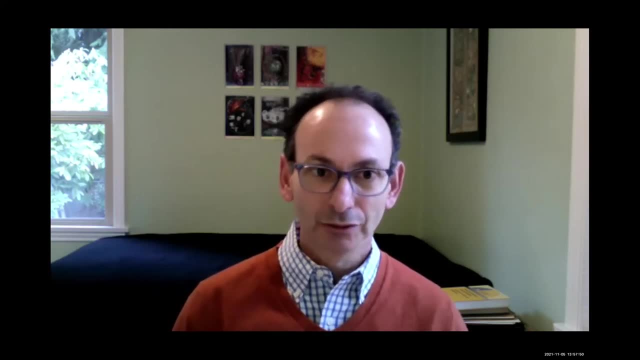 and concerns have increased. Is that pushing towards finding non-nuclear options for power? So, Roger, you talked about new solar panels and there's certainly been development of solar panels for trust fuel power. Are there opportunities to leverage that for space power? 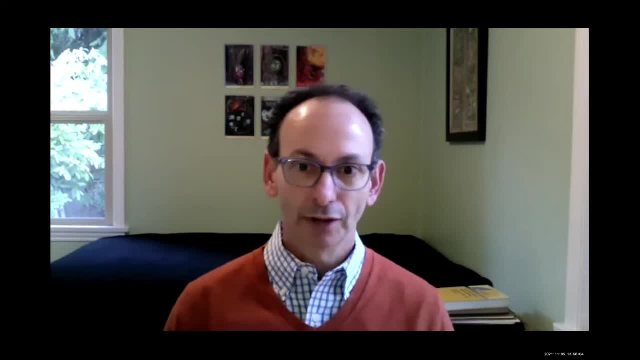 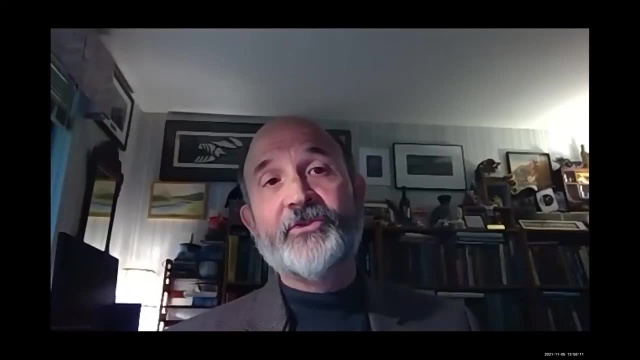 at least for local space power, or maybe, as you described it, AU less than one sort of missions. So, Roger, maybe you can say something about that. Sure, I mean actually new solar panel technology, new solar arrays, new solar cells. 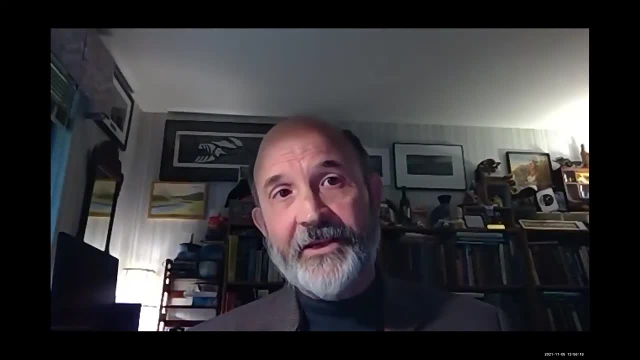 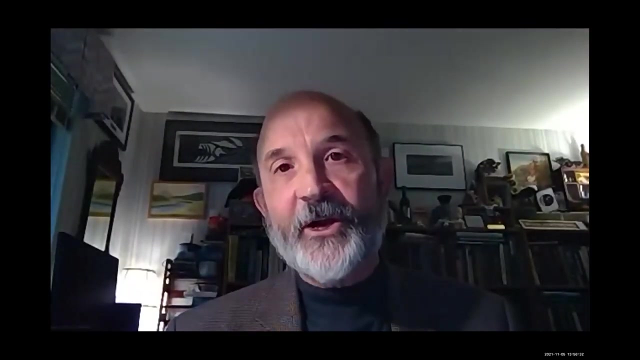 are continuously being invested in for terrestrial applications, Although for terrestrial applications the efficiency requirements and the mass requirements are not nearly as extreme. I mean 10 years ago, 15 years, let's see- when I entered the business. I have lots of gray now, so it was a long time ago. 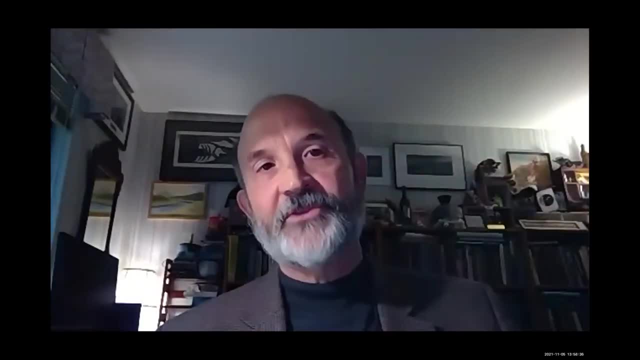 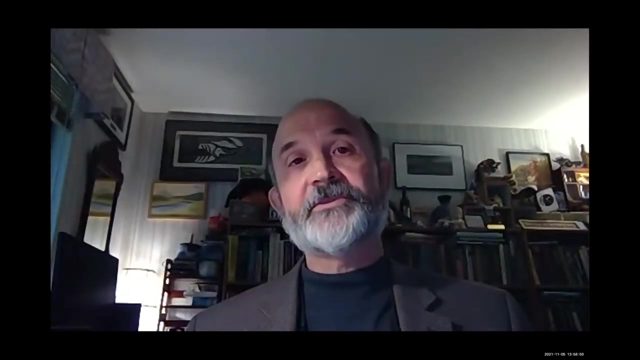 Nobody ever thought we would be flying solar missions to Jupiter. Well, now we're flying two. Right, Lucy just launched, and we have Juno, which launched several years ago. So it's clear that the and that's to Jupiter, let alone Mars. So the penalties associated with going extra solar are decreasing as solar technology advances- solar and battery technology- don't forget the batteries. But they are still extreme and one of the big challenges, for example, for the lunar surface right, is that the lunar night is two weeks long. And if you scale batteries to work for two weeks, they get to be enormous And you just can't. the mass trades just don't work very well. In addition, when you look at overall architecture, reliability for crewed missions- you need backup systems. that are very reliable for surface power, And so the question is: how do you arrange a large enough set of large solar systems with their batteries to deal with on the moon a two-week night, or on Mars, a one-week night, but with a lot less because of the distance to Mars? 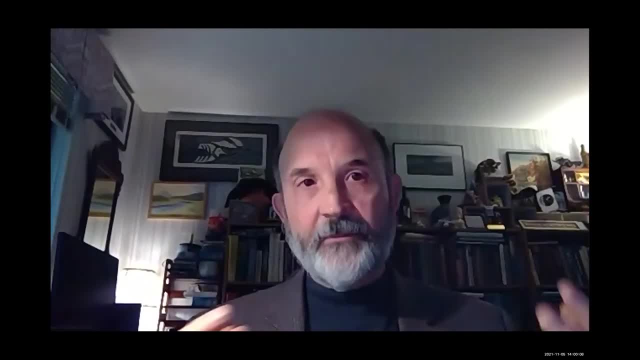 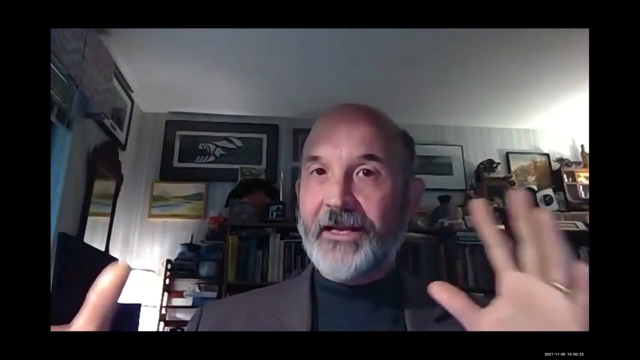 and the challenges of communication. there are other reliability factors that need to be assessed when thinking about power systems. So the advances in solar array technology in my mind are very exciting because they are non-nuclear, so they don't carry the regulatory challenges. But there are some missions where that just won't work, and at least not today- And so we really do need investment in fission systems for, you know, to enable new missions that we haven't been able to do: Crewed missions to Mars. 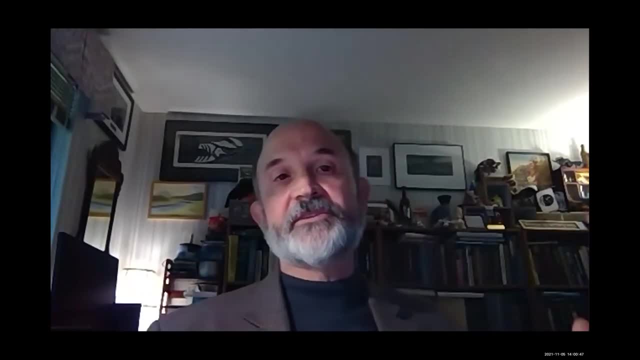 or staying the lunar, having a permanent presence on the surface of the moon. You know, there are architectures, solar architectures, that might work, that might, for example, use some of the beam, be a combination of solar plus beamed to get the energy down. 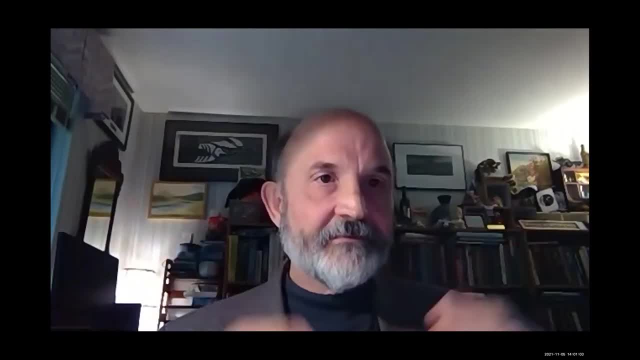 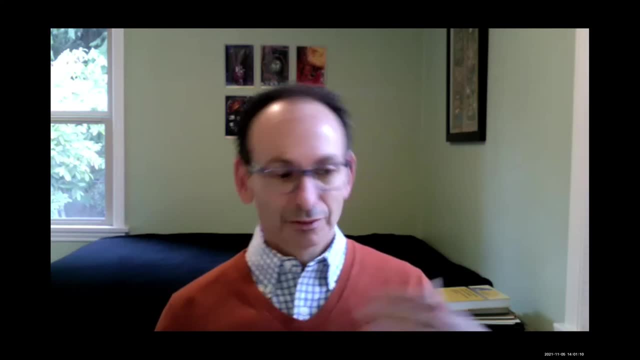 into a permanently shadowed region of the moon. But you know so. anyway, those are my. that's a quick, quick answer, Right Yeah, So you know, in discussing kind of the evolution of technology, which has certainly evolved in significant ways, 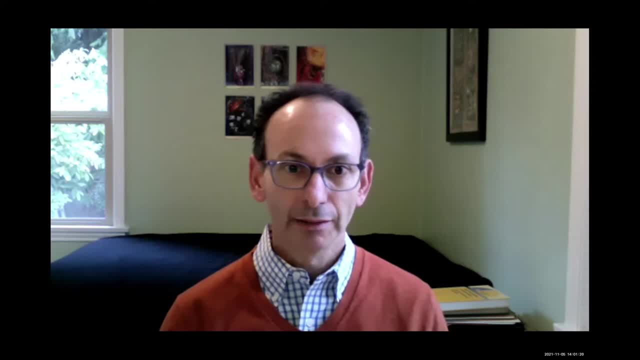 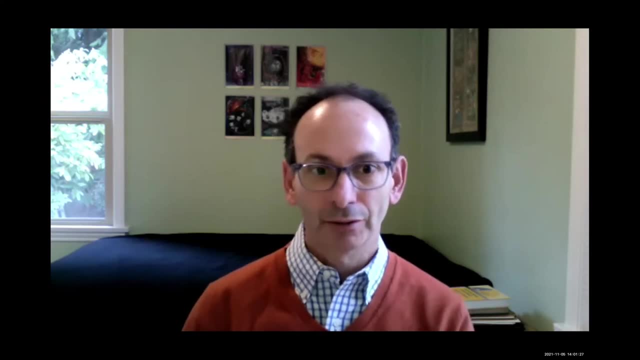 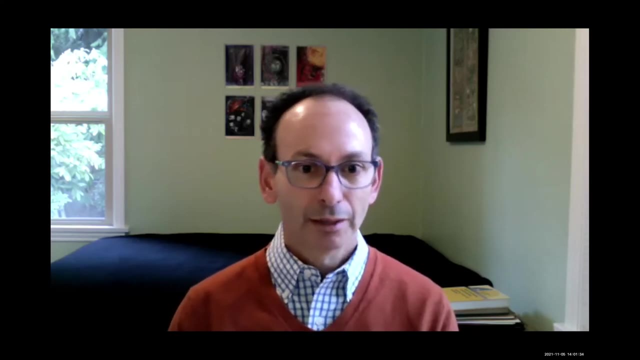 certainly policy issues have also evolved And I think in particular the last few years things have changed quite rapidly. So maybe, Jess, can you describe how some of the US policies have developed and also in the context of how there are international legal considerations regarding nuclear energy in the space. 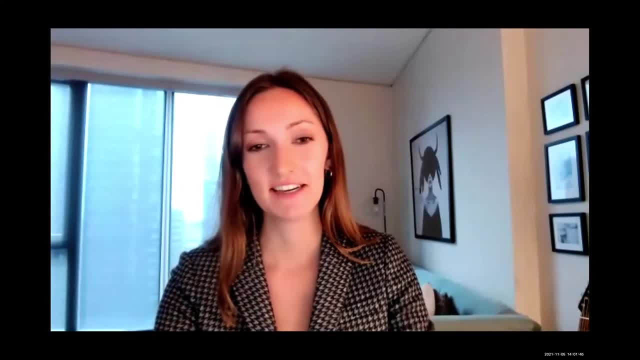 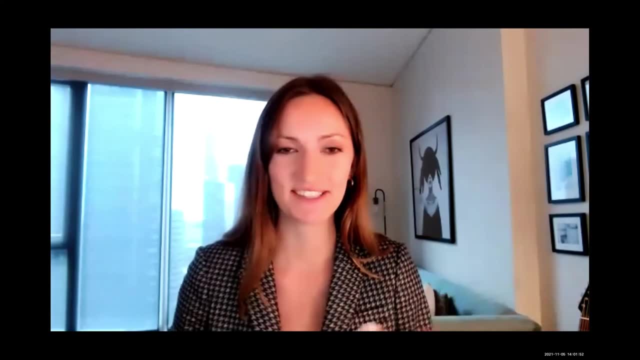 Yeah, happy to. So let me start off by saying the rules have developed, but there's still a lot, of, a lot of need to catch up with technological development and constantly reassess where we're going, what the risks are, what we need to address now. 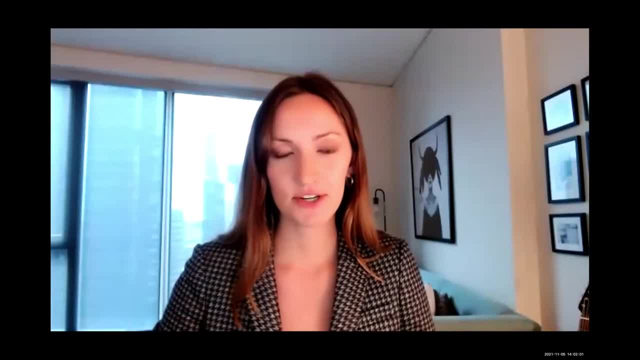 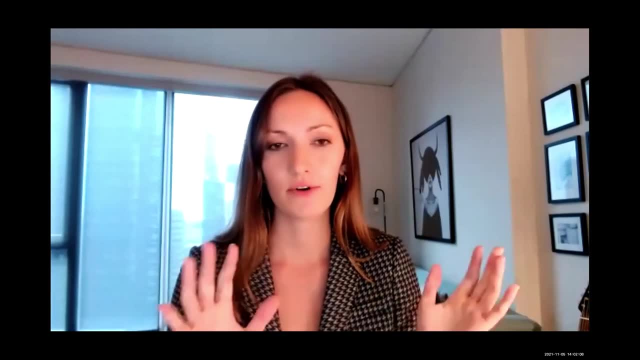 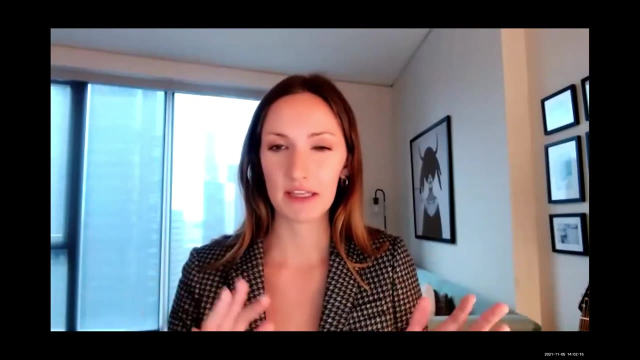 so that companies can prepare for these measures. So just going back real quick, the long-standing US policy for particularly nuclear, was to reduce the use of highly enriched uranium, And that's something that's really important, I think, for space propulsion. 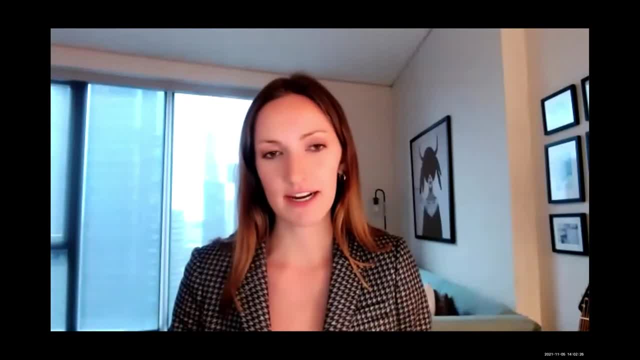 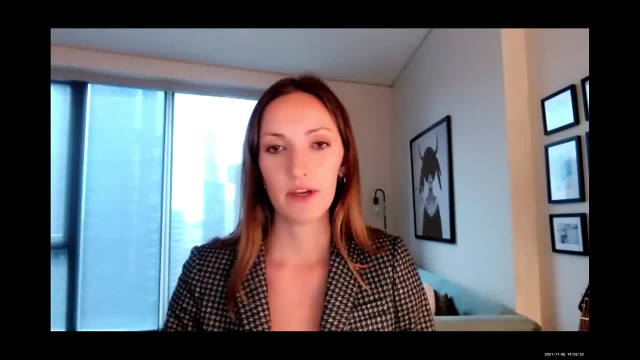 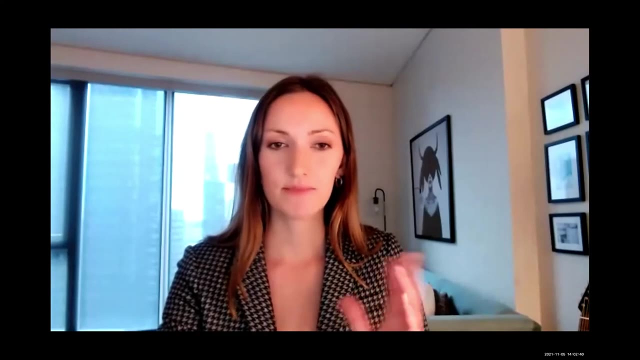 because we might. we've invested a lot as a country into making sure that other countries also go away from highly enriched uranium, have helped them use low enriched uranium, And so that's one big thing that has been addressed again more recently with regard to space nuclear power, So in 2020, I think this was the last Space Policy Directive, Space Policy Directive 6- of the Trump administration. The administration decided to limit the use of highly enriched uranium fuel to applications for which mission would not be viable with other nuclear fuels or non-nuclear power sources. 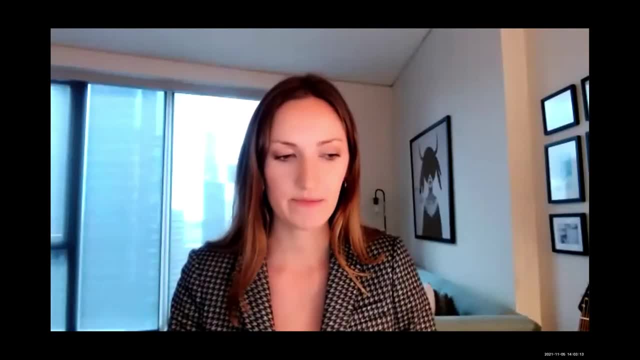 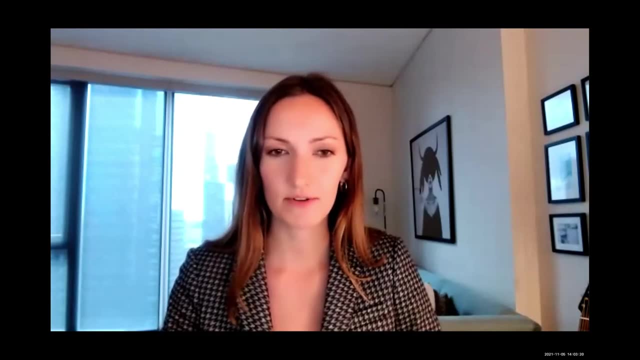 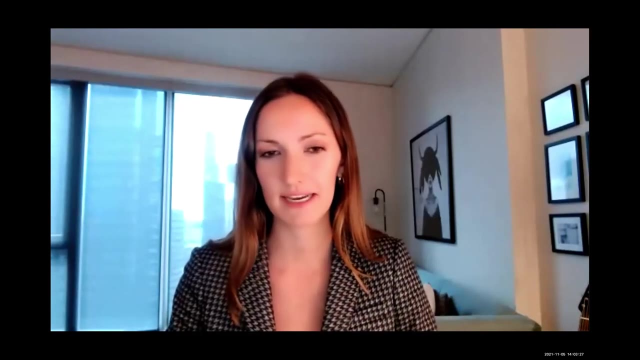 So that was some- I think, one of the biggest developments that we've seen in recent years- that now I don't think it's really possible to justify for US operations the use of highly enriched uranium anymore, unless there is really a huge need and you can't really close out a mission with lower enriched uranium. So the weight, the costs, performance advantages would really have to be rather big And so that's been a big difference and a change, because NASA was a little bit looking into the highly enriched uranium fuel reactor. 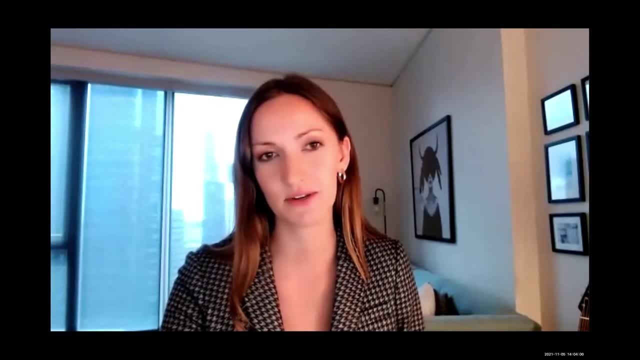 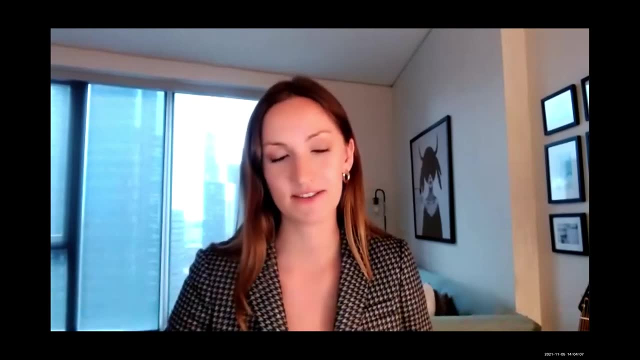 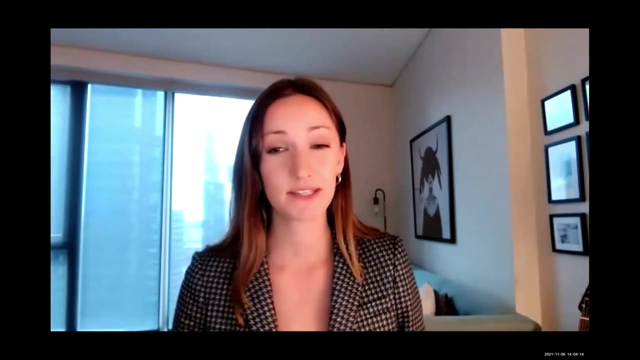 So I think that's what I see as one of the big, big changes in US policy. And then also, we had a little bit more attention coming to the regulatory space In 2019, there was a presidential memorandum on launch of spacecraft containing space nuclear systems. 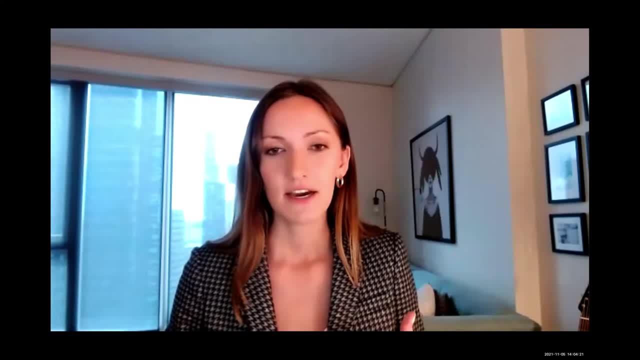 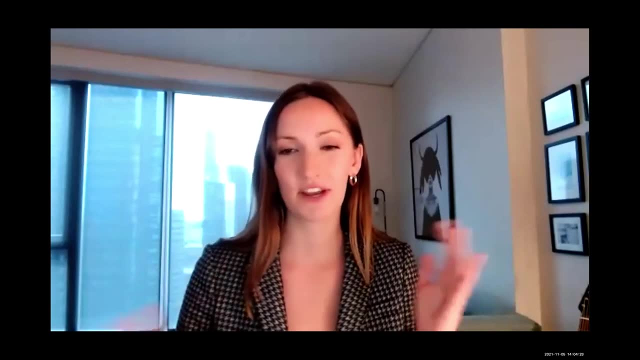 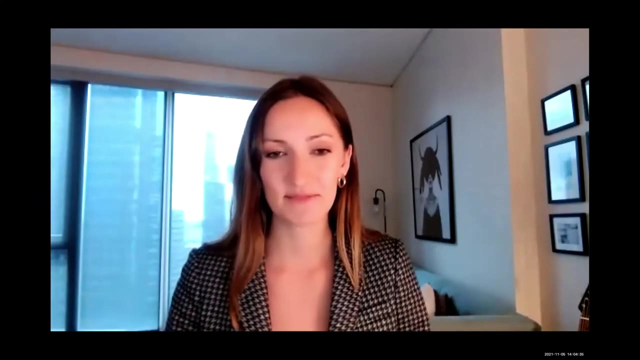 and that revised the launch approval process. We saw here a little bit of this: this consideration to balance regulatory requirements with commercial desires to raise capital and also to market these systems to to foreign customers. So the launch approval process was reformed. I would say in part to support this commercial development through a more tiered structure and establishing more of a pathway for commercial launches to be regulated by the Department of Transportation. Those were the two big, I think, policy developments in the US. 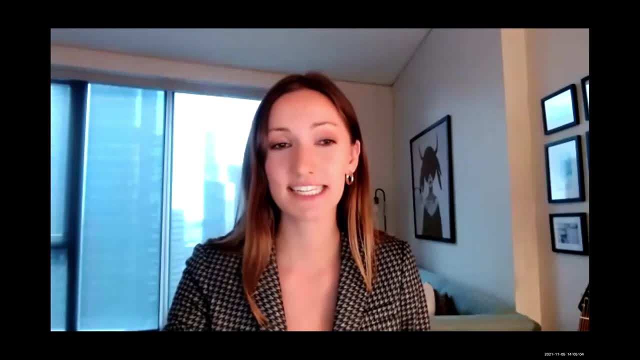 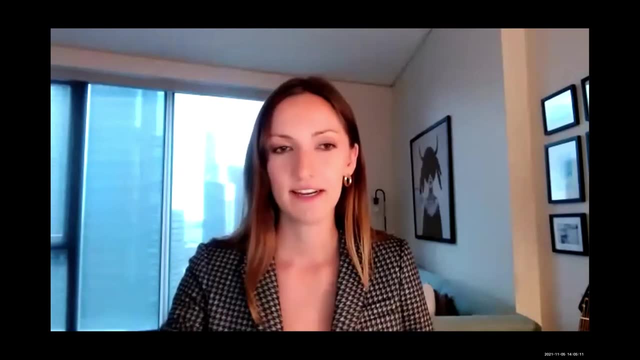 And then internationally. I think there's still a lot to catch up on. International law obviously applies to space, and IEA safeguards will apply to any nuclear materials used in these, in these reactors. But then there's instances where I still see a lot of need to catch up on. because you can't really reach the fuel once it's up in space And just monitoring what happens with it. there is a whole other story. So we'll have to develop some probably technologically innovative solutions to make sure that our safeguards are effective and also for nuclear security in general. 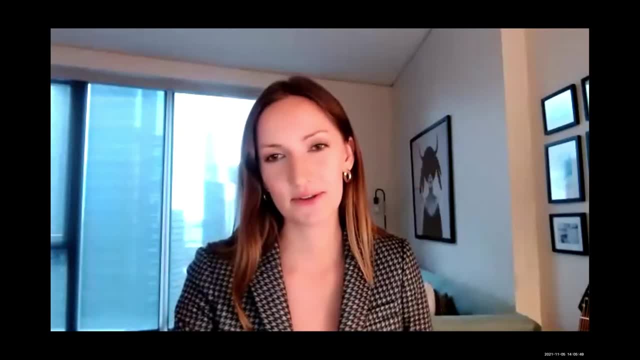 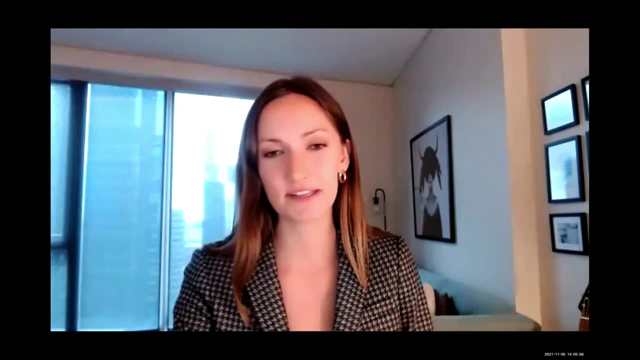 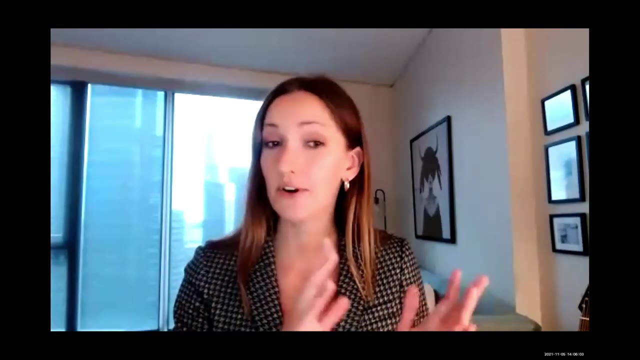 But we do have the principles relevant to the use of nuclear power sources in outer space. So that was the UN General Assembly resolution. Those aren't typically generally binding, but still something that states should follow, And those were largely focused on safety rather than security. 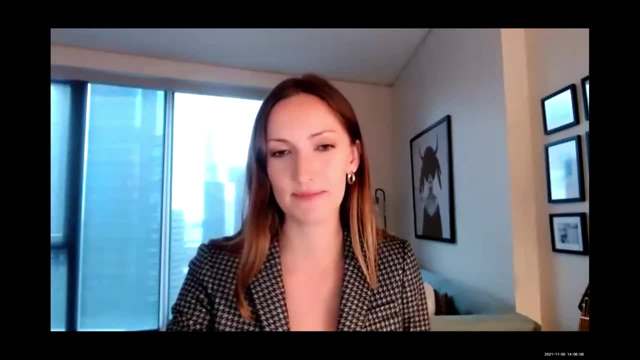 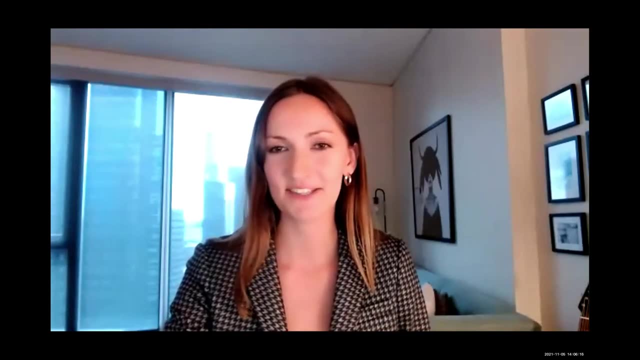 So I still see a lot of need here to catch up, since they really focus more on safety, giving notice, emergency assistance and damages. Yeah. So my conclusion, I think, would be: there's still a lot of need for policy development, Sure, sure. 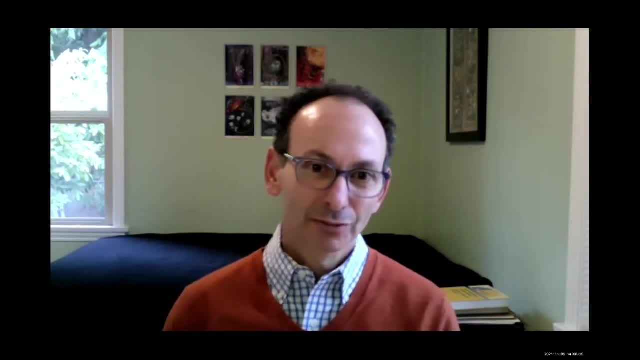 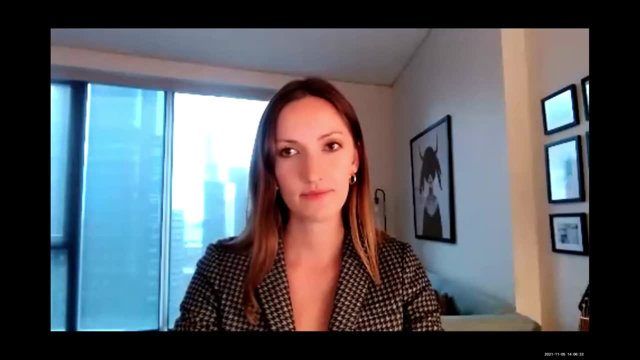 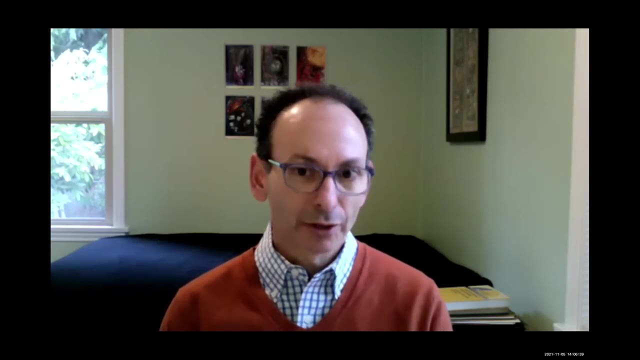 Great, Thank you. So so, Jeff, you know so just touched on the development of of commercial commercial applications, and we've certainly seen commercial space become more relevant in the past few years. How do you see opportunities to apply RTGs or even nuclear fission? 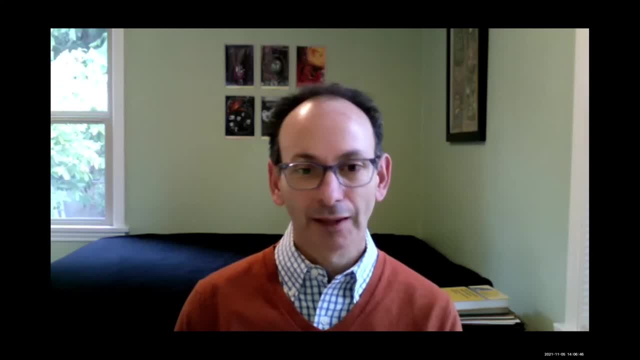 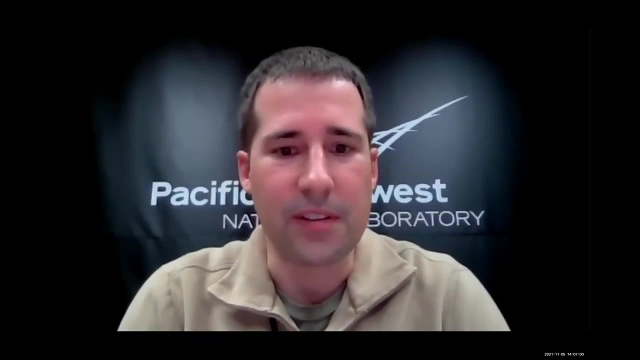 for commercial space, And how do you think that complicates things Or does it actually provide new opportunities for improving the technology? Yeah, thanks for that question. You know it is really pretty interesting If you look at how things were organized under the SP100 program. 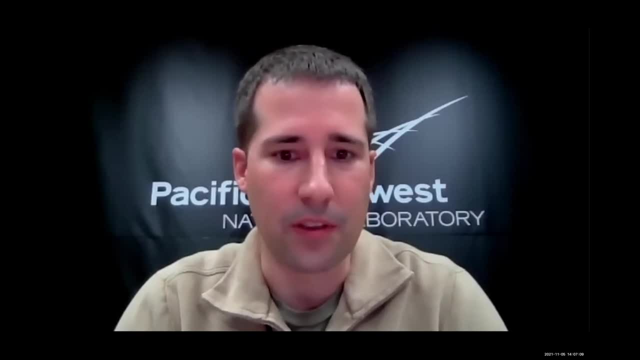 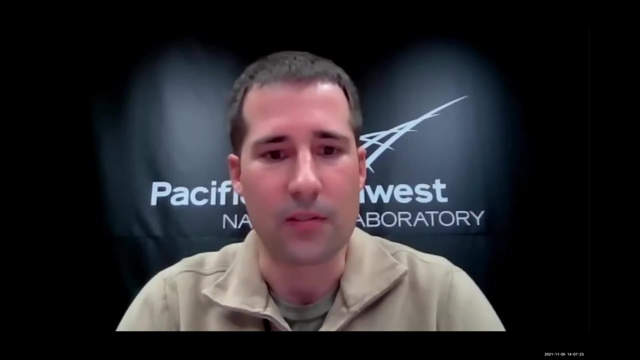 they divided up a lot of the technical aspects of that among the national laboratories for development. But today, as you see NASA issuing these calls and also DARPA, they're not going to the national laboratories, they're going to the industry And so 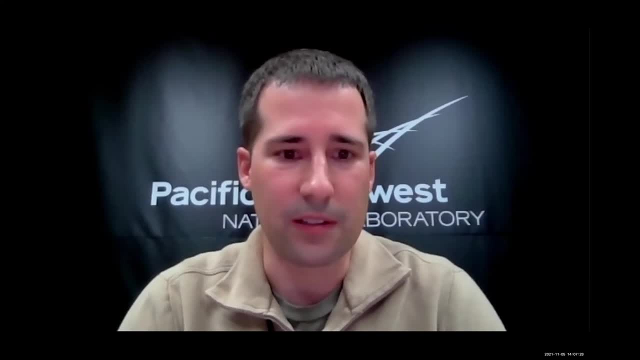 I think it's sort of a. it's going to be interesting to see how the emerging environment or commercial actors to be developing and implementing both RPS as well as space reactor systems, whether that's, you know, nuclear thermal propulsion or space reactors for power at large. 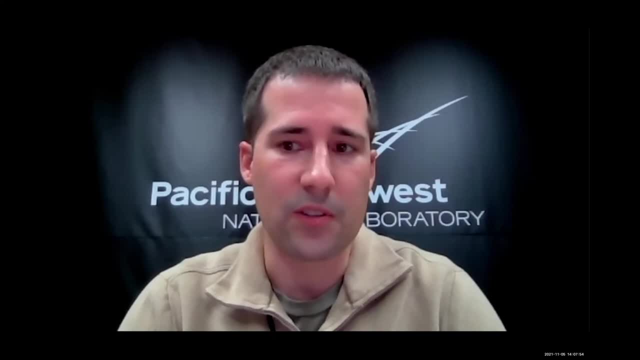 So you know, I think that this is something that's going to continue to expand And it will be interesting to see how that market evolves and where it goes. But I do think that that's one of the most exciting aspects of space nuclear power in general right now. 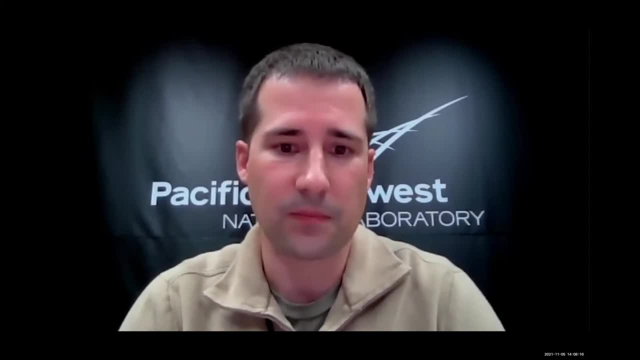 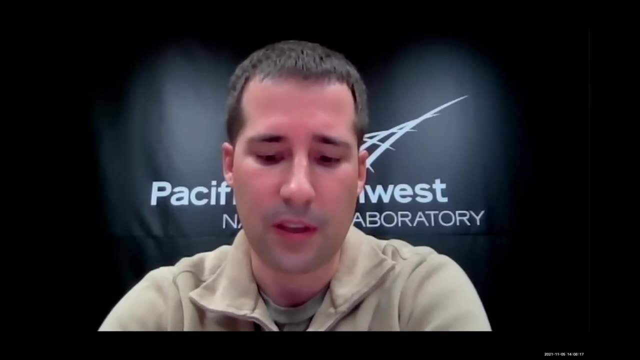 is the increased involvement of the commercial sector. And now, regarding the fuel immersion aspect of that, in my mind that's one of the drivers behind the use of HALU fuel is that I think it makes it simpler for commercial entities to be significant players in space reactors. 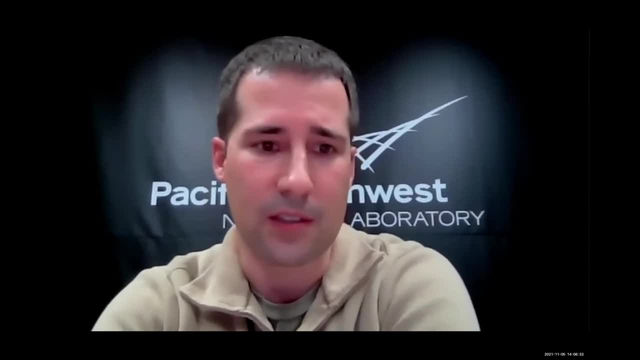 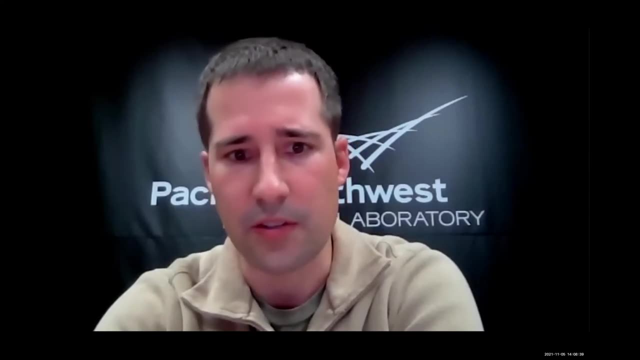 because it would be a lot simpler for them to manage HALU fuels as opposed to highly enriched uranium. And with respect to RTGs, I think it'd be challenging for commercial entities to work with plutonium-238, but they can likely successfully work with alternative radioisotope power systems using different isotopes. 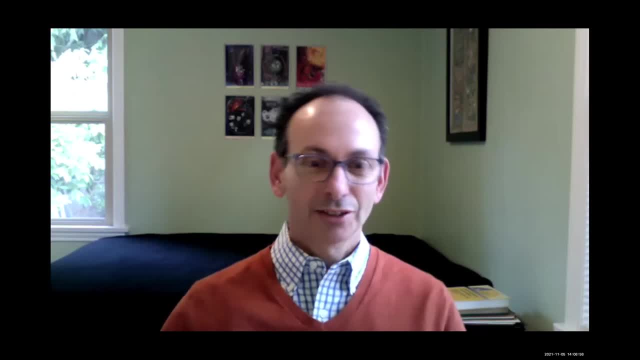 Great. Thank you, Jeff. So so, Jacob, you touched on the challenges of storing hydrogen for you know, at least in my mind, a relatively short mission to the moon. What are the challenges for storing hydrogen for deep space missions where you have to store? 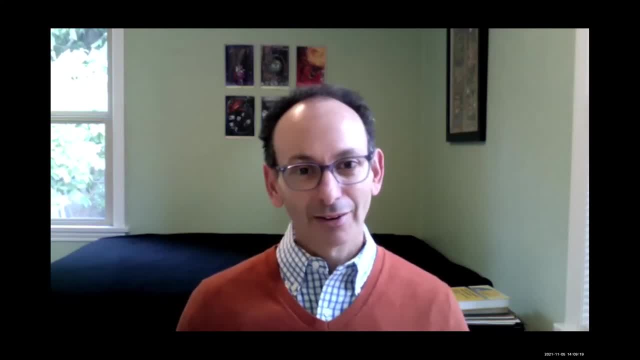 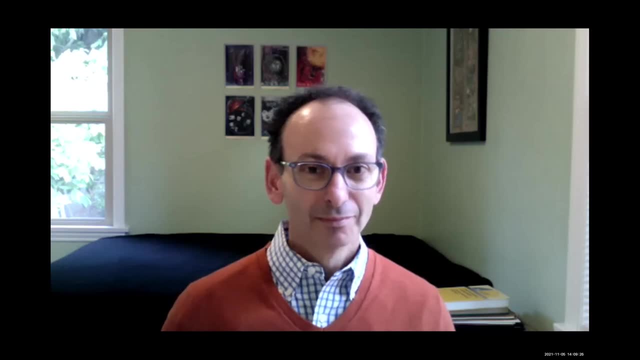 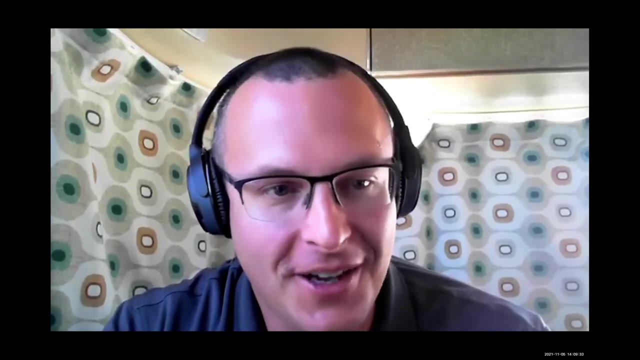 for you know many years, And also if I could get your thoughts on how is storing hydrogen different than storing helium? Yeah, that's a great question, Yuri. So the my friends at NASA Glenn came out and gave a talk a few years back about their design for a liquid hydrogen thermal. thermal nuclear rocket to go to Mars And the amount of cryo-cooler technology they would need and the amount of power they would need to cool that liquid hydrogen- to prevent from venting hydrogen continuously into space on your way to Mars, was just not even feasible. We're talking orders of magnitude, A way from being close to doing this. Now, the thing is, though, physical law allows that technology to be improved substantially, to the point where just a solar panel array could allow for efficient enough cooling to have zero boil off. I don't know how far out away from the sun you could do that, but for quite a quite a ways. And that same cooling technology that enables zero boil Off also enables efficient liquefiers to work, So it's one thing that can solve both challenges. 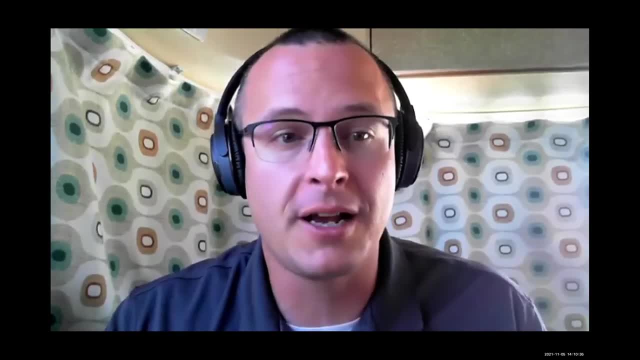 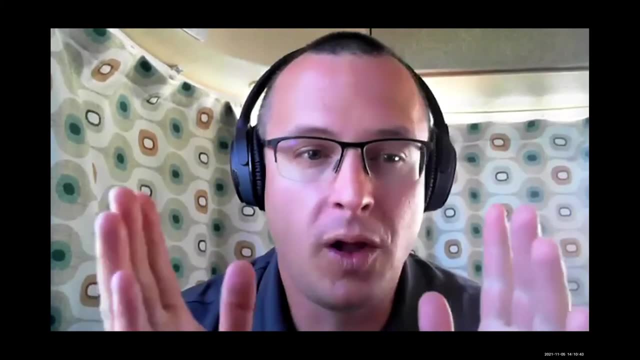 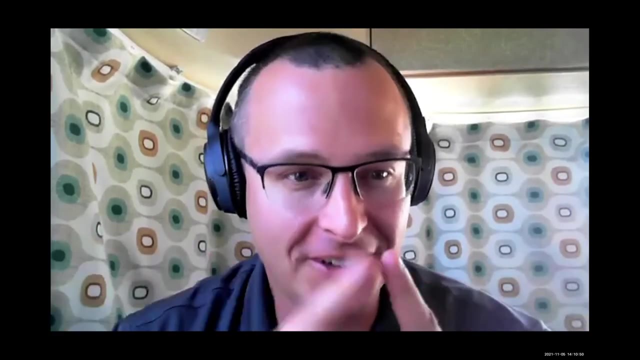 the liquefaction and the storage, but we need more programs looking at how you can cool that hydrogen very efficiently. Now this is where it gets interesting comparing helium to hydrogen. A lot of people don't realize that helium and hydrogen are more quantum than classical fluids there. 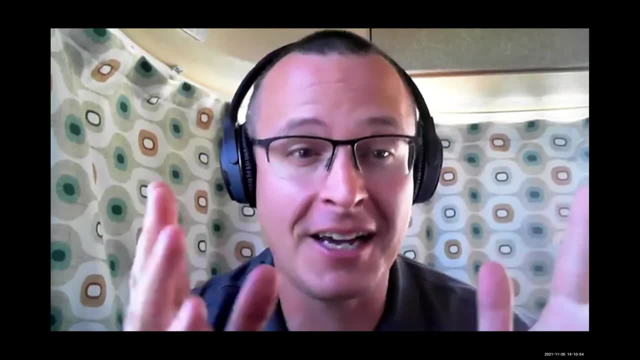 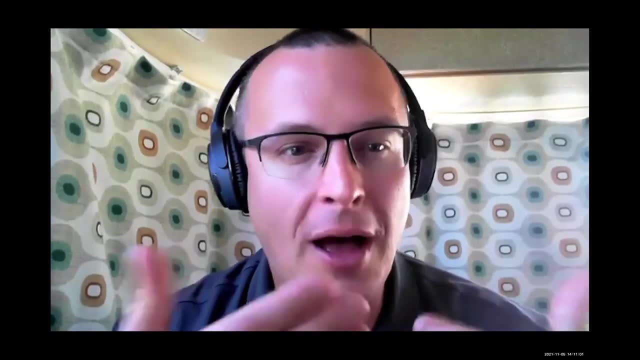 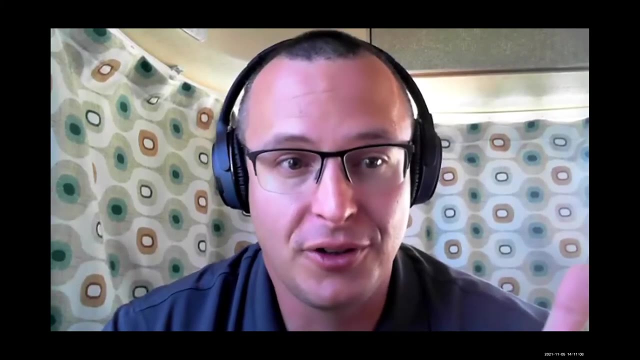 They have a thermal de Broglie wavelength that can be many times larger- there They act than the average distance of interaction, even in the gas phase, And that presents new opportunities for kinds of technologies that we haven't even envisioned yet, because we can't do it with classical fluids and systems at room temperature. 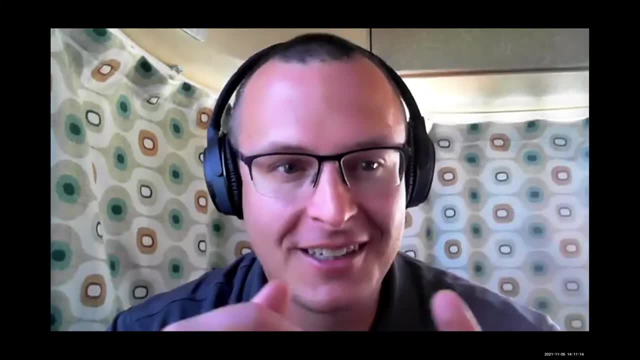 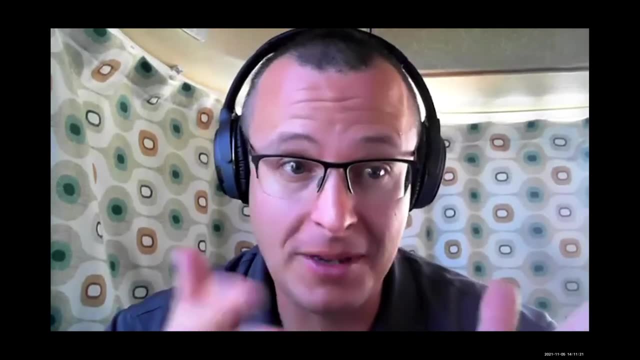 So that's where we need more basic measurements. We need more people researching on this, the load TRL stuff, because you're not going to find people in industry that can really do this Well, because there isn't even measurements for them to design a system from. 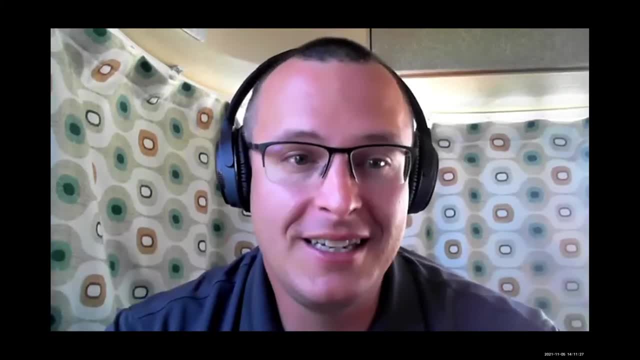 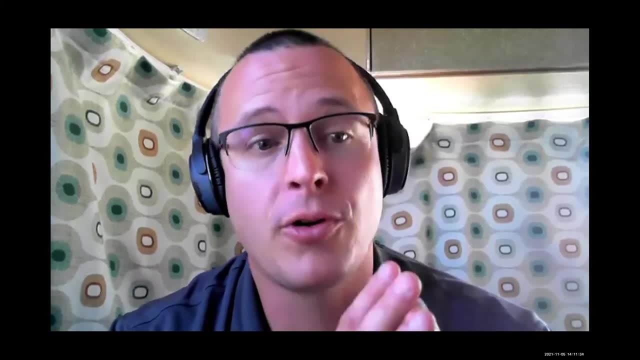 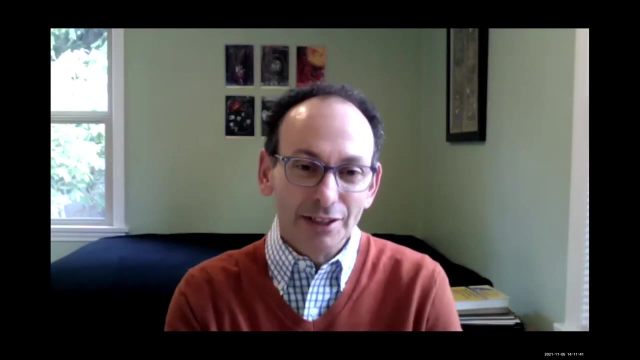 So that's an opportunity that we really need some basic research in the national labs and academia to start helping us out with, and we need the federal programs to start supporting that. Great Thanks, Jake. So you know my interest, of course. 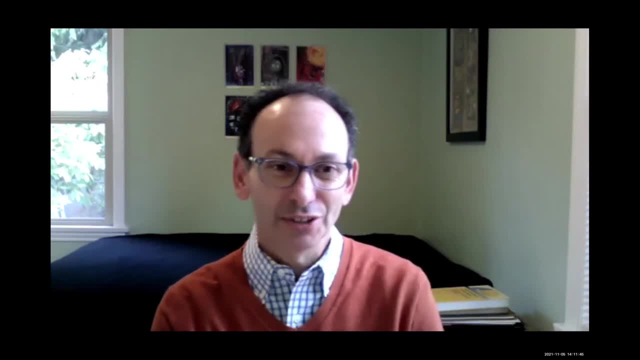 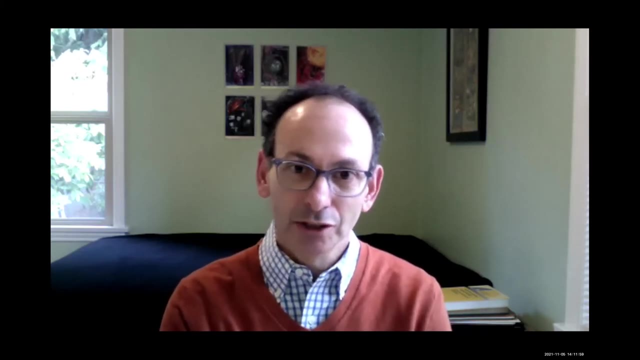 in helium is helium-3 and deuterium for fusion reactors. And so, Josh, in your slides you described mining the regolith For hydrogen, But one of the speculations is that it's also quite rich in helium-3.. 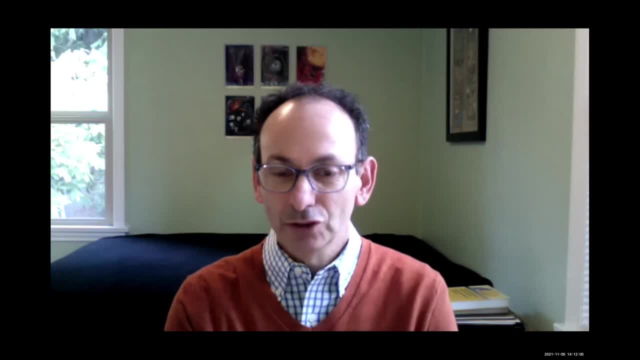 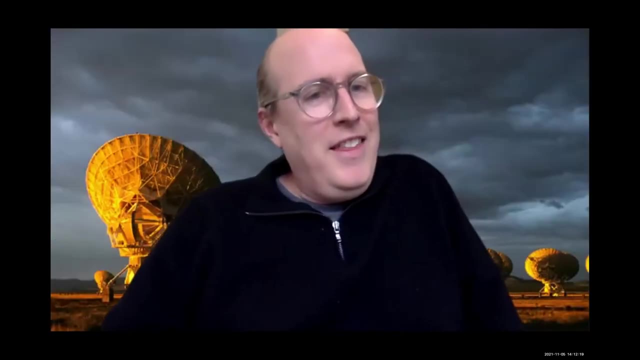 What are the possibilities of extracting helium-3 and really using that as the source for a fusion rocket, maybe even the launch pad for fusion devices? Yeah, unfortunately. I think you probably know more about that than I do. I don't have much to add there. 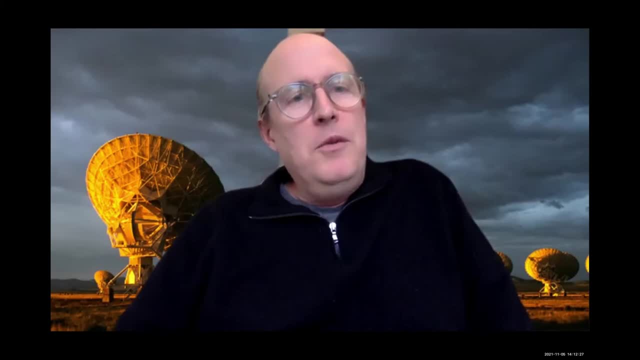 But you know, I was just curious to follow up with Jake. So the properties of these liquids, I mean, is it that the viscosity is, you know, very strange, Or what are the unusual properties that you end up with? Yeah, viscosity is one of them. Helium-3 will go superfluid, just like helium-4 will at certain temperatures, And that enables a whole neat cadre of devices. I mean liquid hydrogen. it won't go superfluid, but it still has the lowest viscosity of any of the regular fluids. 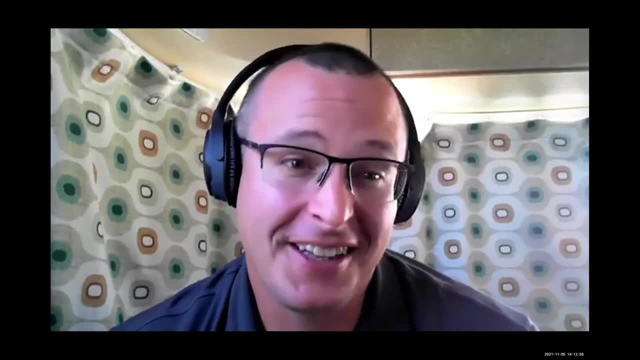 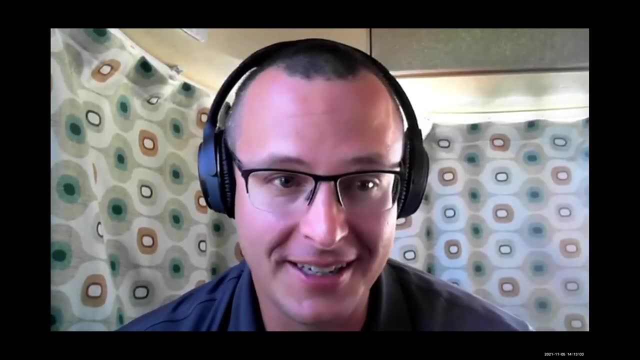 which presents its own challenges and opportunities. You just have to think differently when working with some of these fluids. So yeah, if you're mining the moon for helium-3, I'm all about designing a helium-3 liquefier and storage tank. 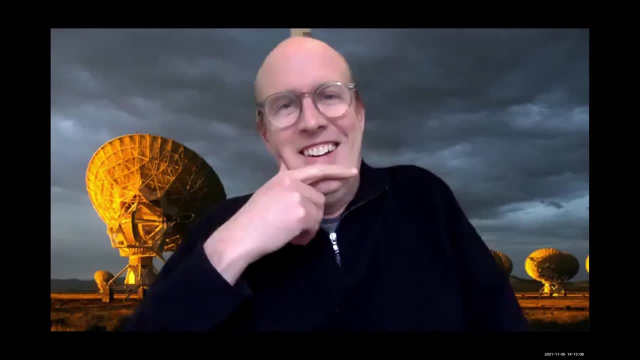 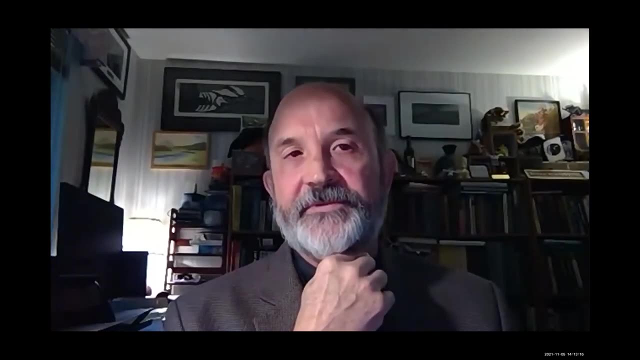 I'll help you out with that. I mean I would, that's great. Sorry, I wanted to add one thing to that, because the studies that I've seen of fusion systems for Mars missions indicate that we don't that there's actually plenty of helium. 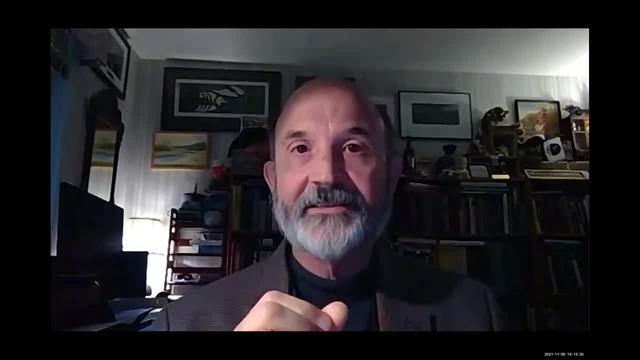 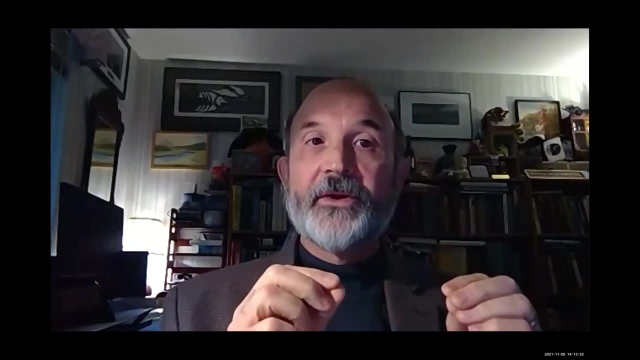 Helium-3 is produced today on the Earth in small quantities. The beauty of a fusion system is you don't need very much to do a pretty amazing mission. So in fact, if you look at the production rates of terrestrial helium-3,, 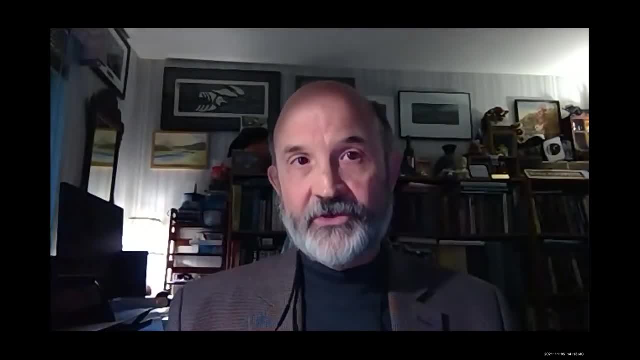 that is enough to do many Mars missions, crude Mars, big Mars missions, right? So yes, Yuri, I totally agree with you that it'd be wonderful to mine helium-3 on the moon, And I hope Josh is successful and manages to. 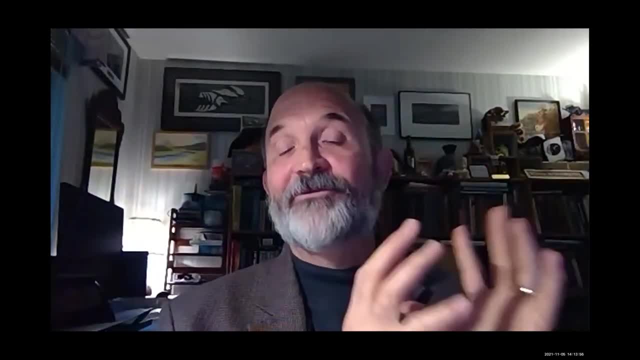 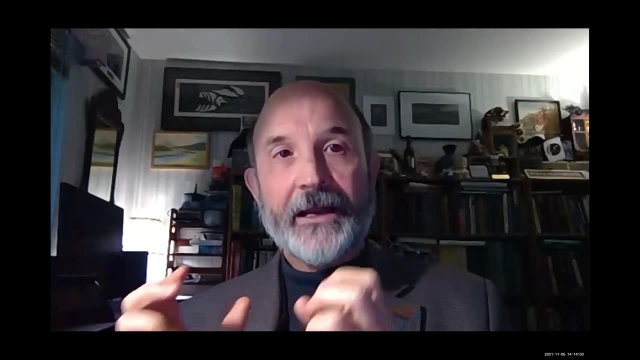 to have that, but we don't have to do it for the first several missions. right, We can. we can proceed. if we are successful in developing the technology, figuring out how to how to build fusion propulsion systems, we can do the Mars missions. 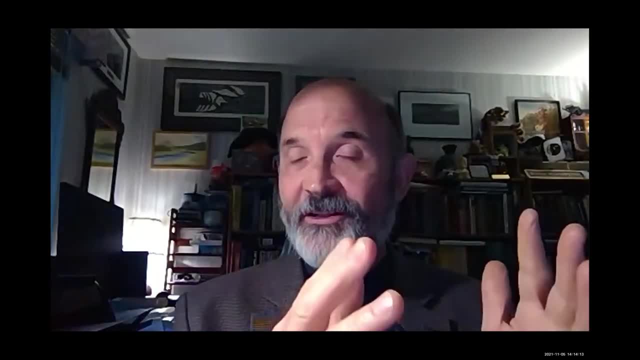 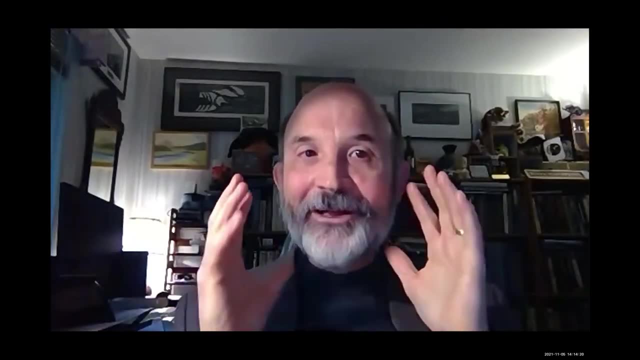 And luckily they're fast enough so that we don't have to invoke all of Jake's fancy long-term storage, because you only have to store it for much shorter periods of time. You will need some, Absolutely Yes, Jake, we need you. 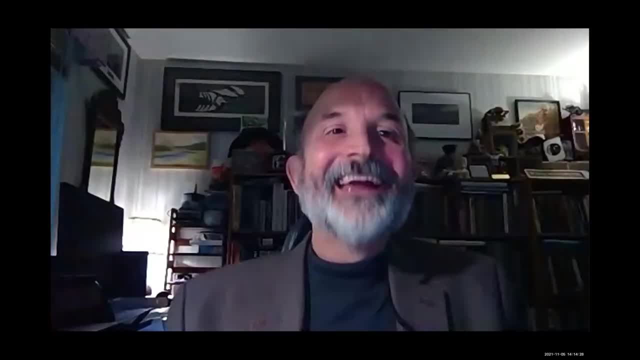 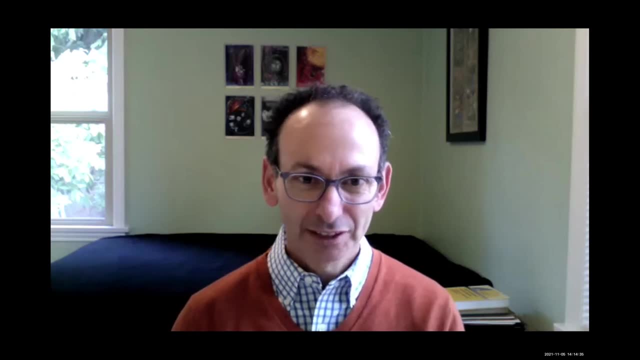 We'll see who solves their problems first. How about that Exactly? Yes, I agree, Good, good, good point. This is a great discussion. I think we've got a couple of minutes. Maybe we can take some questions from the audience. 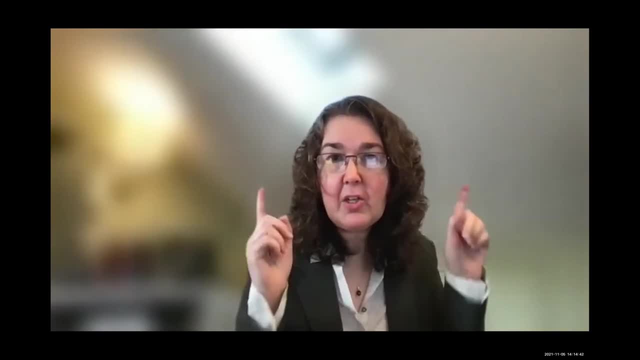 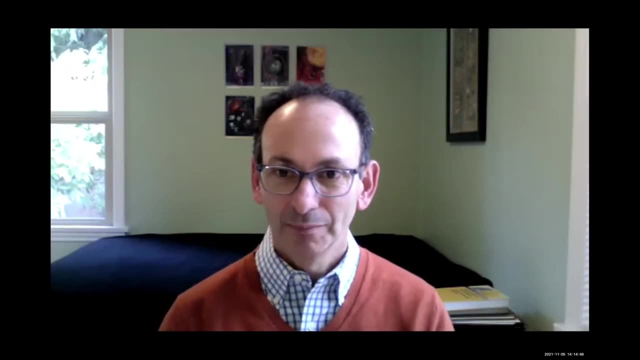 We can do a couple of minutes, but then if you, if the panelists can answer things on Whova, that would be awesome too. Yes, Thank you, Christie. So, Amy, do you have? can you have a read a question from the audience. 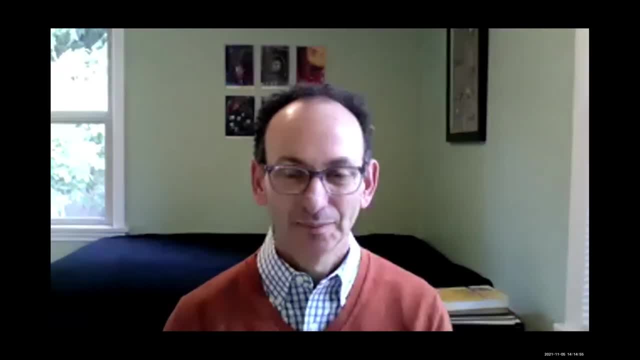 please, I can. Let's see, Anna. can you connect? She signed in again, but I can certainly take it. Oh, are you ready, Anna? You're good, Yuri, you've been answering, asking most of these questions actually in a. 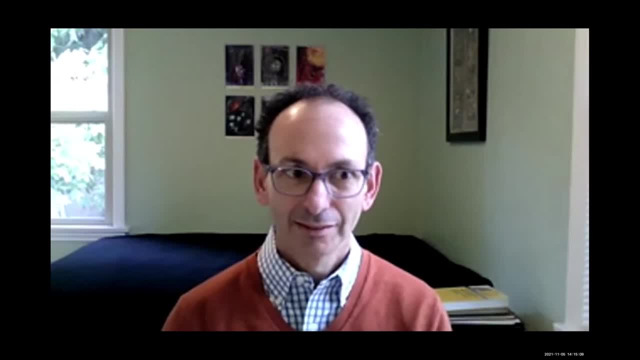 in a relatively reasonable format, just with your interest. but I guess the top rated question is what policy or political changes should be made to advance the research, commercial work and scaling of highly experimental nuclear power systems. I mean, we've kind of been discussing that. 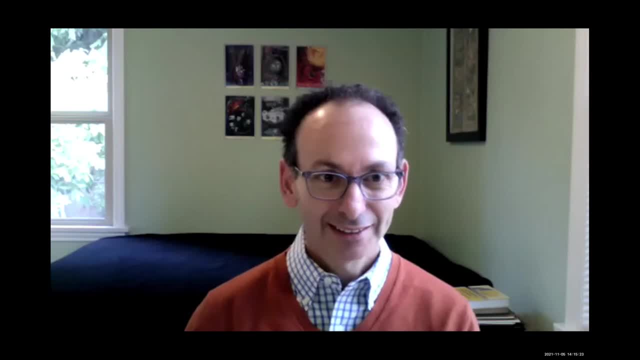 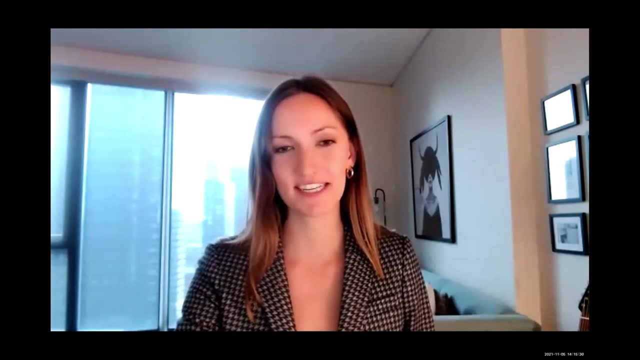 but if anyone has any other thoughts. No, Jess, would you like to take that one? Sure, Sure, Thanks for the question. Yeah, So there are a couple of policy and legal changes that are definitely already being discussed in the international community. 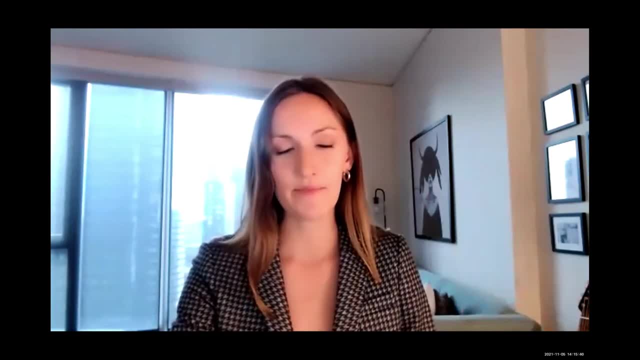 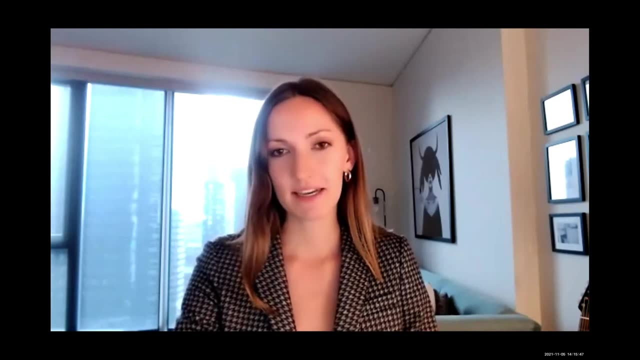 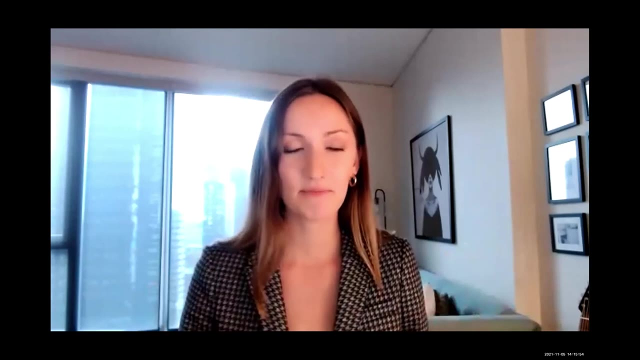 And so, with regard to safety, the, like I said, the the principles from the UN general assembly resolution. they're not binding, And so this really hinges on um national implementation, on this becoming national law and these principles being spelled out more. 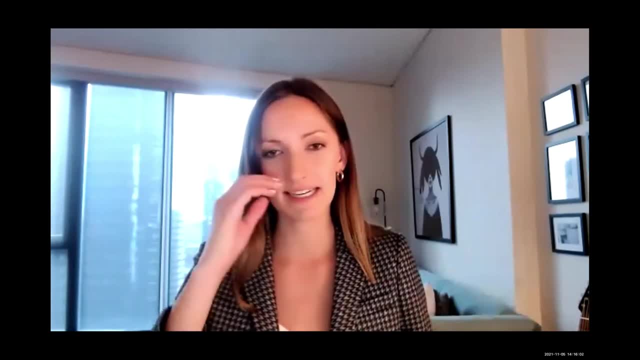 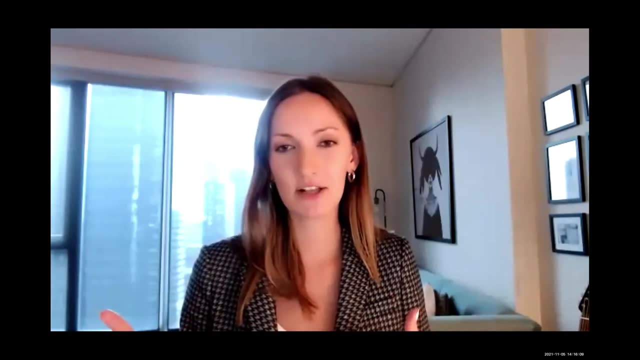 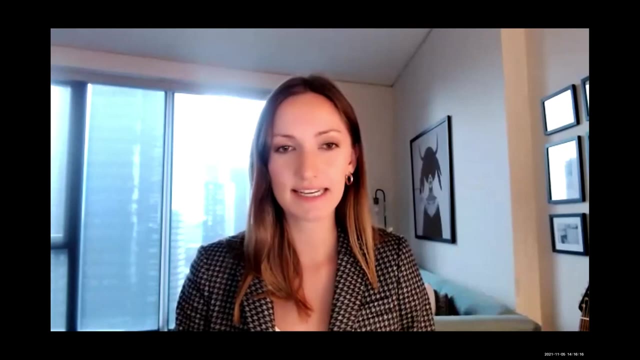 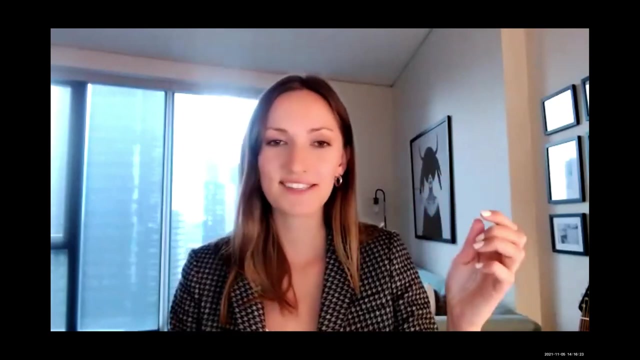 So they're very broad. They do recognize that nuclear power sources in outer space should be based on a thorough safety assessment, including, you know, risk analysis and all these considerations like accidental exposures, And so the I think the real crux is how to 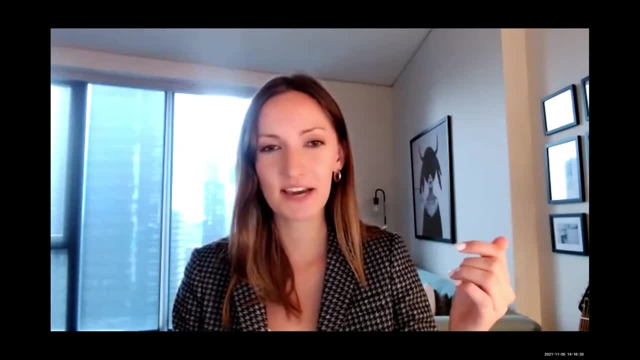 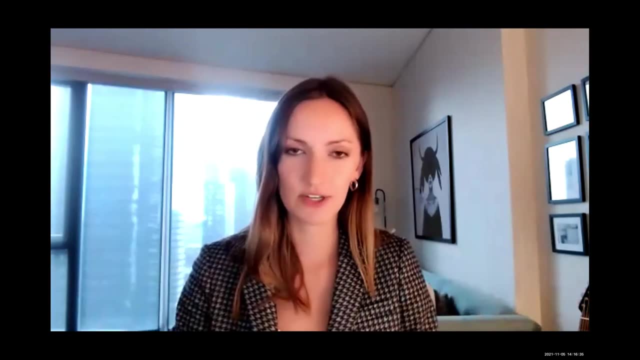 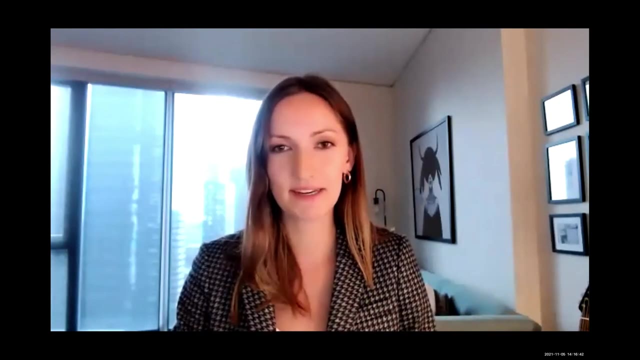 how to formalize these risk assessments, how to formalize these risk analyses um and determine more in licensing conditions and regulations- what, what risks we're we're willing to accept. So so that's definitely a big challenge um. 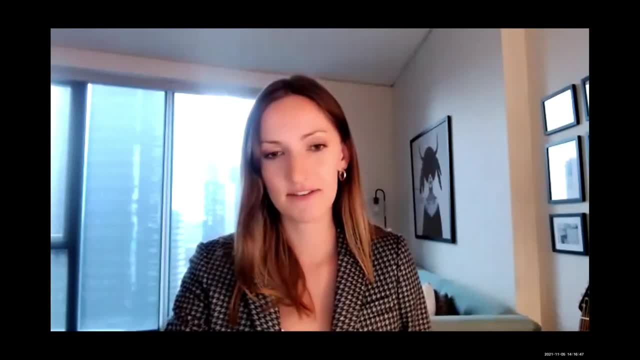 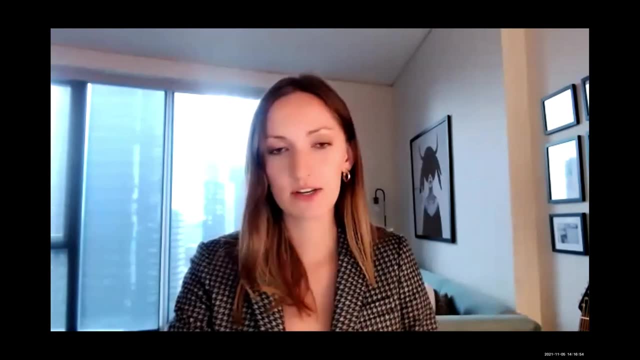 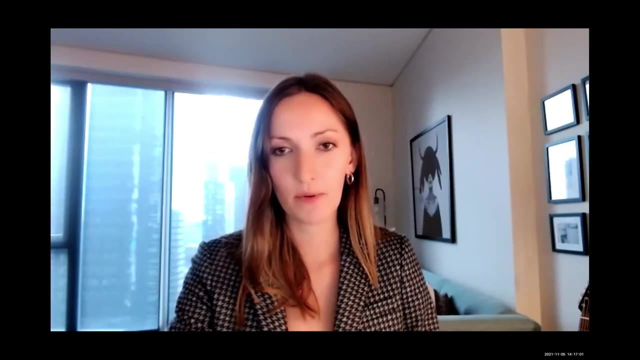 for any regulatory agency in the US and outside of the US. Um and then um looking at um more general international law, I think there's definitely the the IAEA safeguards. um question of how do we? I think I already touched on this. 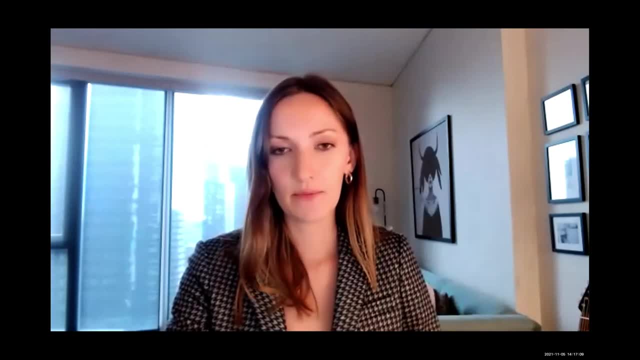 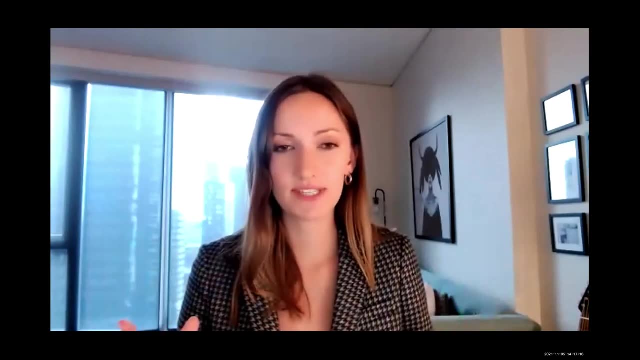 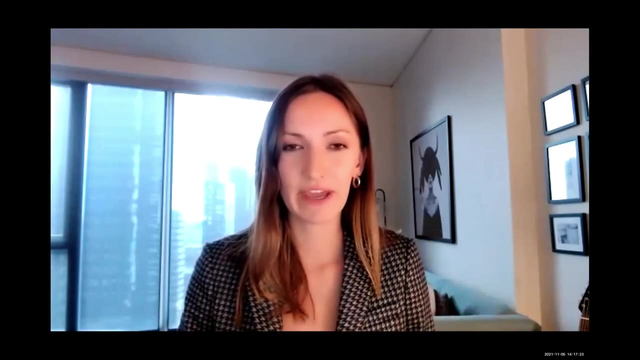 How do we um make sure that we account for shipping, testing um and launch um safeguards during those times, which aren't um usually in place for for more traditional uh reactors that we have on the ground? 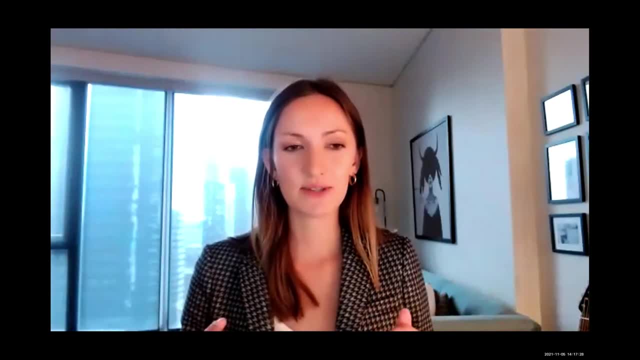 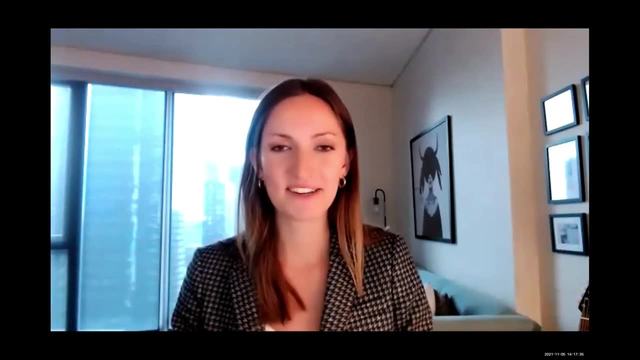 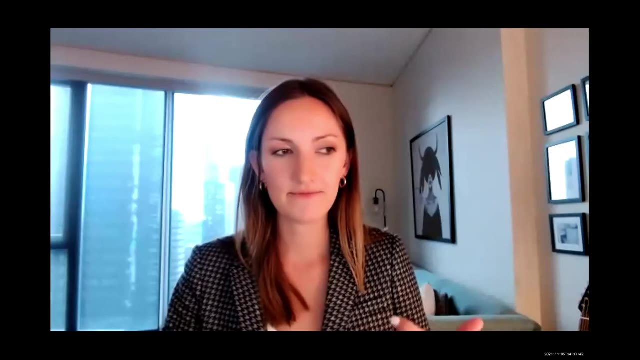 right. So. so there's really these considerations where I think we need to speak. the technical community needs to uh, speak, uh to the policy makers and to to the legal people and really make sure that we understand how we can reach. 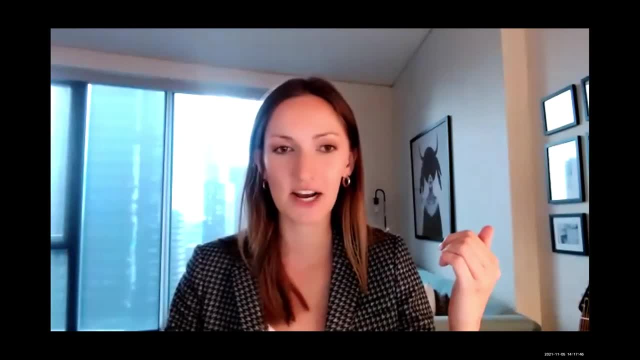 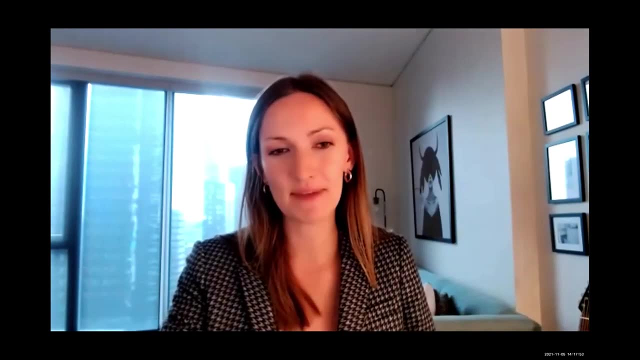 uh solutions that are risk-based and smart and allow the commercial sector to to advance and for us to for us to eventually reach Mars, um while also um making sure we don't accept any um risks that are disproportional. 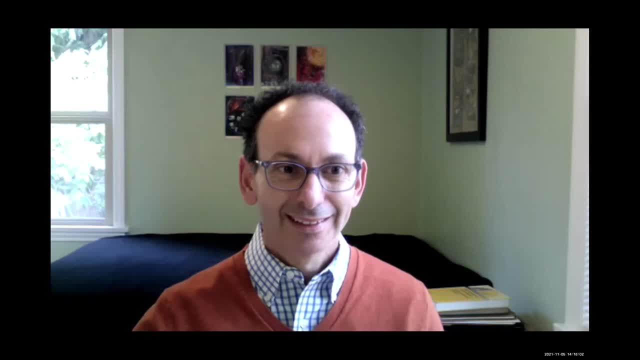 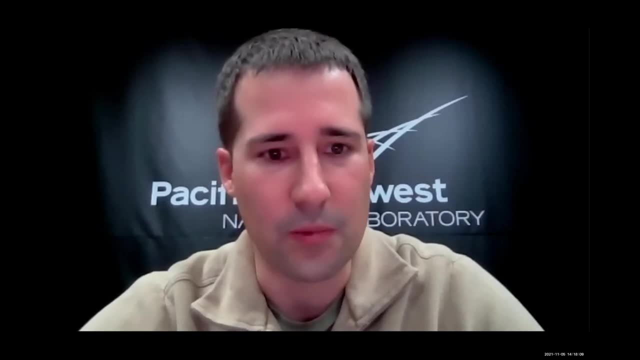 Great. Thank you, Just like- if I can hop on that too, Yuri, uh from from the technology side, I think what is needed, uh, especially to support commercial developments and long-term deployment, is for the government to have a 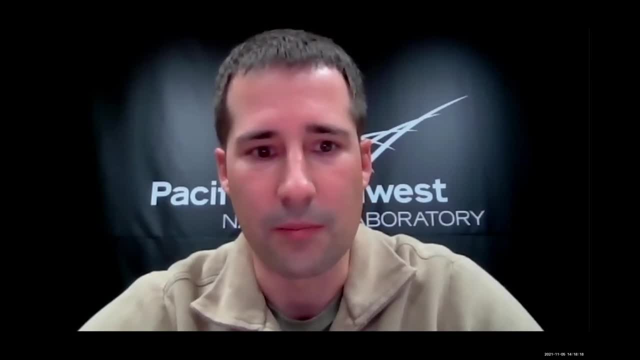 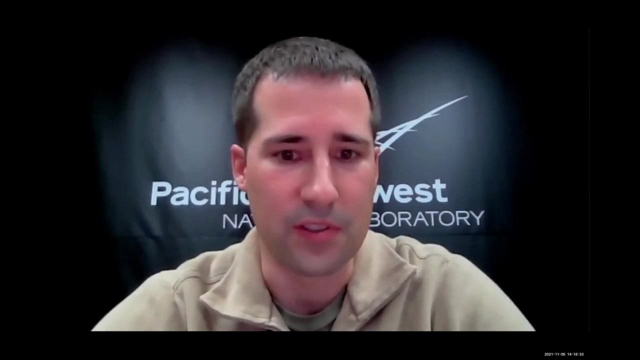 a sustained fundamental R and D program, particularly in materials that are pertinent to space. nuclear power systems- uh- and propulsion systems- Uh. these are technologies and and areas that aren't necessarily developed for other purposes in some cases, And. 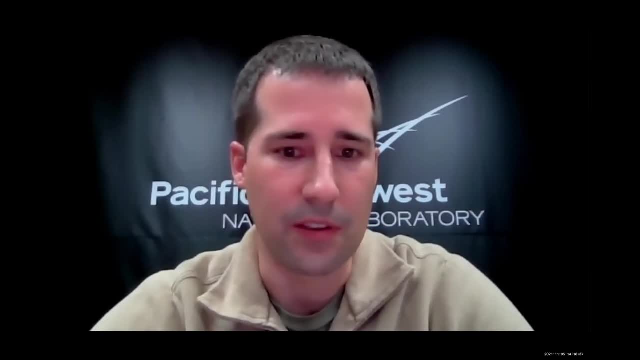 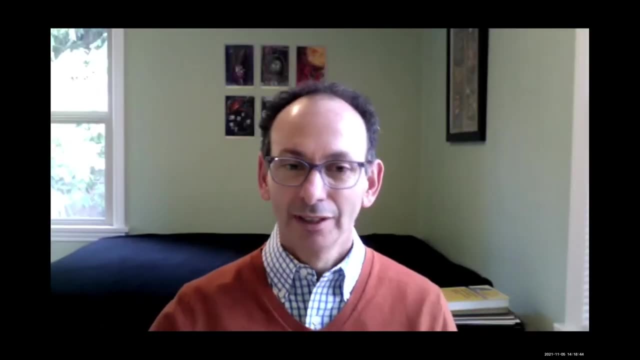 uh, having a sustained program to advance. those is something that I think is going to be important in the long term. Thanks for that addition, Jeff. That's really helpful. Um, so I I think with that we'll wrap up our.